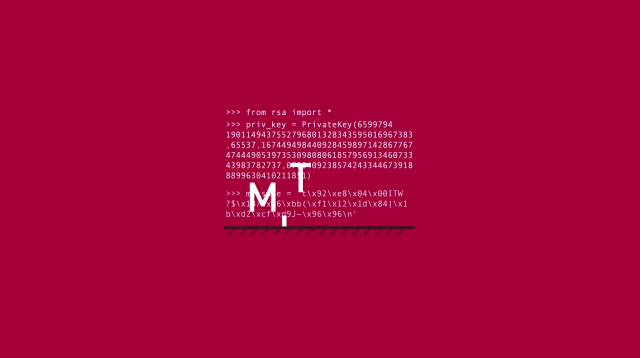 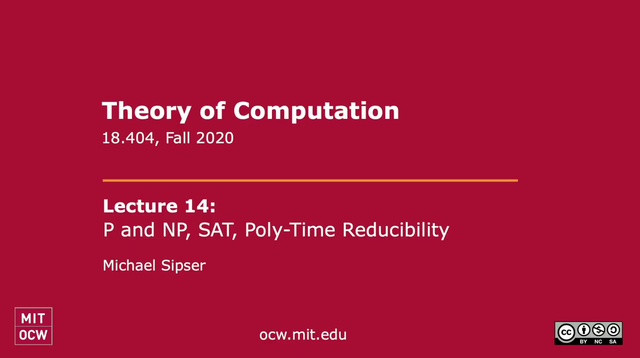 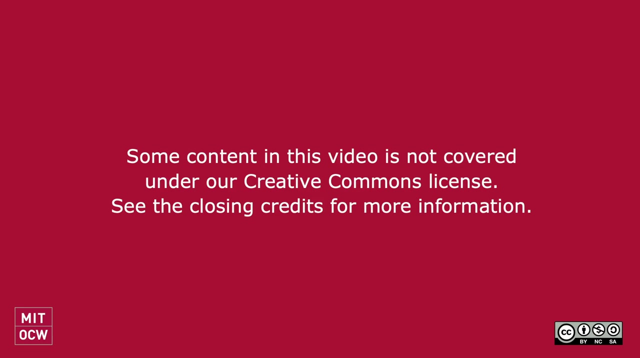 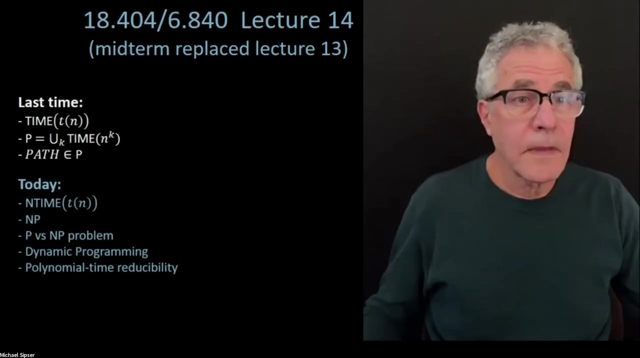 Okay, hi everybody, Let's get started. So it's been a while since we came together in a lecture. Last week we had the holiday, we had the midterm, So with that, what have we been doing? We finished the first half. 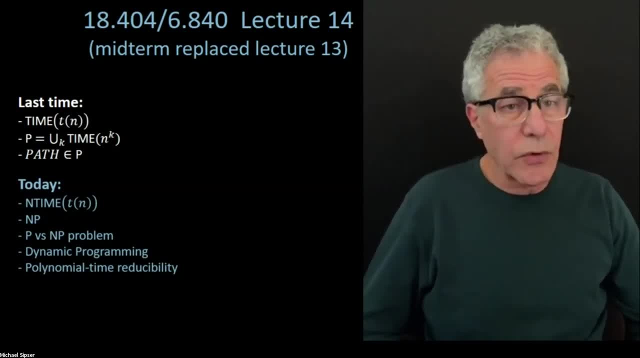 of the course you know about two weeks ago, where we were talking about computability theory, We have shifted into the second half, talking about complexity theory. We have shifted back to that. We discussed the various different models and ways of measuring complexity on. 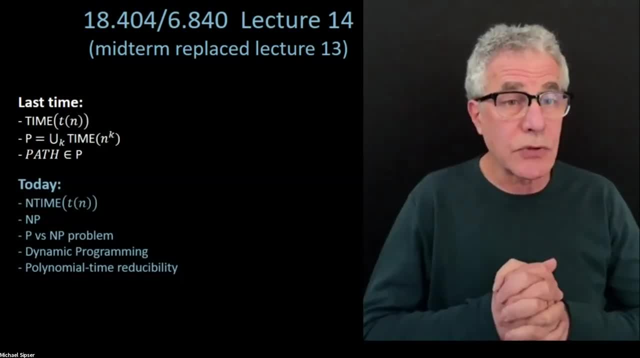 different models, at least in terms of the amount of time that's used, And in the end we settled on the one-tape Turing machine, which is the same model we had been working with in the first half of the course, and argued that, though they're, they're not. 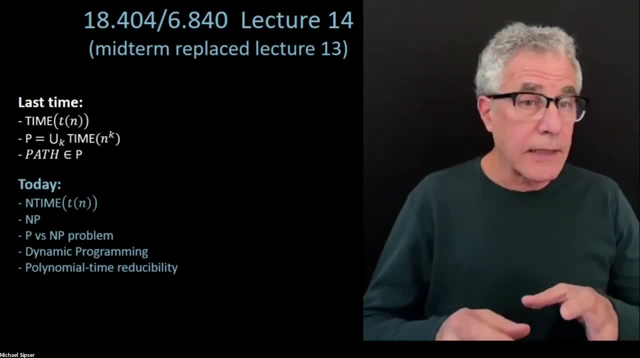 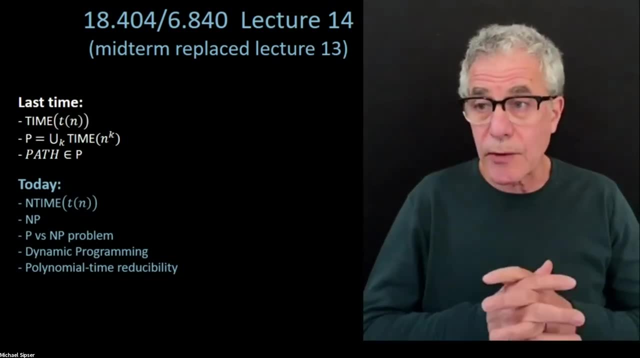 the measures of complexity are going to differ somewhat from model to model. they're not going to matter, differ by more than a polynomial amount. And so, since the kinds of questions we're going to be asking are going to be, basically, whether problems are polynomial or not, it's 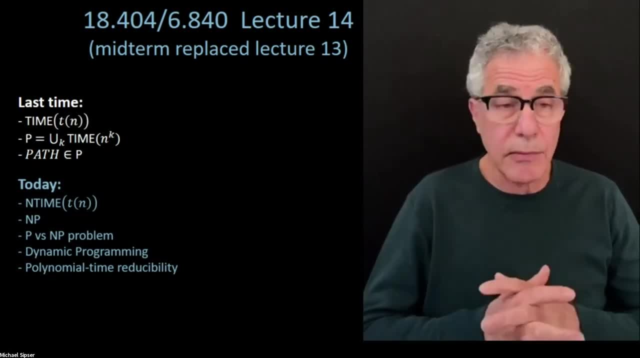 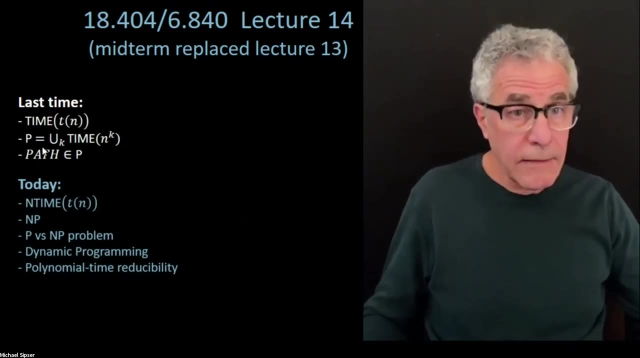 not going to really matter which model we pick among reasonable deterministic models, And so we're going to. the one-tape Turing machine is a reasonable choice, Given that we defined time complexity. We defined time complexity classes, the time T of n classes. We defined the class P, which 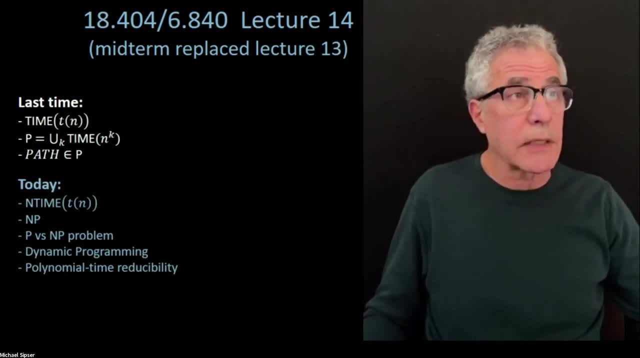 was invariant among all of those different model, deterministic models, in the sense that it didn't matter which model we choose. We were going to end up with the same class, P. so that argues for its naturalness. And we gave an example of this path, problem being: 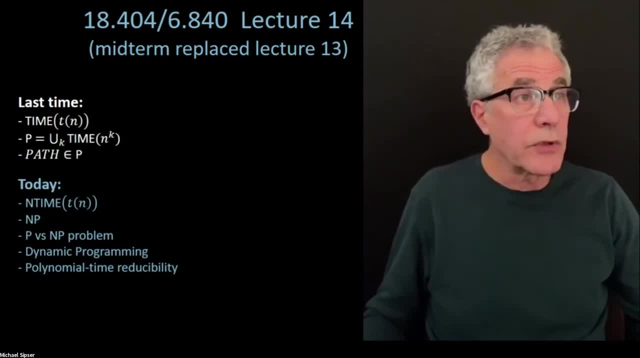 in P and we kind of ended that lecture before the midterm with the discussion of this Hamiltonian path problem. so we're going to come back to that today. So today we're going to look at non-deterministic complexity: define the classes- non-deterministic. 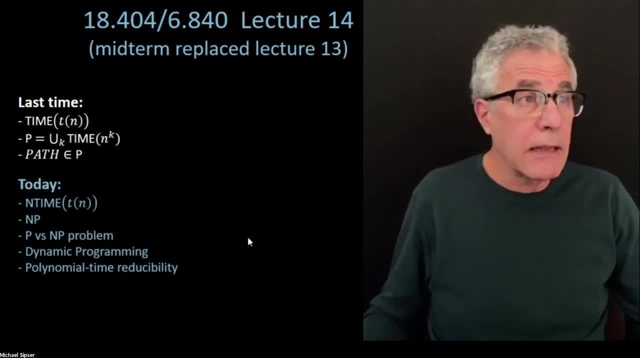 time or n time. talk about the class NP, the P versus NP problem, which is one of the very famous unsolved problems in our field, and look at dynamic programming, one of the most basic algorithm, polynomial time algorithms and polynomial time reducibility. moving toward 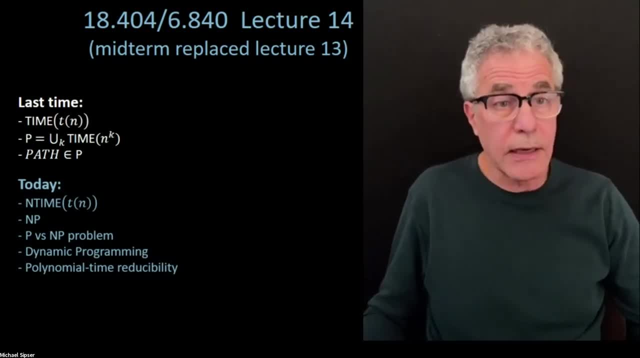 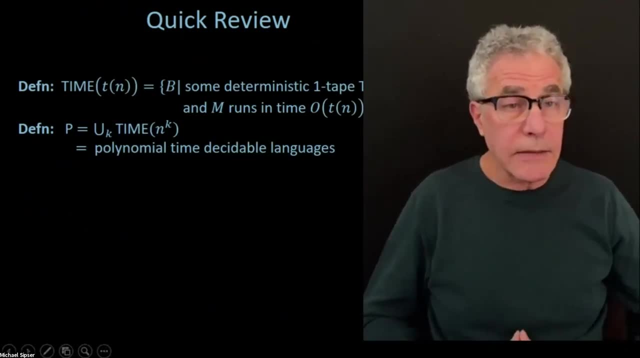 our discussion of NP completeness, which we will begin next lecture. So with that, let's move into today's content, which is, well, just a quick review. We, as I mentioned, we defined the time complexity class. This is a: the time complexity. 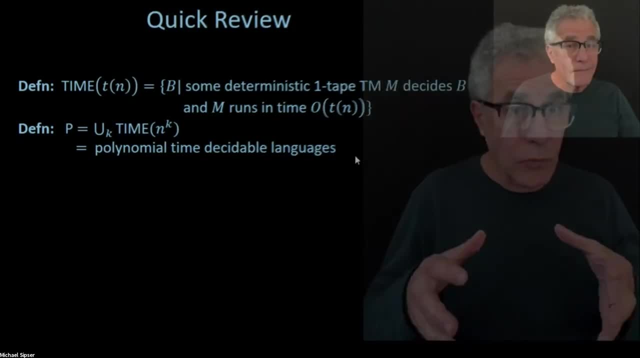 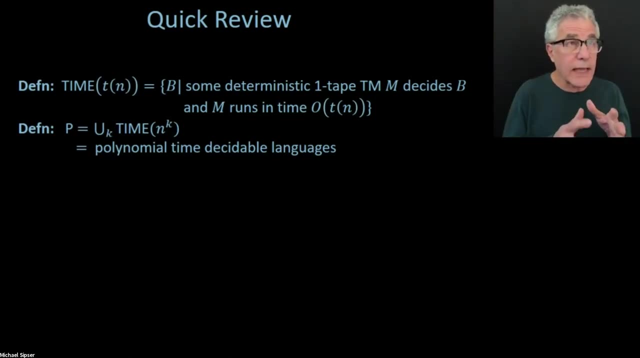 class is a collection of languages, The languages that you can do. these are a collection of languages, All of the languages that you can solve in a certain amount of a certain time, down within a certain amount of time. So the time, the time n squared, for example. 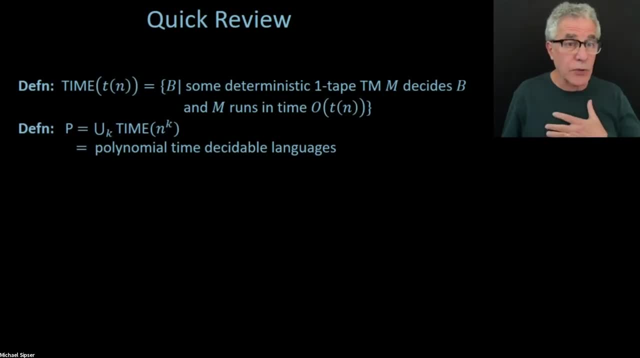 is all of the all of the languages, or all of the problems that you can solve in n squared times. We're identifying problems with languages here, And the class P is the collection of all problems that you can solve, or all languages that you can solve, in polynomial time. So 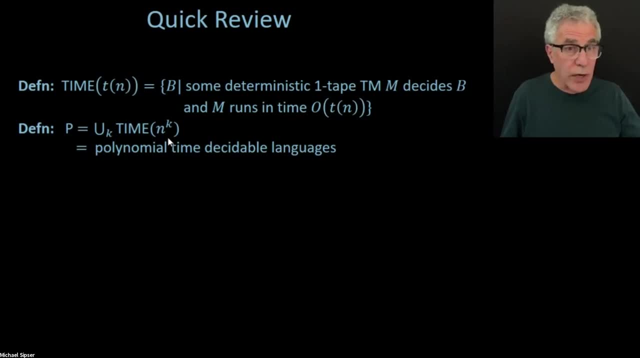 it's the union over all time into the k, So n squared n, cubed n to the fifth power and so on. We're identifying union out of all that, All of those bounds, the associated language, languages. that's the class P, And we gave an example of this path problem. We gave an 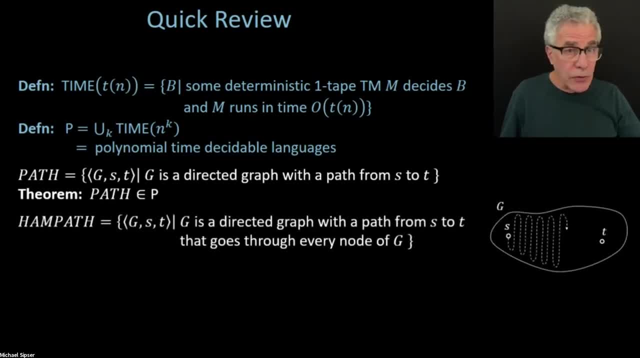 algorithm for path, And then we introduced this Hamiltonian path problem. So, if you remember, instead of just asking, given a graph, whether you can get from s to t, Now we want to know. Okay, s to t, but visit every other node along the way. 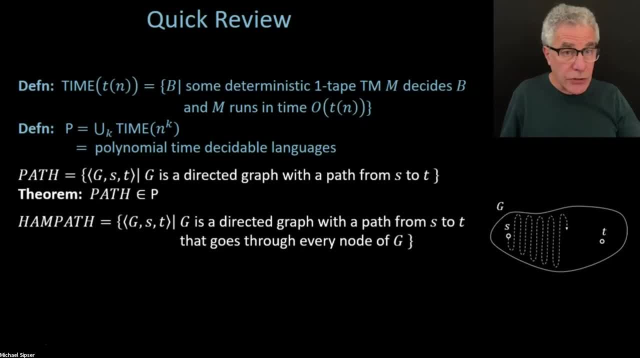 So find a path that goes through everything else and gets from s to t, And I should say it's also a simple path, So you're only allowed to go through every node just once. And now the question is for this problem. 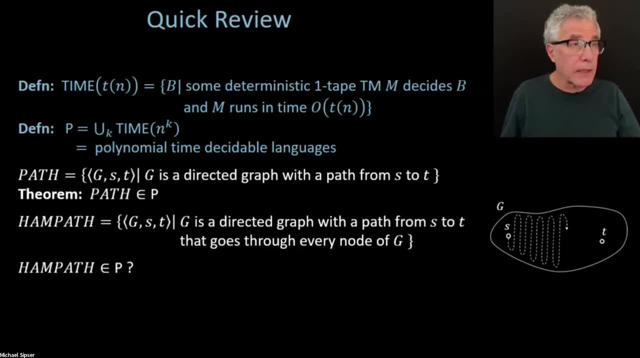 is that: can we solve that problem in polynomial time? Can we somehow modify the algorithm for path to give us an algorithm that solves Hamiltonian path in polynomial time? Of course we could solve Hamiltonian path with an exponential algorithm by trying all possible paths. 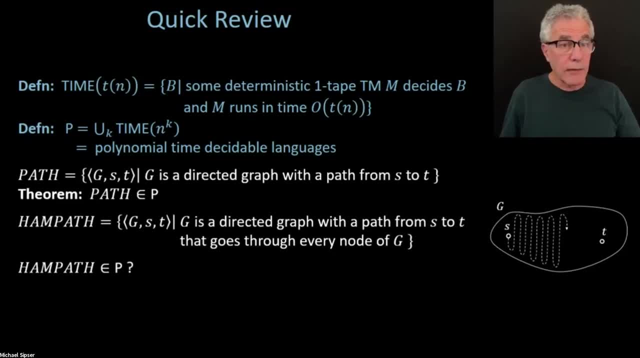 And that will give a correct algorithm. But there are exponentially many different paths And trying them all will not give a polynomial time algorithm. So the interesting problem is that we can solve that problem without doing that brute force searching through all possible paths. And that's a problem that no one knows the answer to. 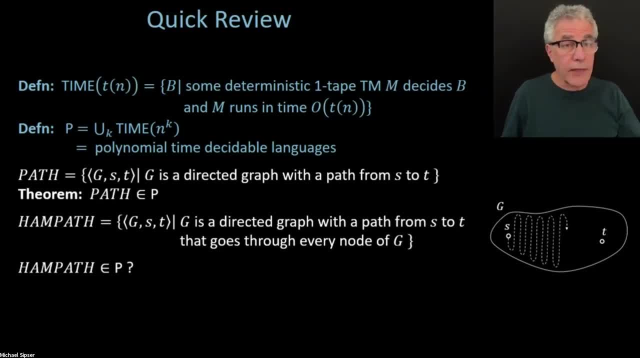 Despite lots of effort, people have not succeeded in finding an algorithm for that, But on the other hand, we don't have any idea how to prove there is no such algorithm. I mean, it's conceivable that one could prove such a thing? 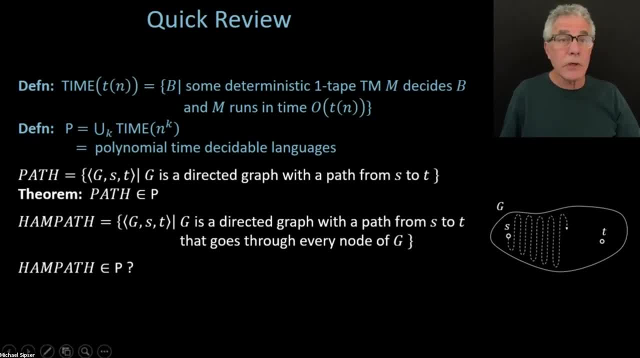 but we just don't know how to do it, And so So that problem is an unsolved problem, And I just want- this isn't really a note to myself- What's kind of amazing. and this is what we're going to be showing over the next few lectures. 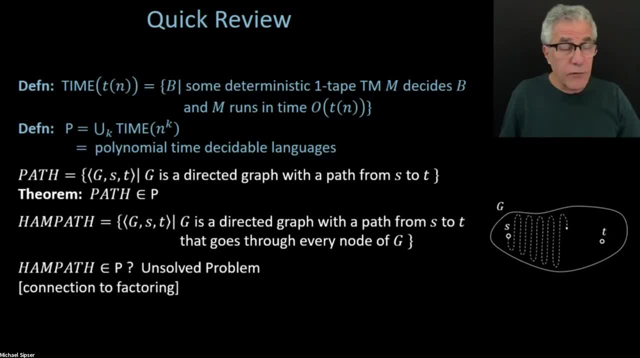 that there would be very surprising consequences if you could find a way to solve Hamiltonian path in polynomial time, Because what that would immediately yield is the polynomial time way of say, factoring large numbers or solving, And a large number of other problems. 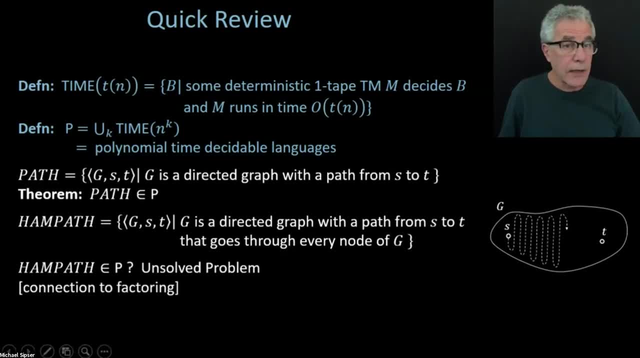 that we don't know how to solve in polynomial time. So, as we mentioned, factoring is a problem that we only know at present how to solve with an exponential algorithm, And it doesn't seem to have anything to do with the Hamiltonian path problem. 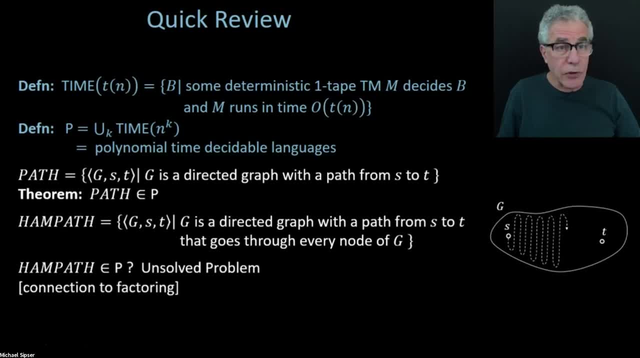 It seems very different, But yet, if you can solve Hamiltonian path in polynomial time, then you can factor numbers in polynomial time, And so we'll see how to make that connection. But that's what we're building toward with the next few lectures. 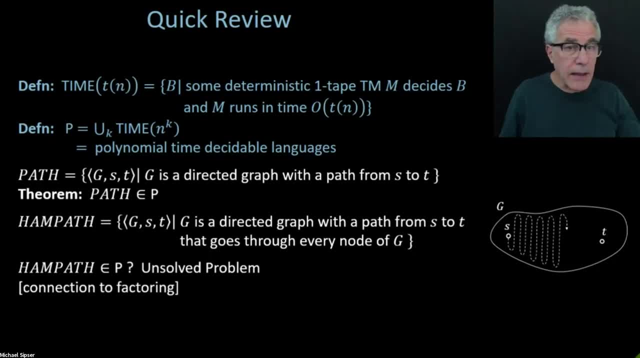 OK, So happy to take any comments and questions on that, Or we'll just move on. if you have any questions on our little review, Well, send questions along, and we can stop at the end of various slides to try to answer them. 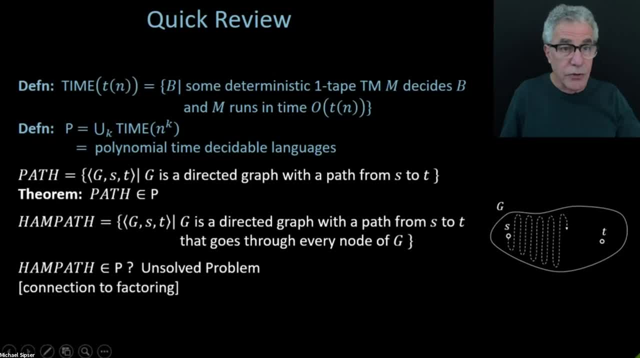 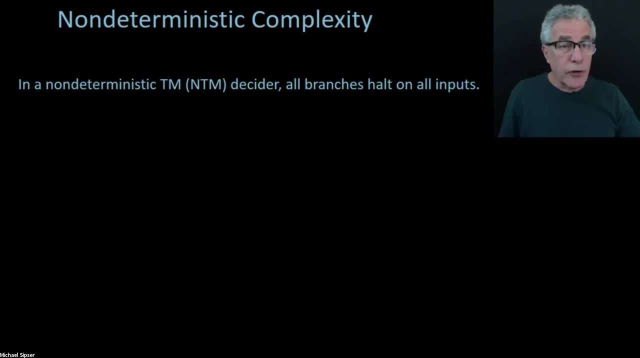 And, of course, write to the TAs, who can take your questions during while I'm lecturing. OK, So to start this off, we're going to have to talk about nondeterministic complexity as a variation of deterministic complexity. So, first of all, when we have all of the machines, 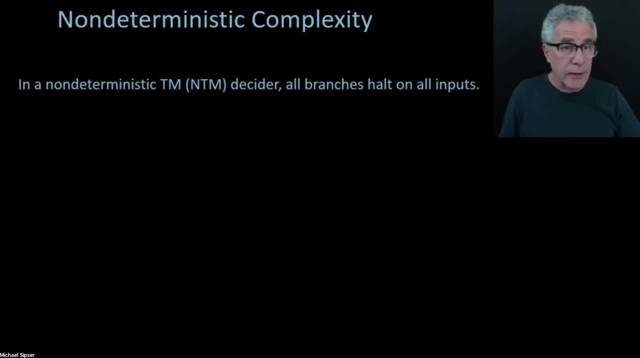 in this part of the course and the languages. everything is going to be decidable and all the machines are going to be deciders. So what do we mean when we have a nondeterministic machine which a decider is a decider? 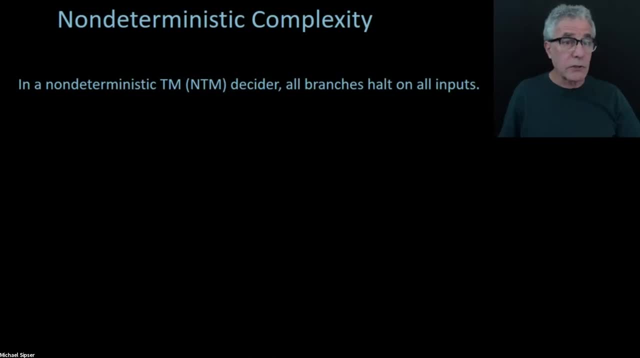 And that just simply means that all of the branches- it's not just the machine- holds on every input, but all of the branches hold on every input. So the nondeterministic machine is nondeterministic. It has lots of possible branches. They all have to hold all of them on every input. 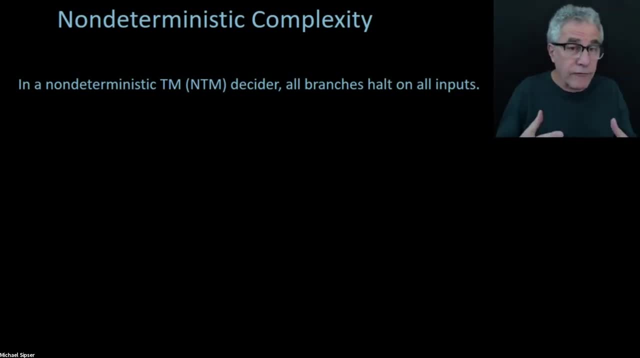 That's what makes a nondeterministic machine a decider. And you're going to convert a nondeterministic decider into a deterministic decider. But the question is: how much time would that introduce? How much extra time is that going to cost? 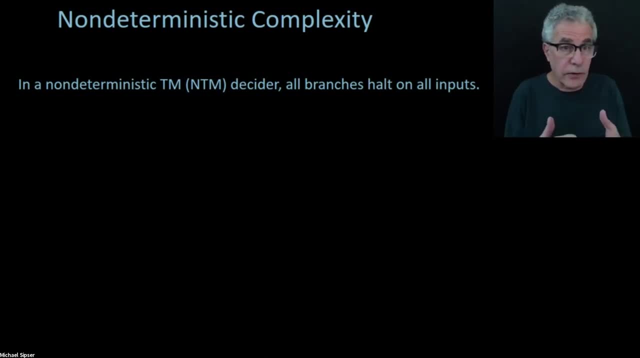 And the only way that people know at the present time for that conversion would be to do an exponential increase, basically to try all possible branches, And that's of course very slow. So first let's understand what we mean by the time used by a nondeterministic machine. 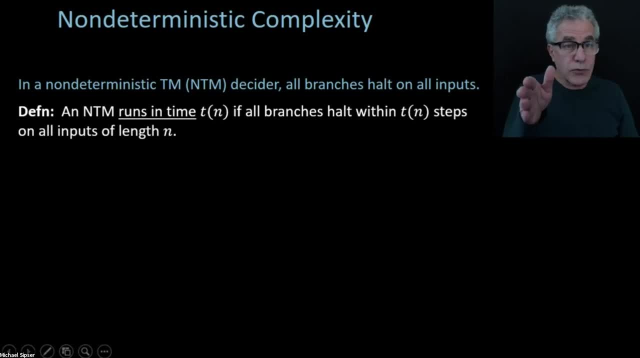 and what we mean by the time. The time used is. we're looking at the each individual branch individually, separately. So a nondeterministic machine, we'll say, runs in a certain amount of time if all of the branches halt within that amount of time. 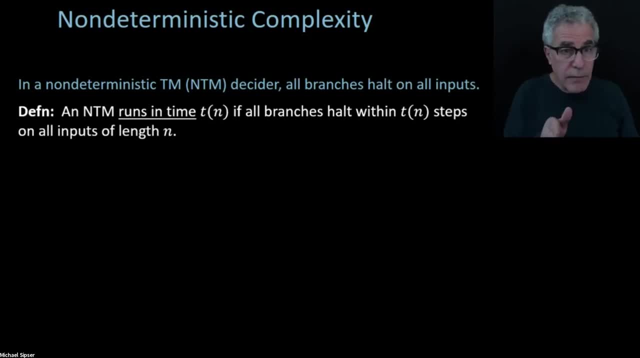 So we do not mean that the total amount of usage, the total amount of effort, by adding up all the branches, is at most t of n. It's just that each branch individually uses at most t of n. That's just going to be our definition. 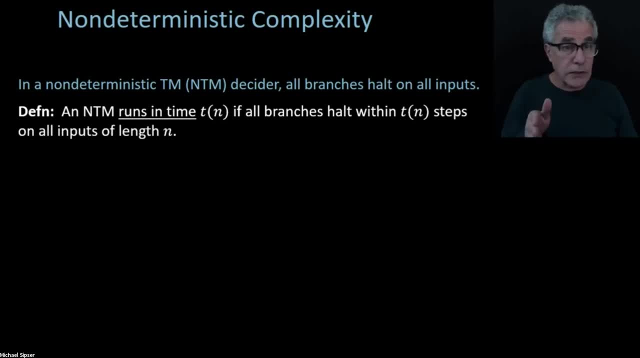 and it's going to turn out to be the right way to look at this to get something useful. So, if we have so, now we're going to define the analogous complexity, the time class associated to nondeterministic computation, which we'll call nondeterministic time. 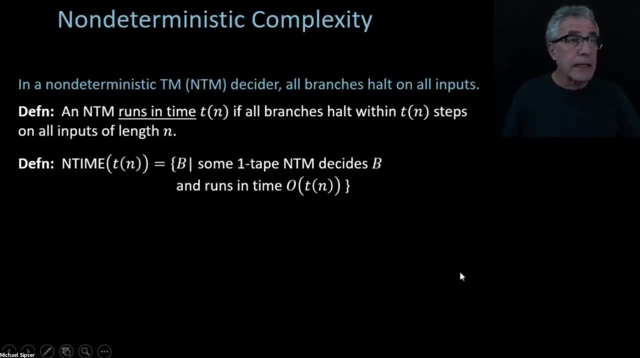 So nondeterministic time, t of n is the set of all languages that you can do with a nondeterministic machine that runs in order t of n time. Just think back to the definition we had for deterministic complexity, the time class. 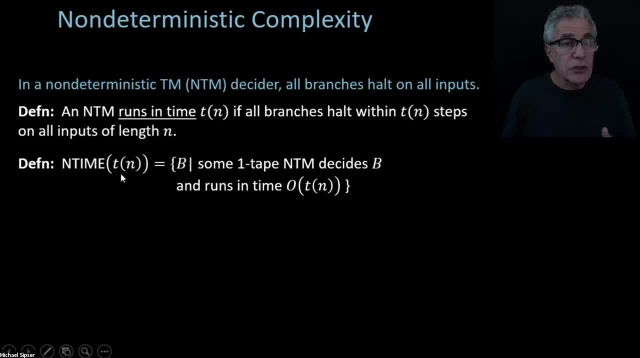 So sometimes people call it d time to emphasize the difference. But let's just say we're calling it in this course time versus n time. So time t of n is all of the languages that you can do with a one-tape Turing machine, that's. 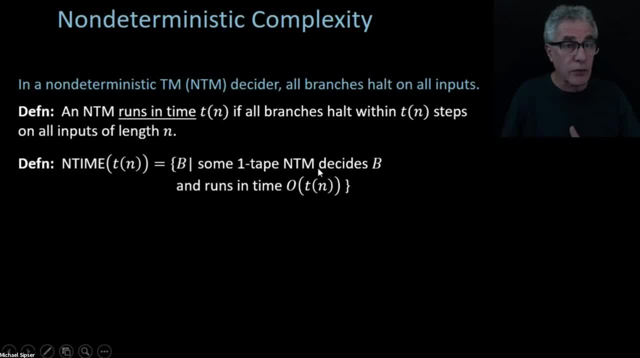 deterministic, But this here is a nondeterministic Turing machine for nondeterministic time. So the picture that is good to have in your head here would be, if you think of nondeterminism in terms of a computation tree, Let's say thinking of all the different branches- 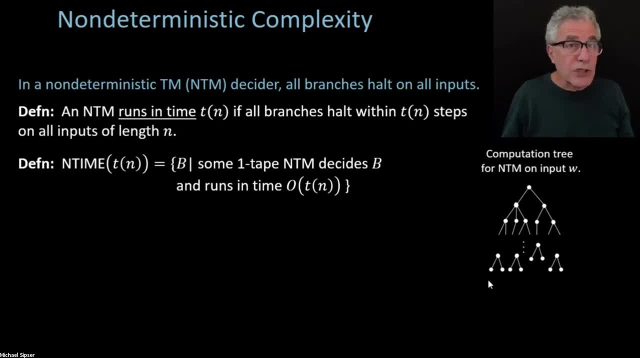 of the nondeterminism. all of those branches have to halt, And they have to halt within the time bound. So imagine here: this is t of n time. All of the branches have to halt within t of n steps for this nondeterministic Turing machine. 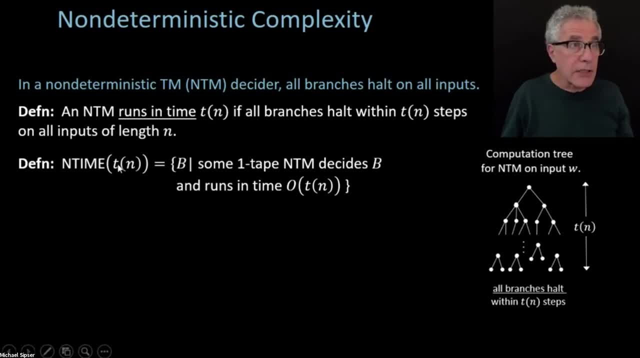 to be running in t of n time and to be doing a language in the n time t of n class And, by analogy with what we did before, the class Np is the collection of all languages that you can do nondeterministically in polynomial time. 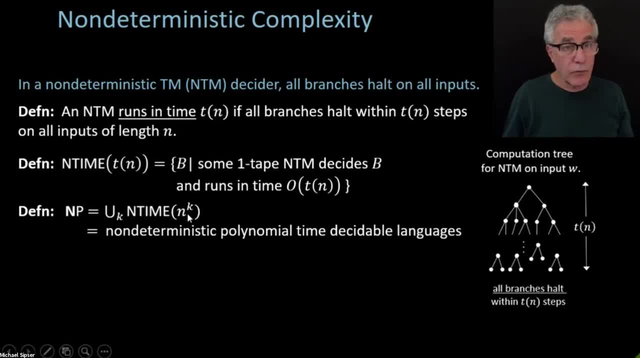 So it's the union over all of the n time classes where the bound is polynomial. So a lot of this should look very familiar, But we've just added, OK, A bunch of nondeterministics and a bunch of n's in place. 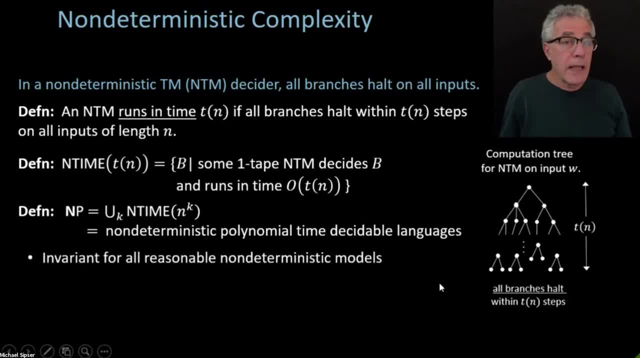 But the definitions are very similar And one of the motivations we had for looking at p, the class p, was that it did not depend on the choice of model, as long as the model was deterministic and reasonable, And this is also the class Np is also. 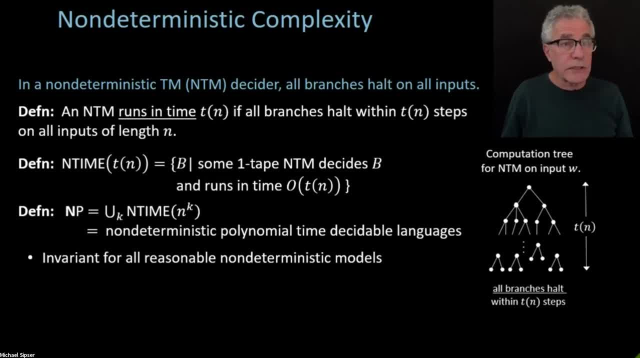 going to not depend on the choice of model, as long as it's a reasonable, nondeterministic model. So it's again a very natural class to look at from a mathematical standpoint And it also captures something interesting from a practical standpoint, which 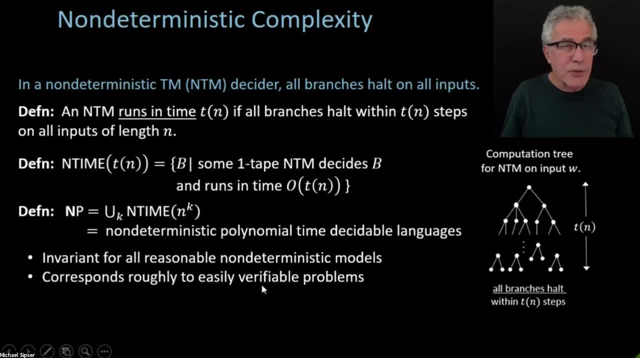 we're going to talk about over the next couple of slides, which is that it captures the problems where you can easily verify when you're a member of the language. OK, so we'll talk about that. but if you take, for example, 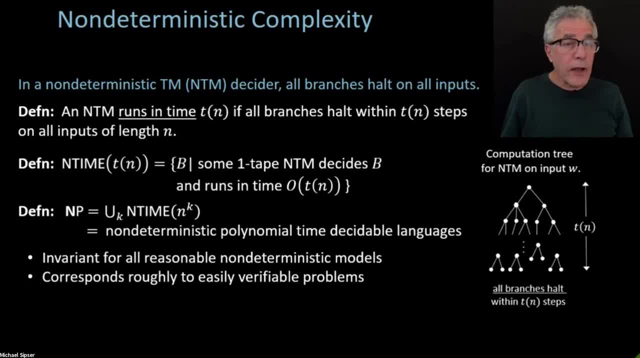 the Hamiltonian path problem when you find a member of the language. so that is a graph that does have a Hamiltonian path from s to t. you can easily verify that's true by simply exhibiting the path. Not all problems can be solved can be verified in that way. 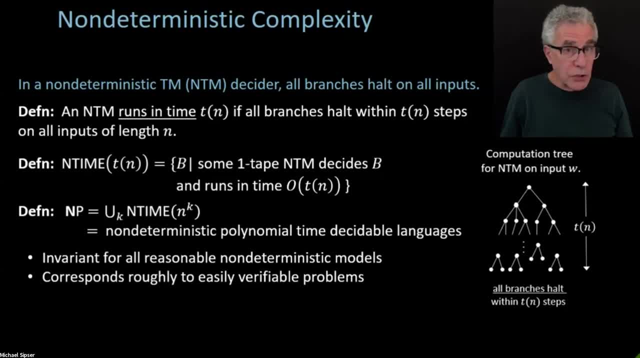 But the problems that are in Np have that special feature that when you have a member of the language, there's a way to verify that you're a member. So we're going to talk about that, because that's really the key to understanding Np, this notion of verification. 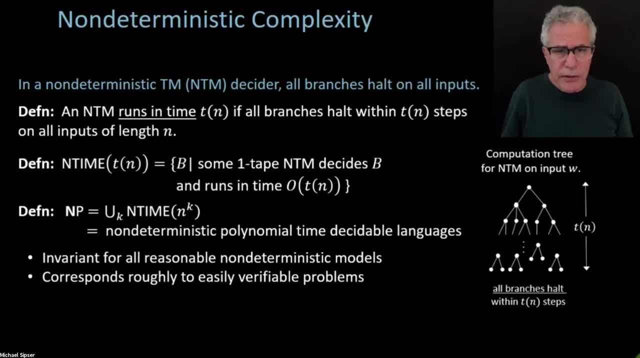 OK, so let me go. There was a good question here. Let me just see if I want to answer that. Yeah, I mean this is a little bit of a longer question that I want to fully respond to, But you mean the well, let's turn to my next slide. 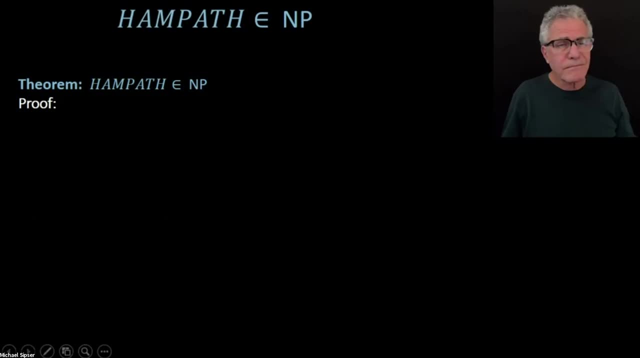 which may be sort of bring that out anyway. Actually, it's a couple of slides from now, But I'll get to that point. So let's look at Hamiltonian, the ham-path problem, And what I'm going to show is the Hamiltonian path problem. 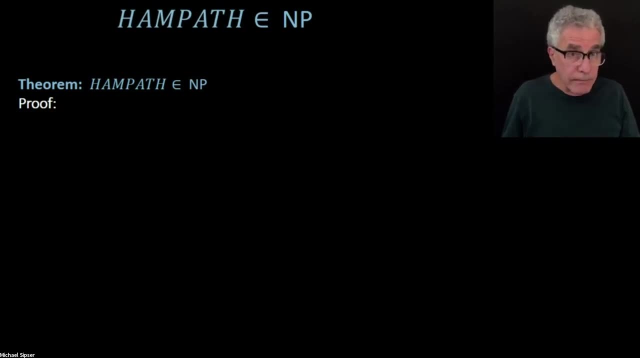 is in Np And I'm going to walk you through this one kind of slowly. So the Hamiltonian path problem, remember, we don't know if it's in P, But it is in Np, So it's in one of these. you can solve Hamiltonian path. 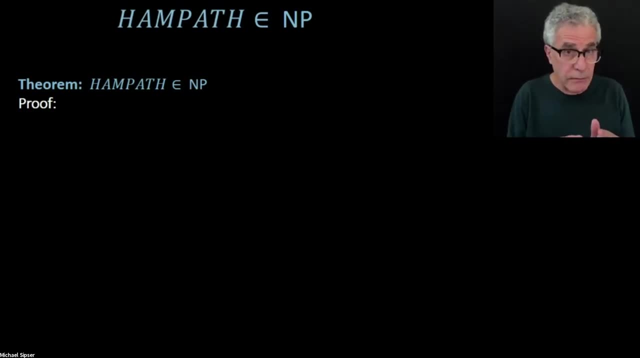 in polynomial time. If you're a nondeterministic machine, why is that? Well, it's because of the nondeterminism, because of the parallelism of nondeterminism, which allows you to kind of check all of the paths on different branches. 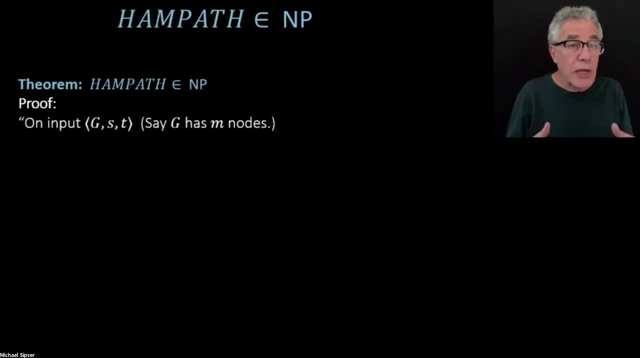 So let me first describe how the algorithm, how I would write down the algorithm, And then we'll kind of try to unpack that and understand how that actually looks in terms of the Turing machine or the Turing machine's computation. So first of all, so taking the Hamiltonian path problem, 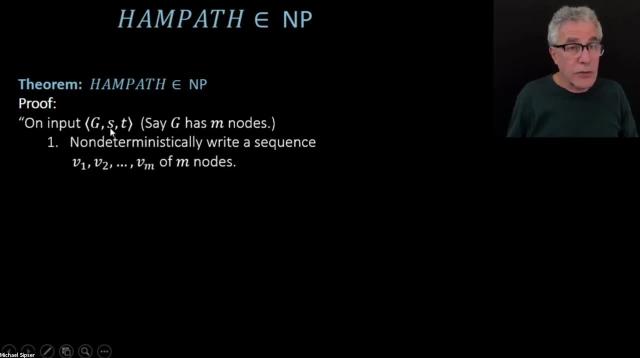 you're given an input now which is a graph and the nodes s and t. where I'm trying to figure out, is there a Hamiltonian path again which visits all the nodes, which takes you from s to t? And we're trying to make now a nondeterministic machine which 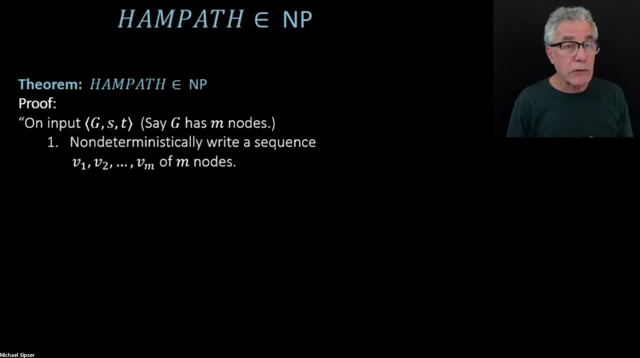 is going to accept all such inputs which have a path. So the way this nondeterministic machine is going to work is it's basically going to use its nondeterminism to try all possible paths on the different branches And the way I'll specify, that is to say nondeterministically. 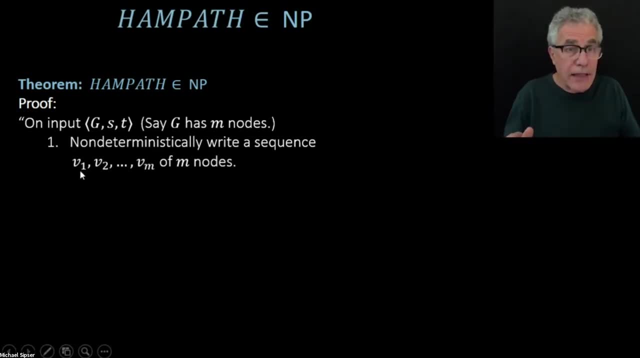 we're going to write down a candidate path Right, Right, Right, Which is just going to be a sequence of nodes, sequence of m nodes, where we'll say that's the total number of nodes of the graph. Remember a Hamiltonian path, because it visits every node. 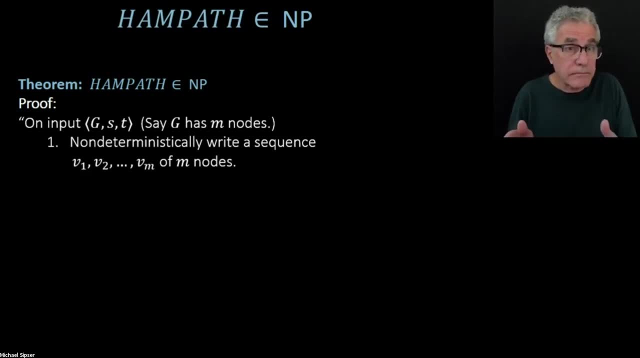 is going to be a path with exactly m nodes in it. So I'm going to write down a sequence of nodes as a candidate path And I'm nondeterministically going to choose every possible sequence in this way, If you like to think of the guessing metaphor. 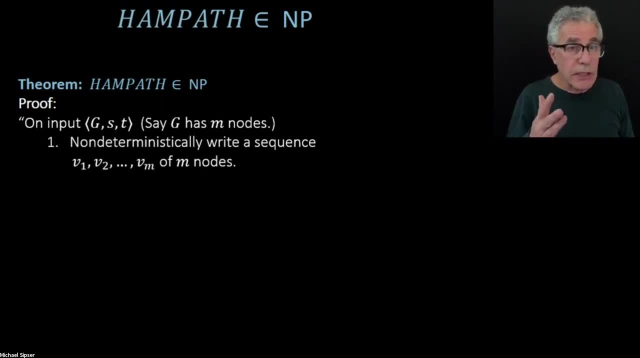 for nondeterminism. you can think of the nondeterministic machine as guessing the right path, which is going to be the Hamiltonian path from s to t. But I think for this discussion it might be more helpful to think about all of the different branches of the nondeterminism. 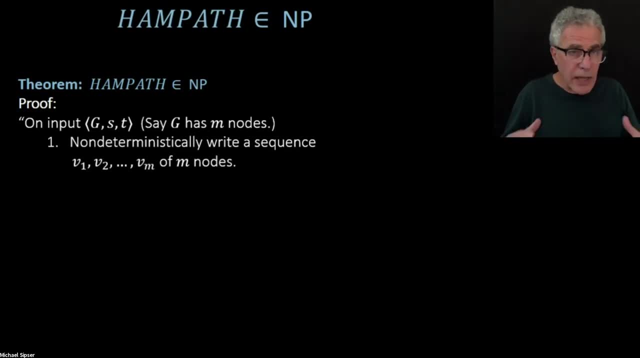 because that's perhaps more useful when we're thinking about it in terms of the time. I think you'll get used to thinking about it in many of the different ways, But maybe the computation tree of all branches might be the more helpful one here. 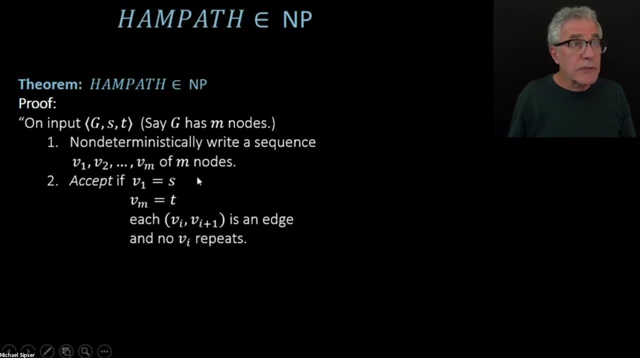 So now, after we write down a candidate path, sequence of nodes, now I have to check that this really is a path. And the way I'm going to do that is to say, well, now, if I have just a sequence of nodes written, 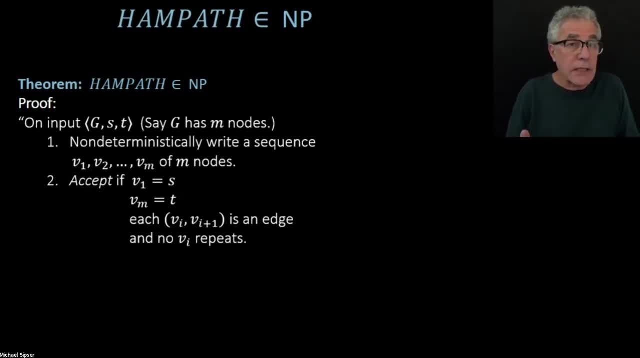 down. what does it mean for it to be a Hamiltonian path from s to t? Well, it better start with s and end with t first of all, And we have to make sure that every step of the way is actually an edge. 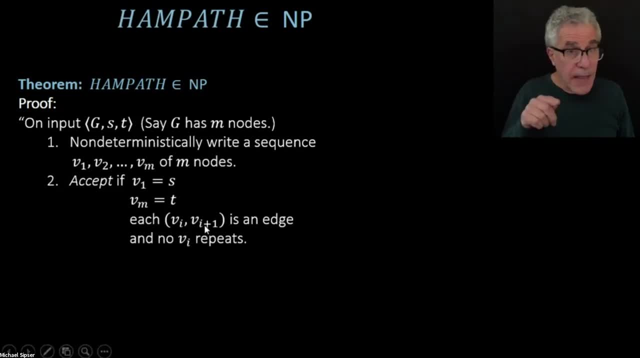 So each pair- vi to vi plus 1, has to be an edge in the graph, Otherwise that sequence of nodes is not going to be a legitimate Hamiltonian path from s to t- And it has to be a simple path. You can't be repeating nodes. 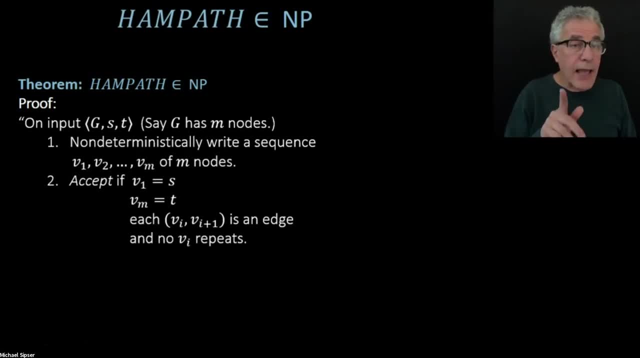 These four conditions together will guarantee that we have a Hamiltonian path. And once we have written down a candidate sequence, we can just check that that sequence actually works. There's no. at this second stage of the algorithm, nondeterminism is necessary. 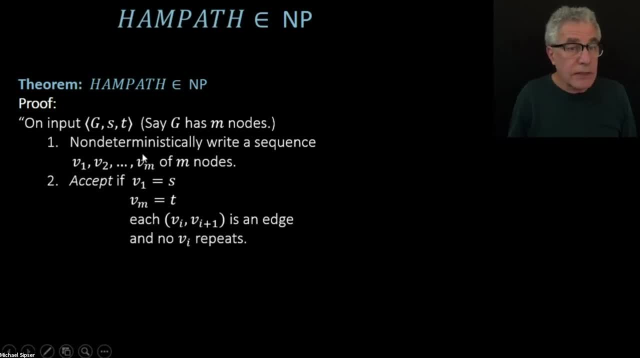 This is going to be a deterministic phase, But the stage one of the algorithm is going to be a nondeterministic phase where it's writing down all possible paths. Now I'm going to try to unpack that for you so you can actually visualize how the machine is doing this. 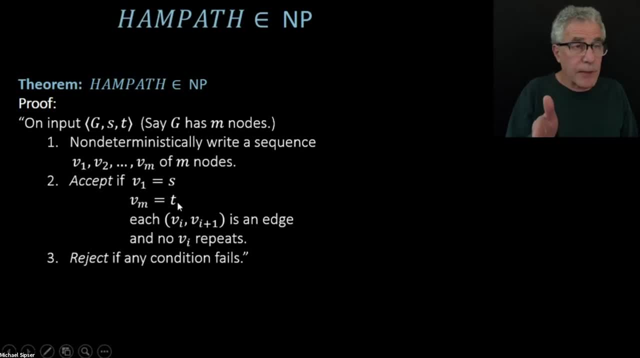 And then, of course. so you're going to, on each branch of the nondeterminism, you're going to check to see whether the conditions have been satisfied And on that branch, if the conditions were not satisfied, that branch is going to reject. 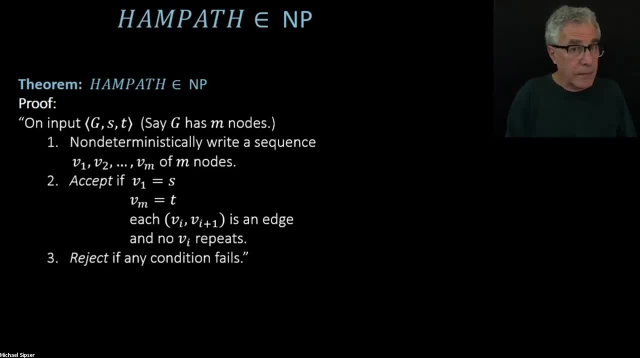 Of course, one of the other branches might yet accept. So That's how nondeterminism works, OK, So I'd like to visualize this. I'd like to visualize this as the tree of the different branches of the computation of M on its input. 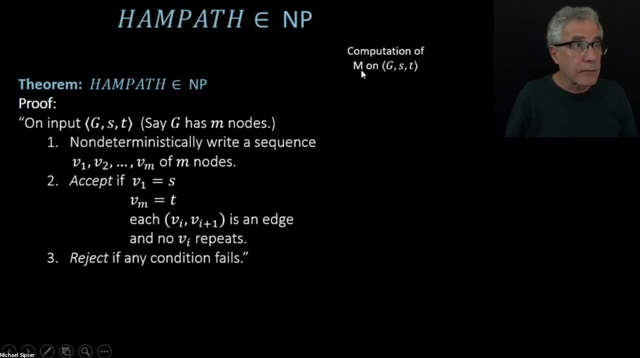 So here is the, here is our nondeterministic. deterministic, It's a Turing machine, which is this one? And you provide it with the input GS and T, And how does the machine actually working, So when I say nondeterministically- write? 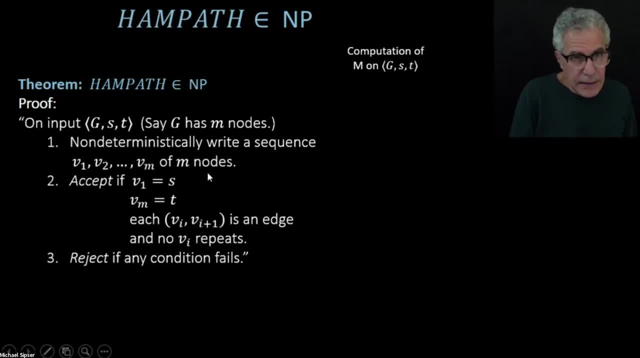 down a sequence of M nodes. this is getting into a little bit more detail than I would normally think about it, because we try to tend to think about things at a higher level. But just for just to get us Started, I think it's good to think about this. 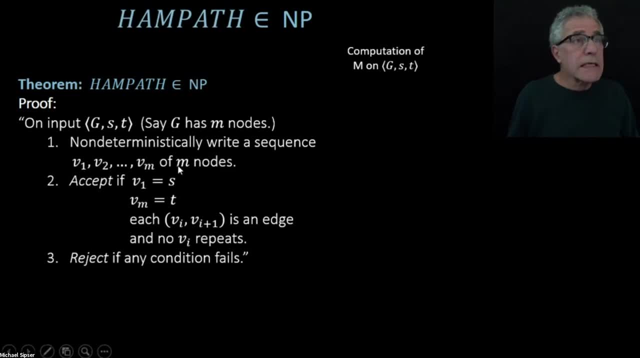 with a bit more detail. So let's think of the nodes, the M nodes, as being numbered, having labels numbered 1 through M, And I'm going to think about them being labeled by their binary sequences. We're going to write down those nodes. 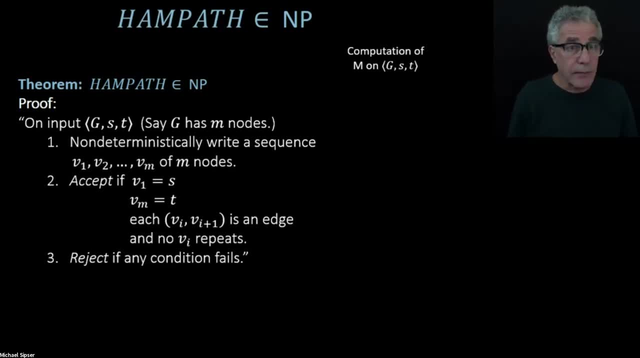 That's how the machine is going to have to operate. on those numbers. for the nodes, We'll think about them as being written in binary And now, As The machine is going to be writing down, let's say, the node V1.. 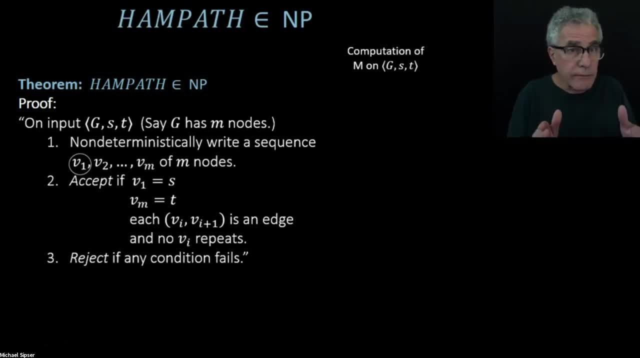 So it's nondeterministically picking the first node of the sequence. What does that actually mean in terms of the step-by-step processing of the Turing machine? M Well, it's going to be guessing via a sequence of nondeterministic moves, the bits. 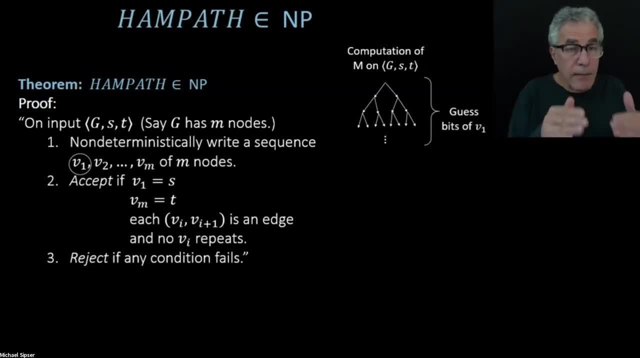 That represent the number of the node for V1.. For example, V1 might be the node number 5 in the graph. Of course, nondeterministically, the machine is on different branches picking all different possible choices for V1.. Those are going to be the different branches here. 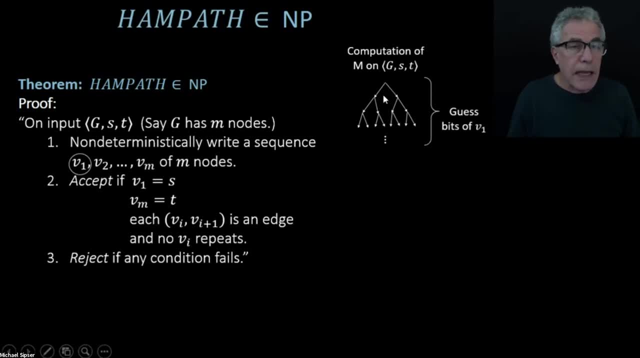 But one of the branches might be, and what I'm really representing here. These are. I probably could have written this down on the slide here in tiny font, but these are like the 0, 1 choices. That's why it's sort of a binary tree here for the writing down. 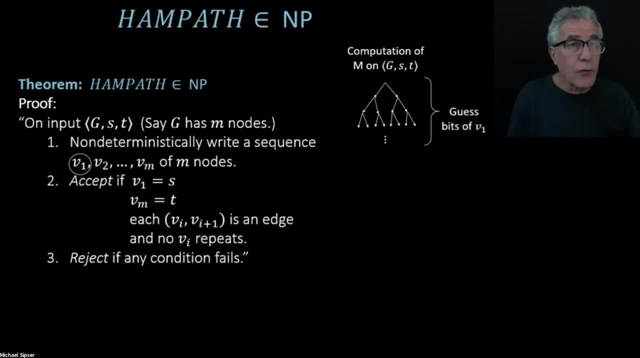 the bits of V1.. So here maybe this could be 1, 0,, 1, representing the number 5, which might be the very first node that I'm writing down in my sequence. Some other branch is going to write down node number 6.. 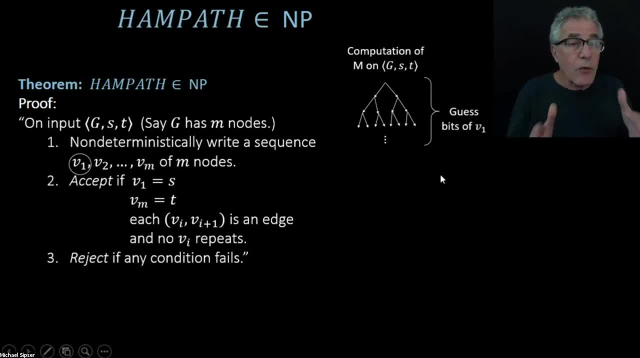 Some other branch is going to write down node number 2. Because, nondeterministically, we're making all possible choices for V1.. That's what I'm trying to show in this little part of the computation of M on this input. So then, after it's finished writing down the description, 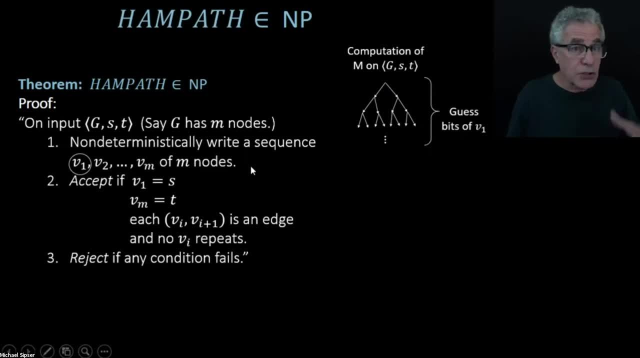 of the node for V1, its choice for V1, it goes down to make choose what V2 is, again nondeterministically. So there's going to be more branches for each possible choice of V2, and so on, node after node. 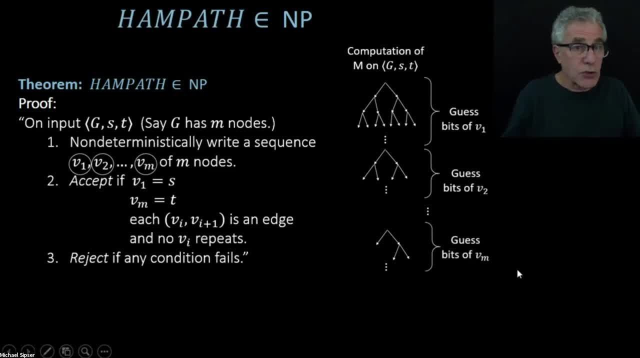 Then it's going to finally get to the last node, Vm. It's going to write down lots of choices for Vm And at this point here we have completed the first stage of the algorithm. Now there's some huge tree of all of the possible choices. 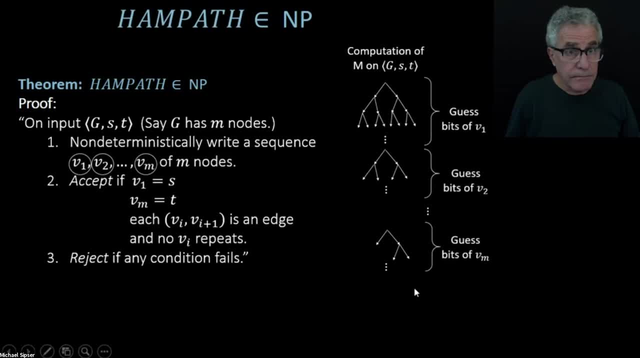 This is for the Vs that have shown up at this point. OK, And now we're going to move into the second phase. So, following this, there's going to be here a bunch of deterministic steps of the machine, So no more branching. 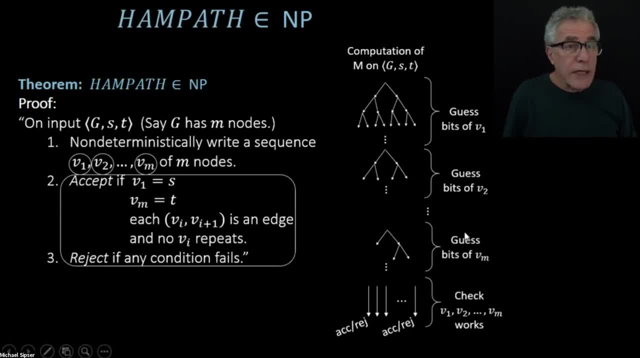 No more branching is needed, Because here we've written down, at this point, at this point, we've reached a point in each of those locations where we've chosen one of the candidates, one of the possible branches, one of the possible paths. 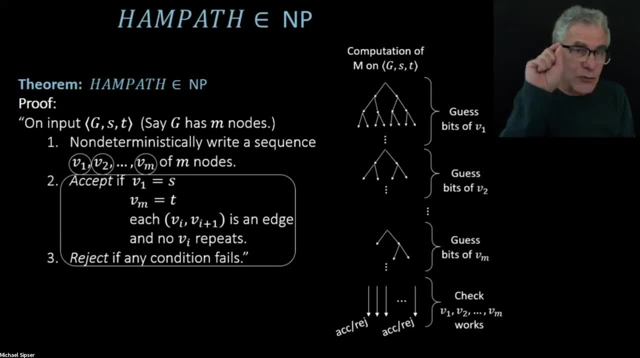 through the machine, one of the possible paths through the graph. I'm sorry. So here we're guessing potential paths in the graph And now we're going to check that we actually have picked a path. that's a Hamiltonian. A Hamiltonian path from s to p, s to t. OK, 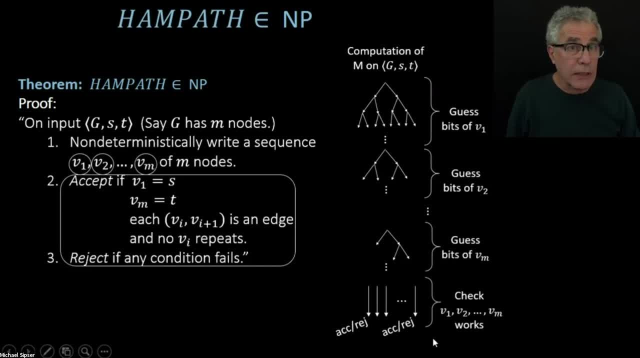 So each one of these branches is now going to end up accepting or rejecting And the whole overall computation is going to accept if at least one of them ended up accepting, which means you actually found a Hamiltonian path. OK, I don't know if that's helpful to you or not. 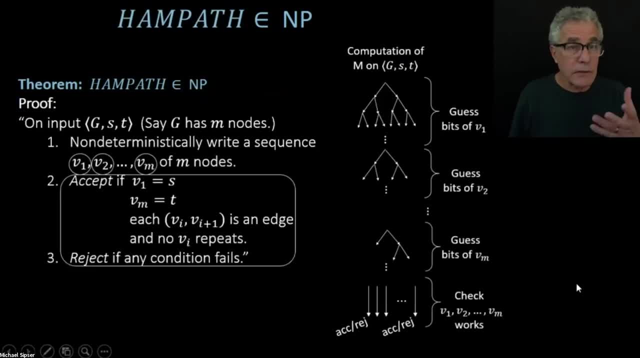 But that is so. we can just, if there's any questions on this, let's see Question on: is there something? OK, You know, trying to draw a connection here between this and computation histories. I mean, there is a pattern here that does come up often. 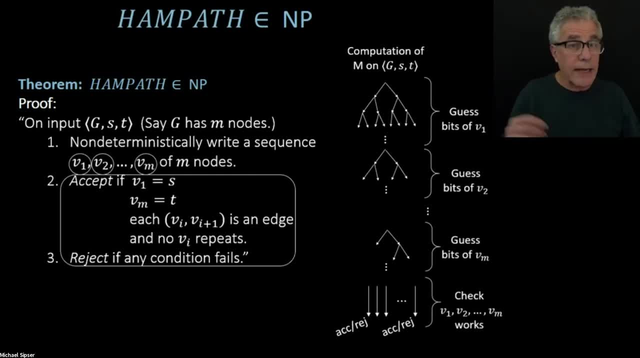 where you want to check something starts right, ends right and that all of the intermediates are right. So I think there is some deeper connection here, probably too hard to explain, But that does have something to do with this Hamiltonian path. 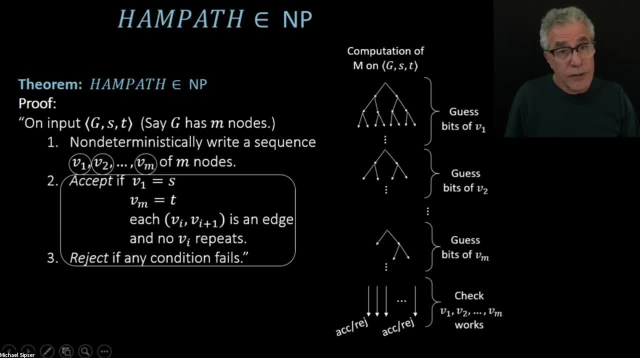 problem. Why are we using binary representation? Well, we're going to talk about the algorithm. would have worked equally well if we used base 3 or base 5 or base 20 as a way of writing down our labels for the nodes. 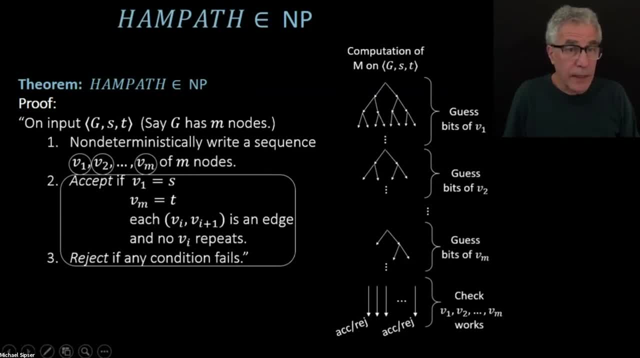 But in a sense it doesn't work that way. Yeah, In a sense it doesn't matter. The alphabet has to be finite. So that's true, I mean. that's why it's not just in a single step of the Turing. 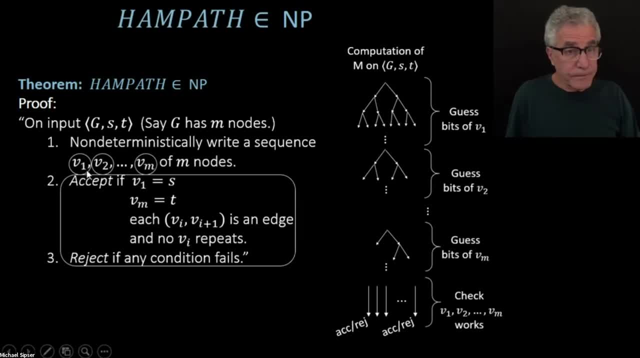 machine that you would pick the node, the choice for v1.. You really have to go to a sequence of steps because each of the branches of the machine only has a fixed number of choices. So you can't, in a single step of the Turing machine, pick. 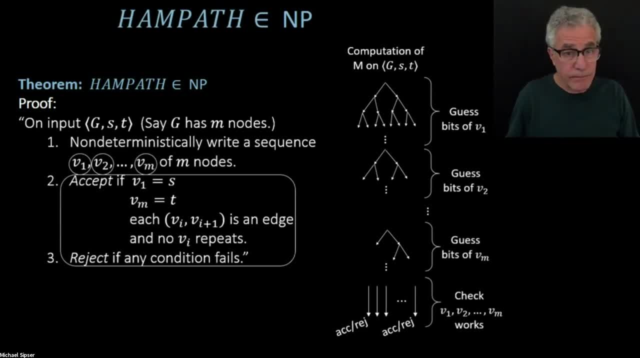 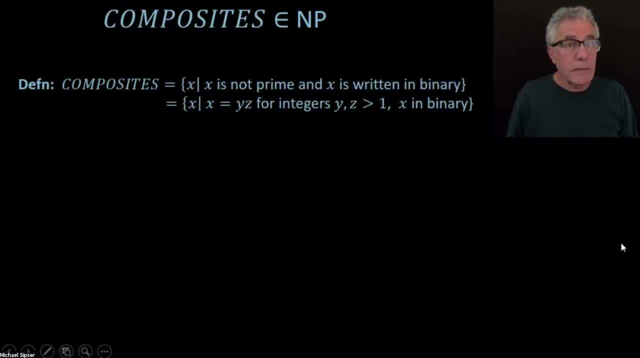 all the different possibilities for v1. It has to go through a sequence. OK, Now let me do a second example, the problem of composites. So the language of all composites are all of the non-primes written as binary numbers again. 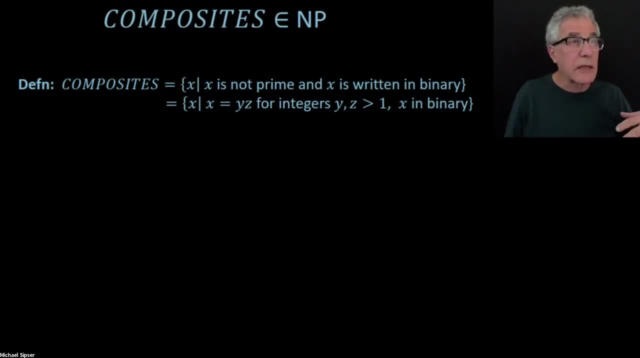 So we'll talk about the base and the representation in a second. But just imagine, You know, You know, You know. These are all of the numbers that are not prime And that language is easily seen to be a member of NP. 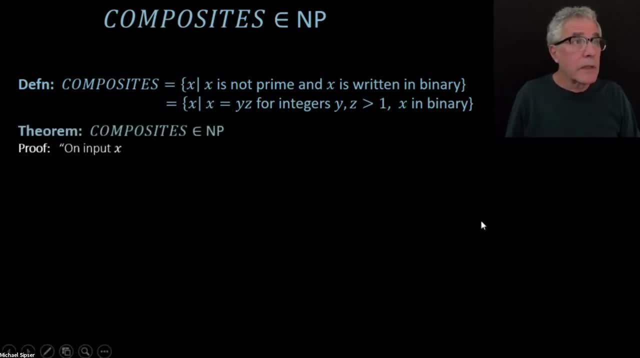 Here is again the algorithm for that: Given x, we want to accept x if it's not a prime number, So it has some non-trivial factor. So first, the way the nondeterministic matrix works, The way the nondeterministic machine is going to work. 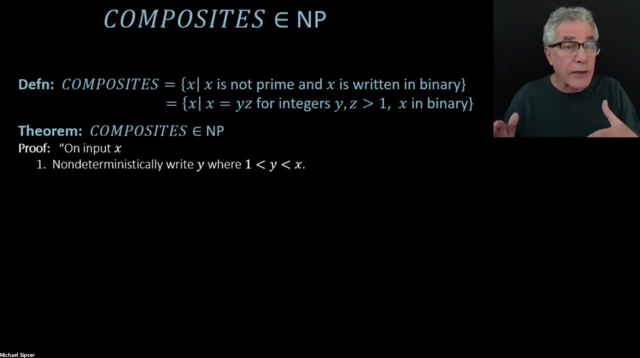 is it's going to guess that factor, So it's nondeterministically, it's going to try every possible factor. y is going to be a number between 1 and x, but not including 1.. That has to be an interesting factor. so not including 1. 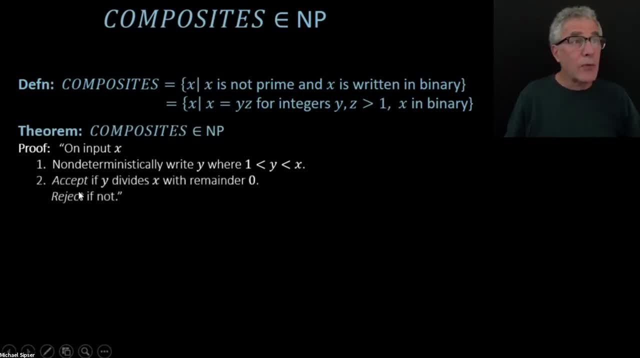 and the number itself. So something strictly in between. And we're going to then, after we've nondeterministically chosen y, then we're going to test to see if y is really a factor. So we'll see if y divides evenly into x, with a remainder of 0.. 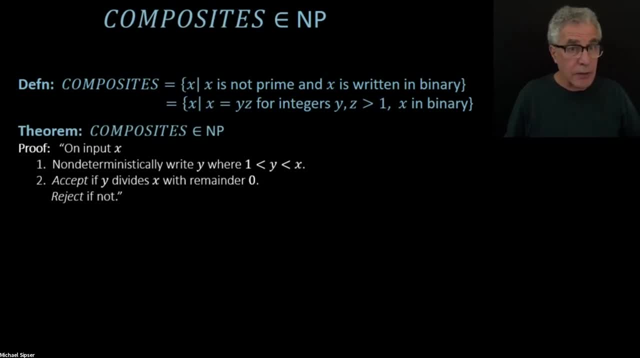 If that branch successfully picked the right y, it's going to accept. And some other branch might have picked the wrong y will not. And if x is really a composite number, some branch will find the factor. Now the base doesn't matter. 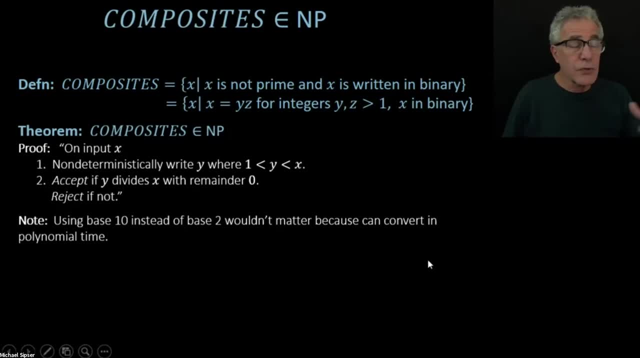 Could have used base 10. Because you can convert one base to another. So this is really in terms of our representation of the number. But I do want to make one point here that changing, we don't want to write the number in unary. 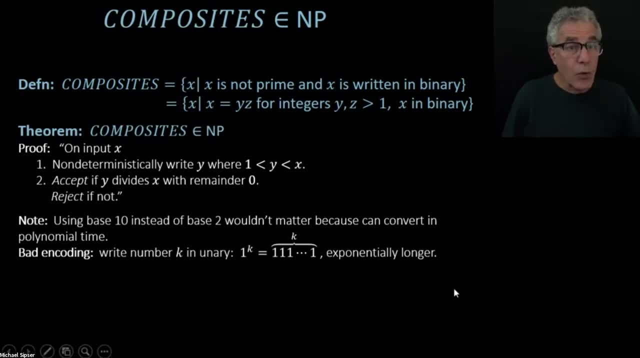 just as writing the number k as a sequence of k1s. That's not really a base, That's just an exponential representation for the number And that changes the game, because if you make the input exponentially larger then it's going to change whether the algorithm relative 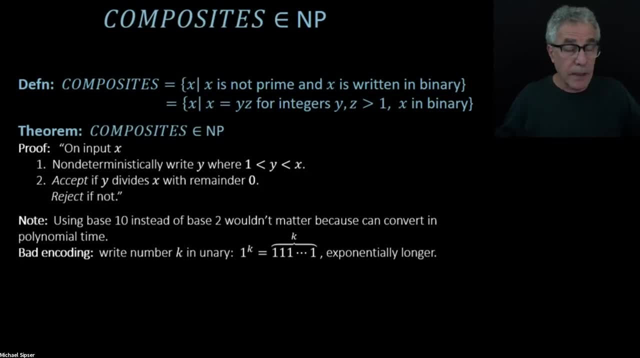 to that exponentially larger input is polynomial or not. So an algorithm that might have been exponential originally when the number is written in binary might become polynomial if the number is written in unary. And I do want to mention as a side note that the composites 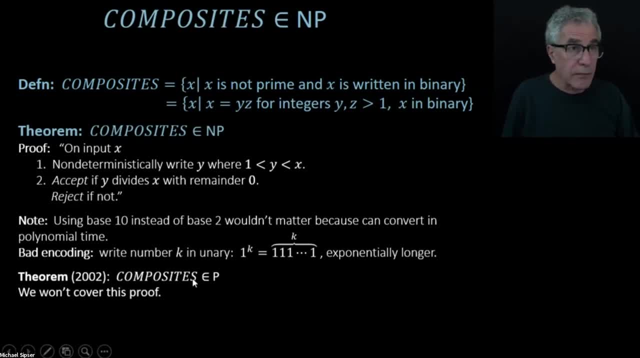 language Or primes, for that matter. Both are in P, But we won't cover that. So whereas the Hamiltonian path problem is not known whether it's in P, the primes and composites problem are in P. So that was known. 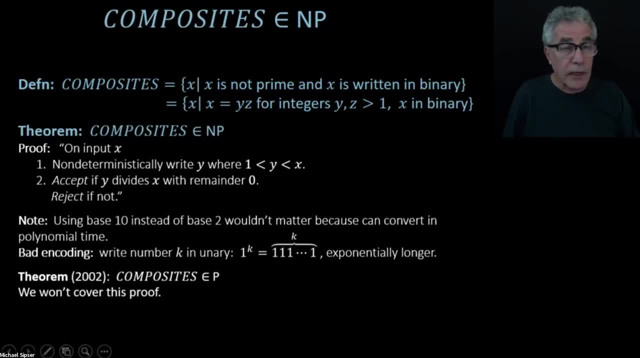 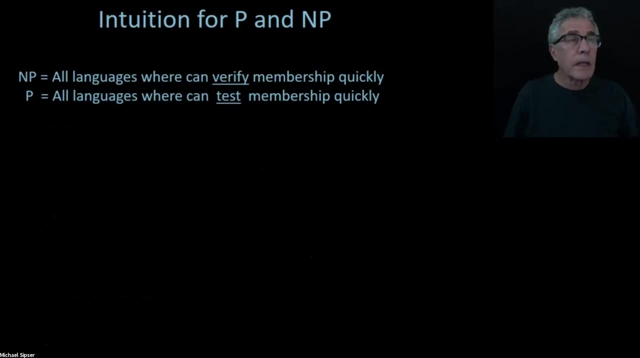 That was actually a very big result in the field, solved by folks at one of the Indian Institutes of Technology back About almost 20 years ago now. OK, so let's turn here to trying to get an intuitive feeling for P and NP. 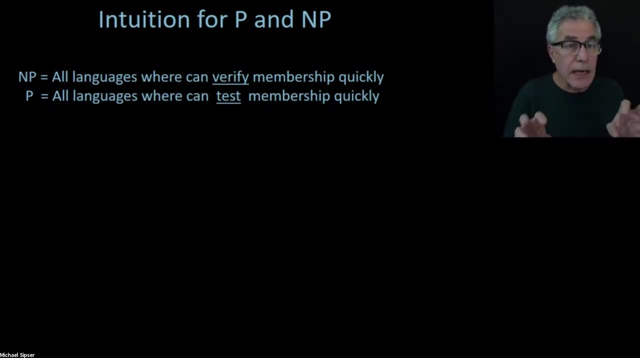 And we'll return now to this notion of NP corresponding to easy verifiability. So NP are the languages where you can easily verify membership quickly, And I'll try to explain what that means. In contrast, P are the languages where you can test membership quickly. 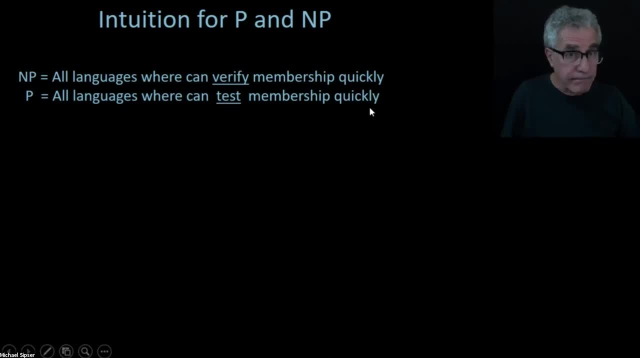 By quickly I'm using polynomial time. That's going to be basically for us. that's what quickly means in this course. So in the case of the Hamiltonian path problem, the way you verify the membership is you give the path. 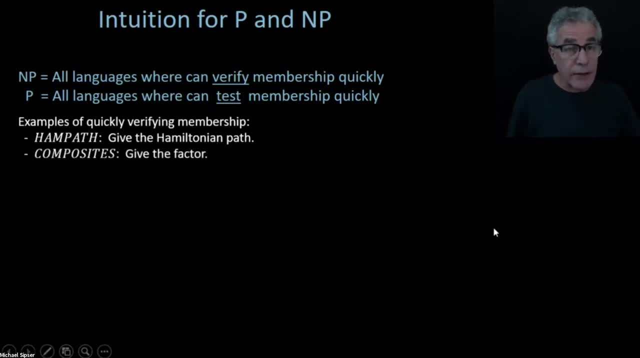 In the case of the composites, the way you verify the membership is you give the factor. In those two cases, and in general when we have a problem, that's in NP, we think of this verification as having a giving. we give it a special name, called a certificate. 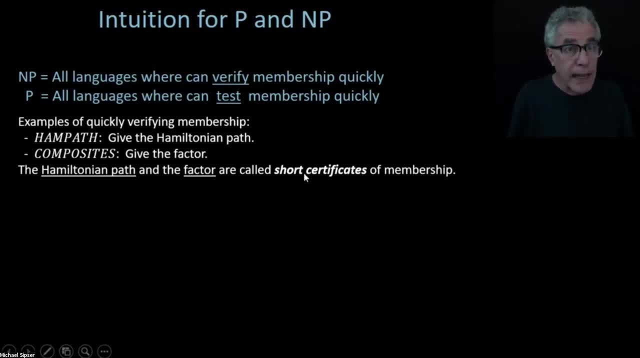 or sometimes a short certificate, to emphasize the polynomiality of the certificate. It's like a way of proving that you're a member of the language. In the case of composites, the proof is the factor. In the case of HAMPATH, the proof. 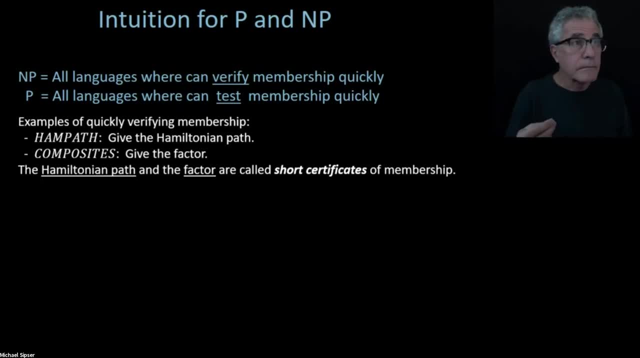 is the path, the Hamiltonian path. Contrast that. for example, if you had a prime number, Proving a number as composite is easy because you just exhibit the factor. How would you prove that a number is prime? What's the short certificate of proving that some number? 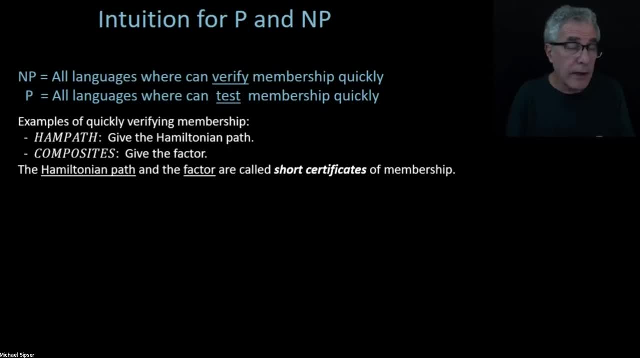 has no factor. That's not so obvious. In fact, there are ways of doing it which I'm not going to get into. in the case of testing of numbers, prime, and now it's even so known to be in p, so that's even better. 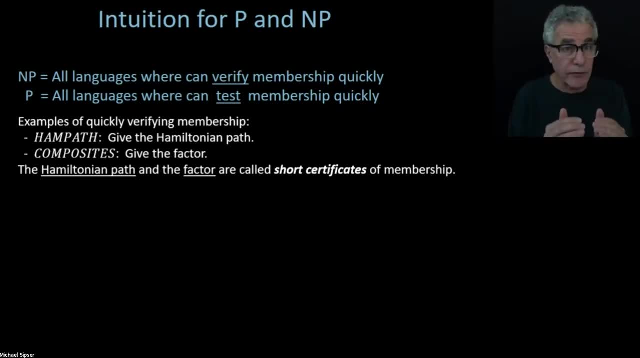 But there's no obvious way of proving that a number is prime with a short certificate. Yes, Yes, Yes. And so this concept of being able to verify when you're a member of the language, that's key to understanding NP. That's the intuition you need to develop and hopefully take away from today's lecture, or at least by thinking about it and reading the book, and so on. 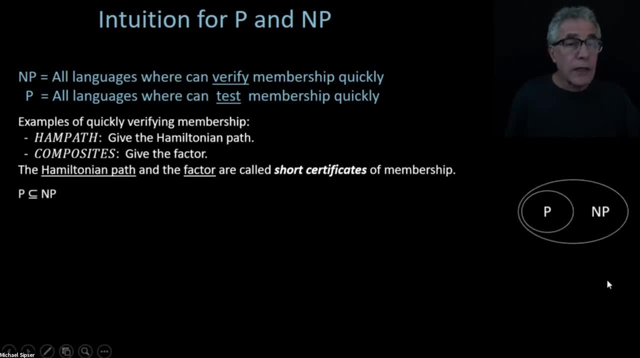 So if you compare these two classes, P and NP, P, first of all, is going to be a subset of NP, both in terms of the way we defined it, because deterministic machines are a special case of non-deterministic machines. 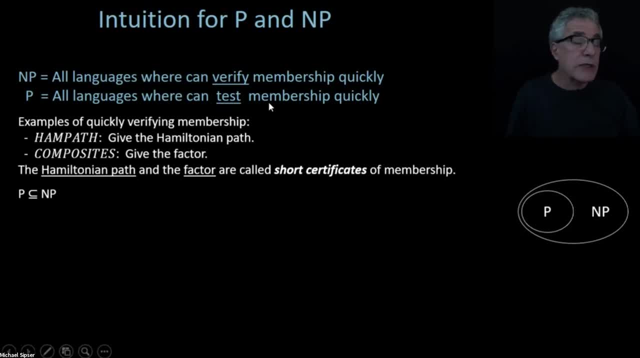 But also if you want to think about testing membership. if you can test membership easily, then you can certainly verify it in terms of the certificate. You don't even need the certificate. It's irrelevant at that point, Because whatever the certificate is, you can still test yourself whether the input is in the language or not. 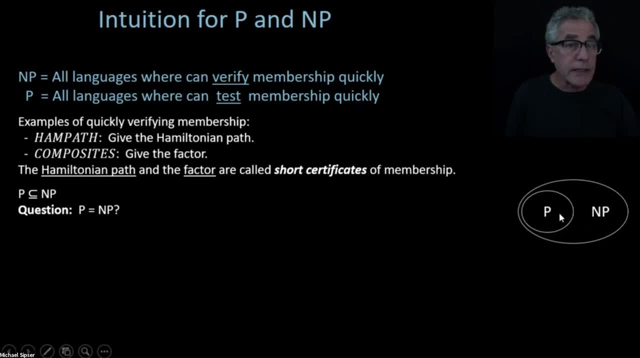 The big question, as I mentioned, is whether these two classes are the same. So does being able to verify membership quickly, say with one of these certificates, allow you to dispense with the certificate, not even need a certificate and just test it for yourself? 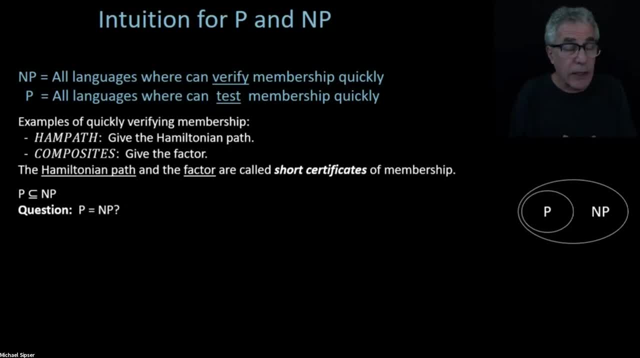 Whether you're in the language And do that in polynomial time. That's the question For a problem like Hamiltonian path. do you need to search for the answer if you're doing it deterministically, Or can you somehow avoid that and just come up with the answer directly with a polynomial time solution? 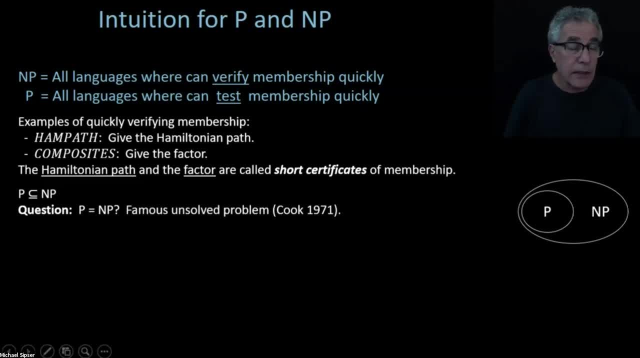 Nobody knows. We don't know the answer to that, And it goes back, at this point, quite a long time. It's almost 60 years now that that problem has been around. 60 years? No, that would be 50 years. 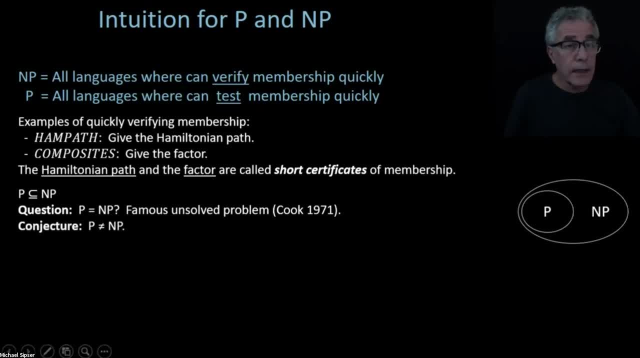 No, 50 years, Almost 50 years. So most people believe that P is different from NP, In other words that there are problems in NP which are not in P, And so the candidate would be the Hamiltonian path problem. But it seems to be very hard to prove that. 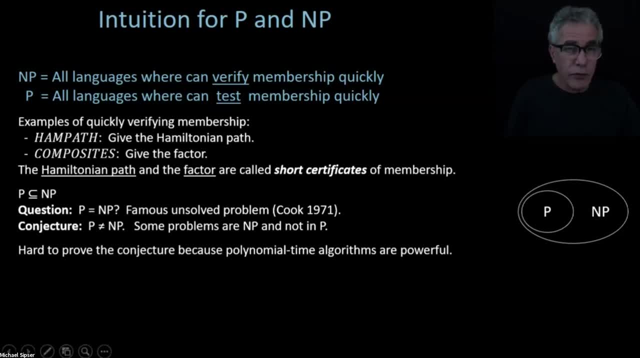 And part of the reason is: I mean, how do you prove that a problem like Hamiltonian path does not have a polynomial time algorithm? It's very tricky to do that because the class of polynomial time algorithms is a very rich class. Polynomial time algorithms are very powerful. 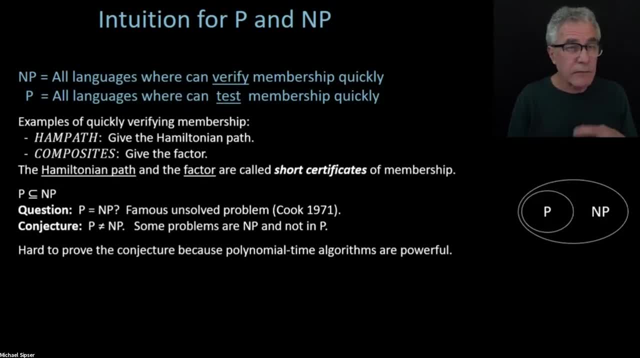 And to try to prove there's no clever way of solving, for example, the Hamiltonian path problem. I mean, the Hamiltonian path algorithm is very rich of solving the Hamiltonian path problem just seems to be beyond our present-day mathematics. 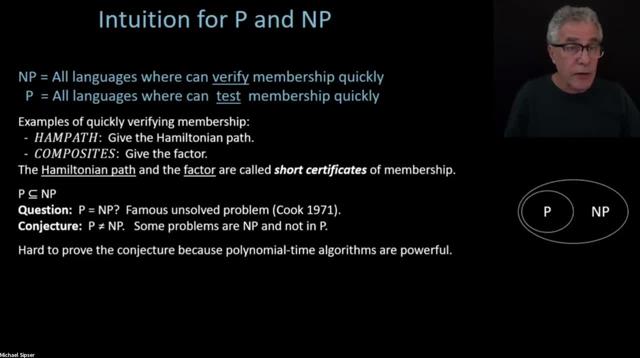 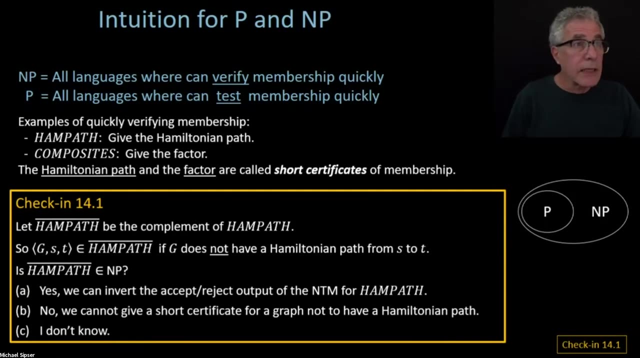 I believe someday somebody is going to solve it, But so far no one has succeeded. So what I thought we would do is I think I have a check-in here, Yes, And then we'll stop for a break. So let's look at the complementary problem. 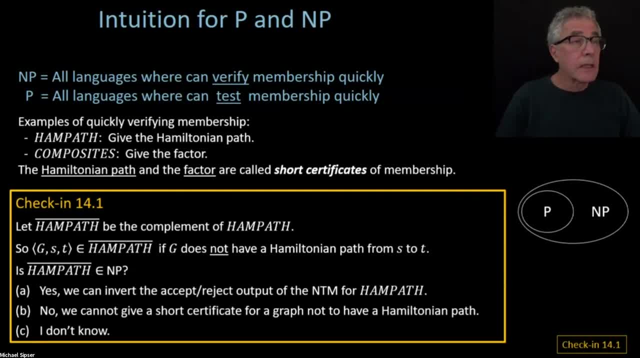 the ham-path complement. So you're in the language now if you don't have a path. So is that complementary problem in NP? OK, so for that to be the case, we would need to have short certificates of when a graph does not have a Hamiltonian path. 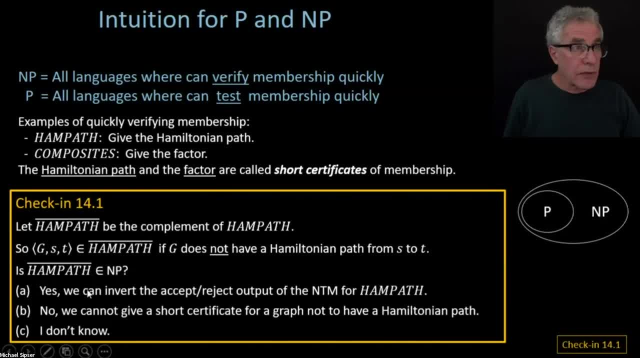 So I leave it to you. So there are three choices. OK, I'm going to stop here, so make sure you get your participation credit here. I'm going to end the polling now. Interesting, so the majority is wrong. Well, I don't know. wrong, we don't know. 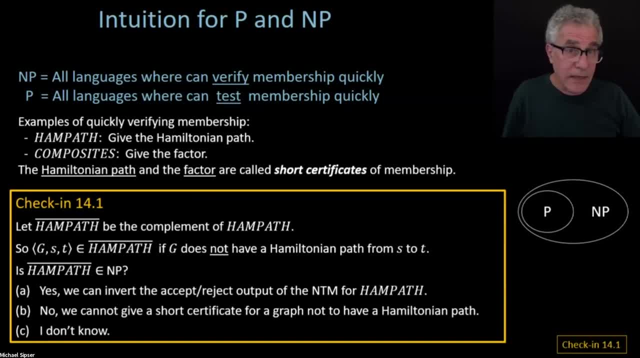 I think the only fair answer Fair answer to this question is C, Because we don't know whether or not we can give short certificates for a graph not to have a Hamiltonian path. If P equal to NP, then you can test in polynomial time. 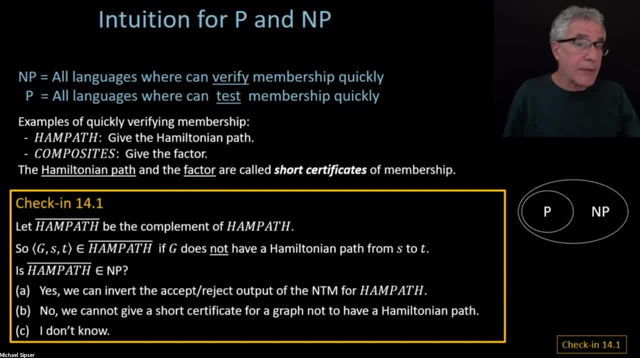 whether a graph has a Hamiltonian path, And then the computation itself would be a certificate- whether it has a path or whether it doesn't have a path, Because it would be something that you can check easily. OK, So, since we don't know for sure that P is different from NP, 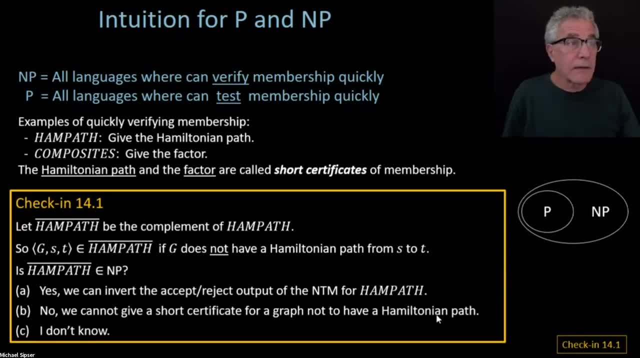 P could be equal to NP, then it's possible that we could give a short certificate, namely the computation of the polynomial algorithm. So the only really reasonable answer to this question is that we don't know. So just ponder that. I think the thing that those of you who answered yes, however, 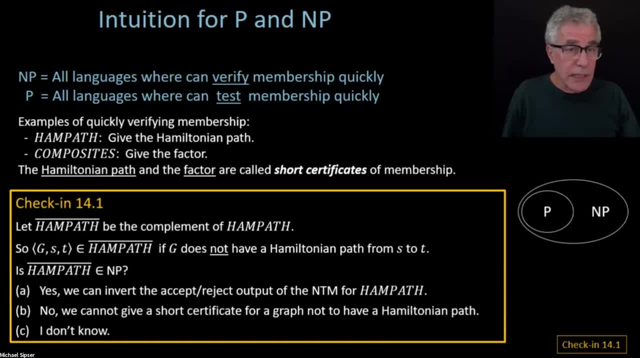 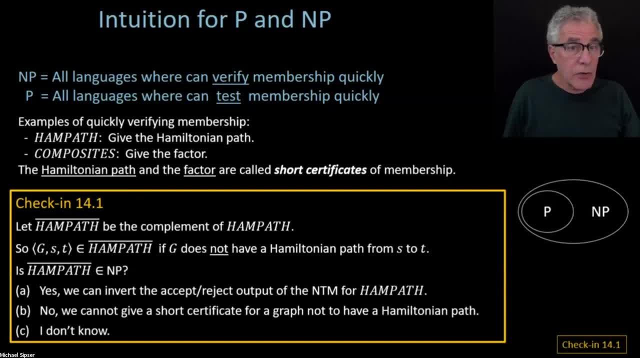 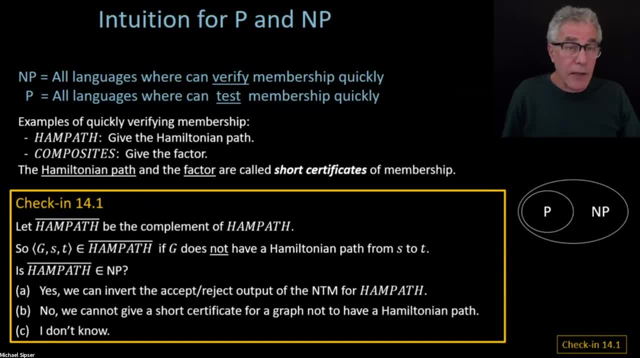 If you remember, the complement of a pushdown automaton is not a pushdown automaton. If you have a nondeterministic machine and you invert all of the responses on each of the branches, it's not going to be recognizing or deciding the complementary language. 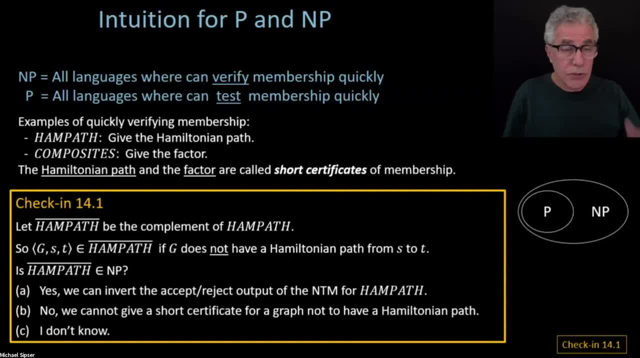 So, because I think that this is something you, if you answered yes, you need to go back and make sure you understand why yes is not a reasonable answer to this question, Because that's not how nondeterminism works. So you have a not complete understanding. 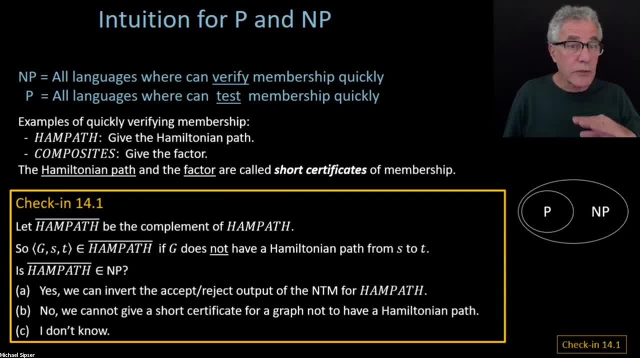 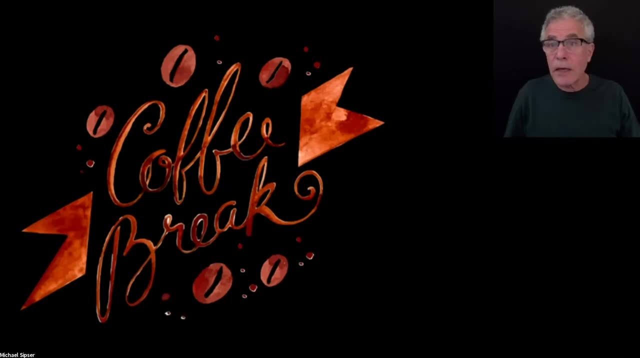 of nondeterminism, And that's going to be really important for us going forward. So I really urge you to figure out and understand why yes is not a good answer to this check-in. OK, so I think we can talk about that more over the break. 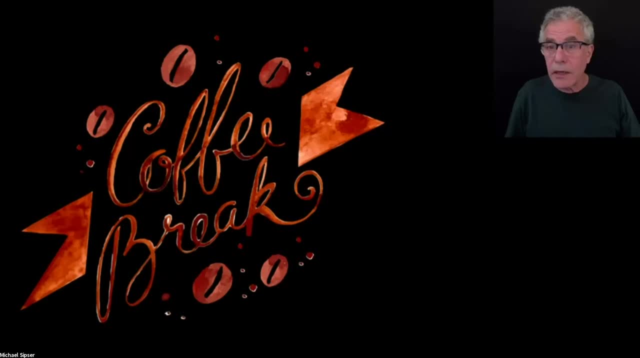 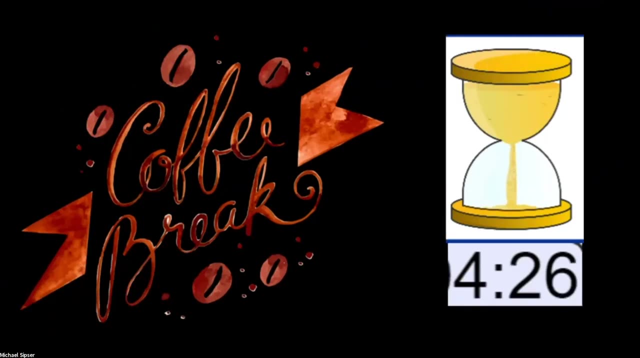 And so we'll return here in five minutes. Somebody is asking about infinite sequences be generated by the machine. When we're talking about- especially in the complexity section of the course, all of the computations are going to be bounded in time, So we're not going to be thinking. 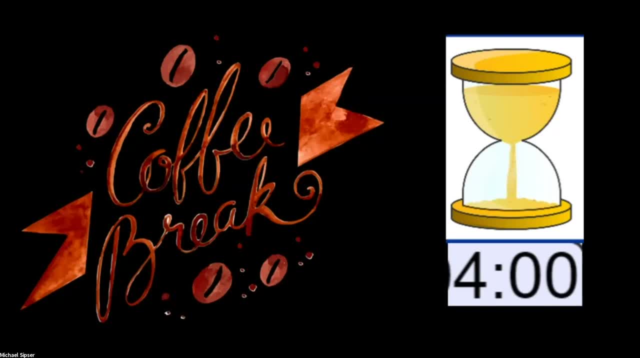 about infinite runs of the machine. That's not going to be relevant for us, OK, So let's not think about that. How does the Turing machine perform division? How does a Turing machine perform division? Well, how do you perform division? 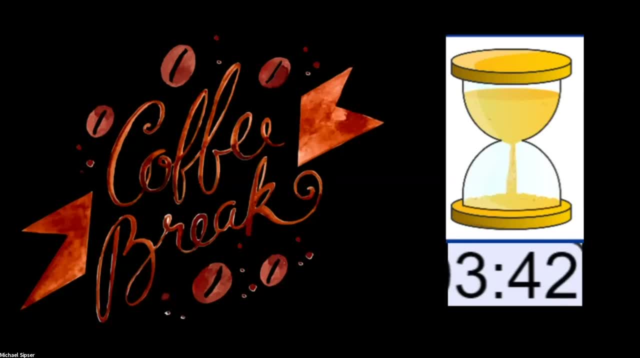 The long division is an operation that can run in the long division procedure that you learn in grade school. You can implement that on a Turing machine. So yes, a Turing machine can definitely perform do long division or division of one integer by another in polynomial time. 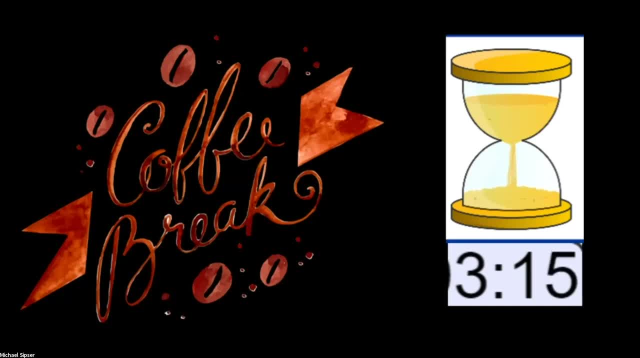 OK. another question: Can we generally say: try dividing y by x, Or do we have to enumerate a string of length y and cross off every No? I think that's the same question. I mean, how would, if you have numbers written in binary? how? 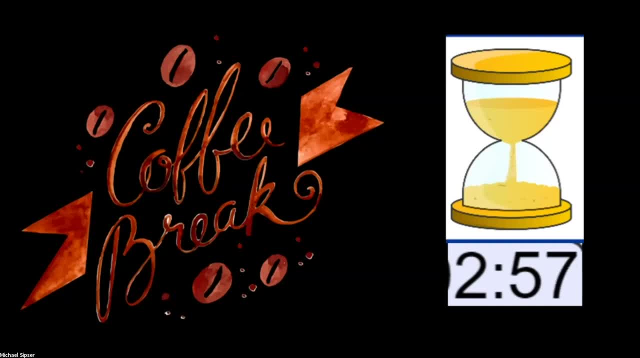 would you do division? You're not going to use long division. Anything such as the thing that's proposed here by the questioner is going to be an exponential algorithm, So don't do it that way. Why does primes in P, composites in P, not implied primes in P? 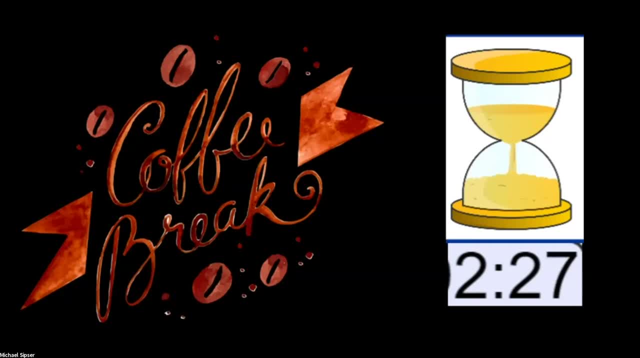 It does imply If composites are in P, then primes is in P as well, Because you can. just when you have a deterministic machine you can flip the answer. When you have a non-deterministic machine, you may not be able to flip the answer. 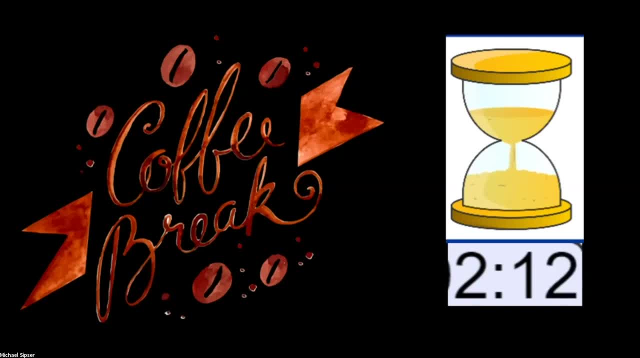 So the deterministic machine just having a single branch, you can make another deterministic machine that runs in the same amount of time. that does the complementary language, Because for deterministic machines, just like for deciders in the computability section, you can just invert the answer. 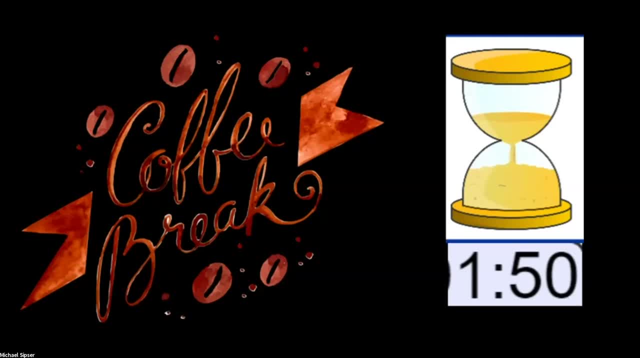 There is an analogy here between P and decidability and NP and recognizability. It's not an airtight analogy here, but there is some relationship there. Somebody's asking me the implications of P equal to NP. Lots of implications. 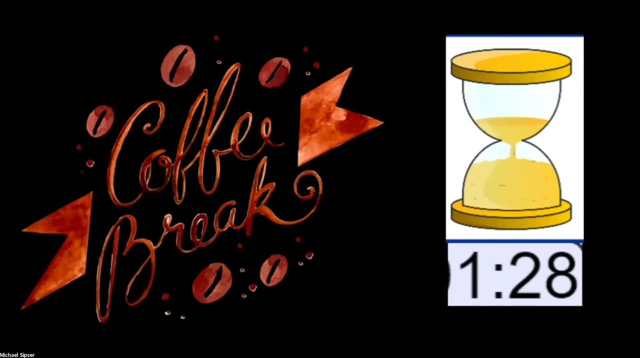 Too long Too enumerate now. But, for example, you would be able to break basically all cryptosystems that I'm aware of if P equal to NP. So we would have a lot of consequences. Somebody's asking so composites, primality and compositeness testing. 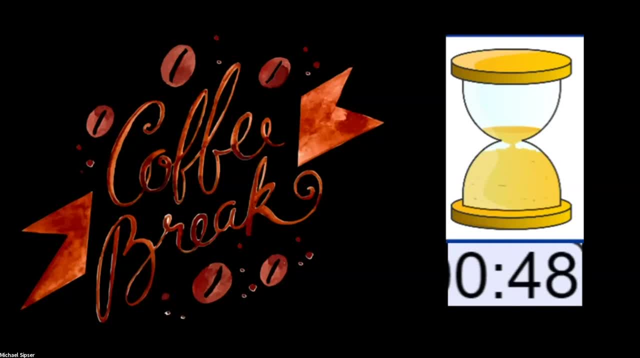 is solvable in polynomial time, But factoring, interestingly enough, is not known to be solvable in polynomial time. I mean, We may talk about this a little bit toward the end of the term if we have time. But the algorithms for testing whether a number is 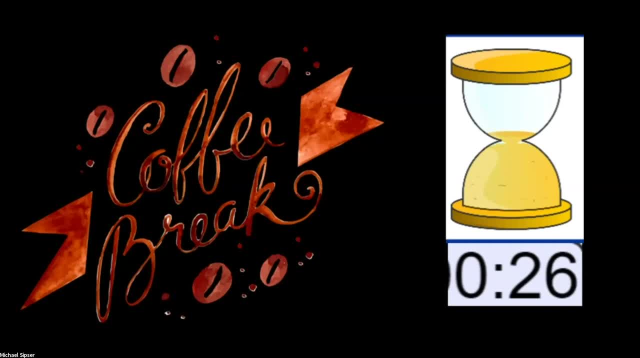 prime or composite in polynomial time do not operate by looking for factors. They operate in an entirely different way. basically by showing that a number is prime or composite, by looking at certain properties of that number, but without testing whether it has a number or not. testing, but without finding a factor. 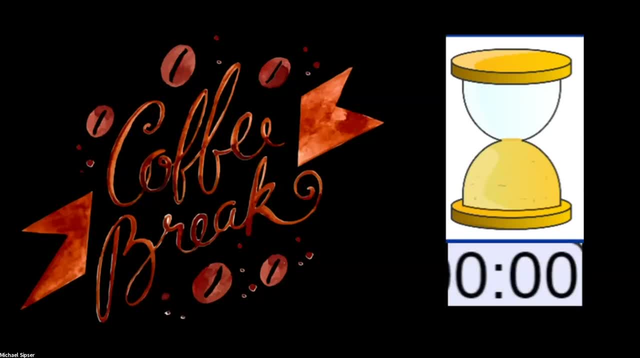 OK, Another question here about asking the: when we talk about encodings, do we have to say how we encode numbers, values? No, we don't have to. We usually don't have to get into spelling out encodings, as long as they're reasonable. 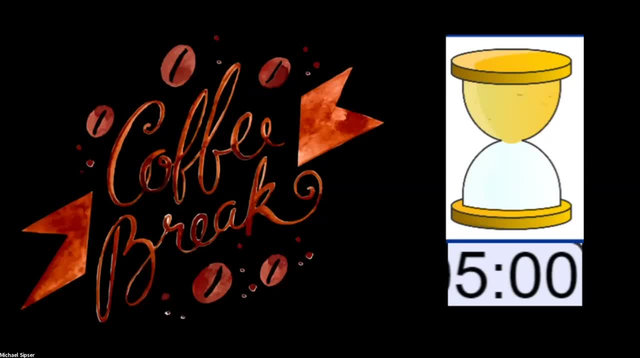 They're reasonable encodings, So you don't have to. Usually, we're going to be talking about things at a high enough level that the specific encodings are not going to matter. OK, let's return to the rest of our lecture. 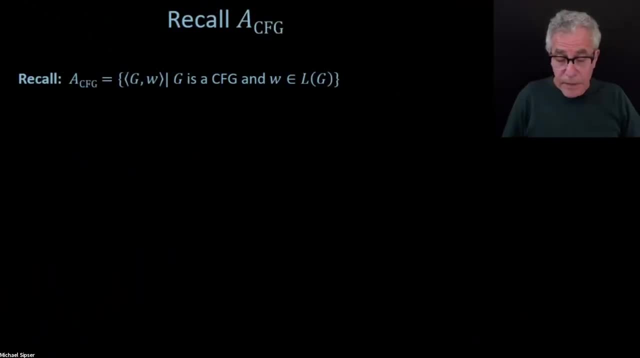 When we talk about, say this, P versus NP problem, and how do you show that? OK, So a problem might not be solvable in P, like the Hamiltonian path problem. Many people who are not practitioners in the field know about the P versus NP problems. 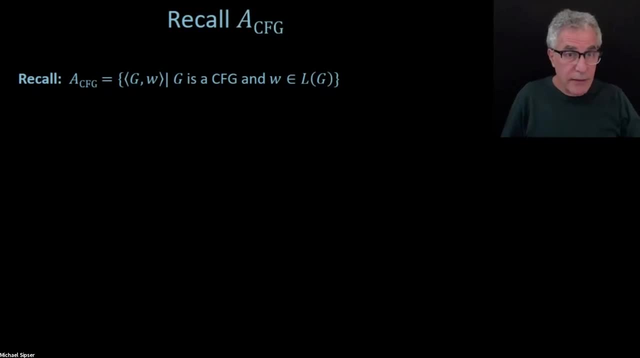 Over the years, I've gotten many, many emails and physical letters from people about that, Since people, since I've spent some time thinking- I'm known as having spent some time thinking about it- And people claim to solve the problem. solve P is NP. 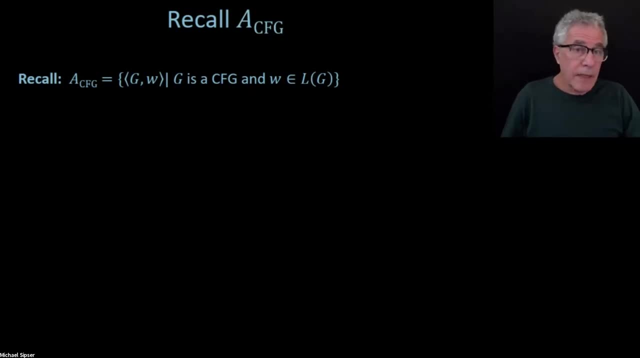 the P versus NP problem by basically saying problems like the Hamiltonian path or other similar problems. basically there's clearly a problem. There's clearly no way to solve them without searching through a lot of possibilities, And then they go through a big, long analysis. 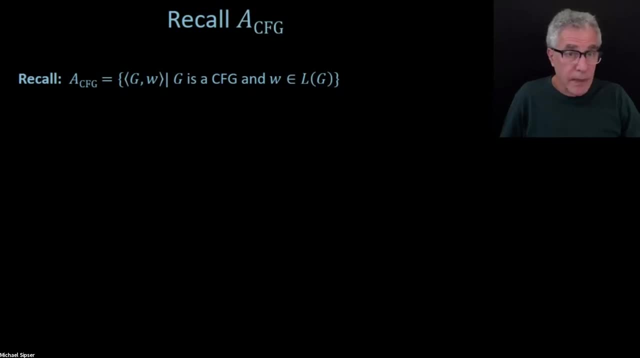 showing that there are exponentially many possibilities And a lot of the proofs that claim to solve P versus NP. they all look like that. Somewhere in that paper there's going to be a statement along the lines to solve this problem. clearly you have to do it this way. 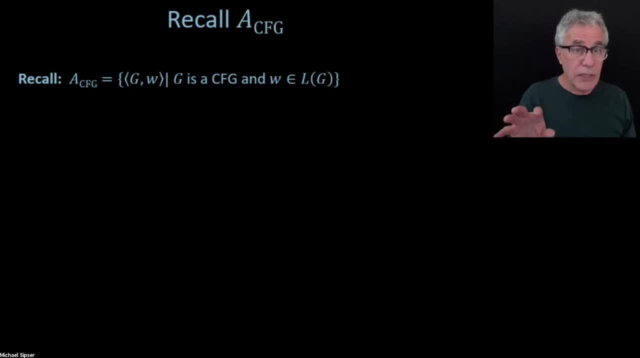 And that's the flaw in the reasoning, Because, just like for the factoring problem, just like for the composite testing problem, you don't necessarily have to solve it. used by searching for factors, There might be some other way to do it. You might be able to solve a Hamiltonian path problem. 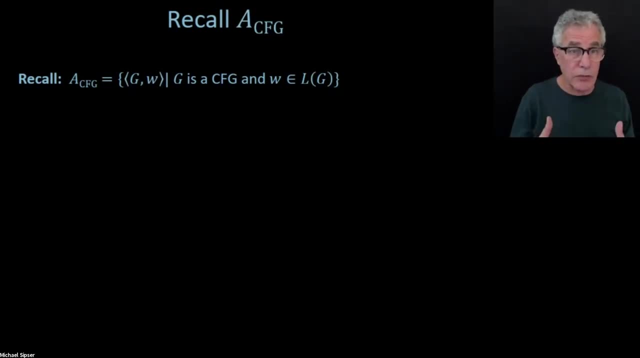 without searching for Hamiltonian paths. There might be some other process that you can use which would give you the answer. So the class of polynomial time algorithms is very rich. It can do many, many things, And I wanted to present to you one. 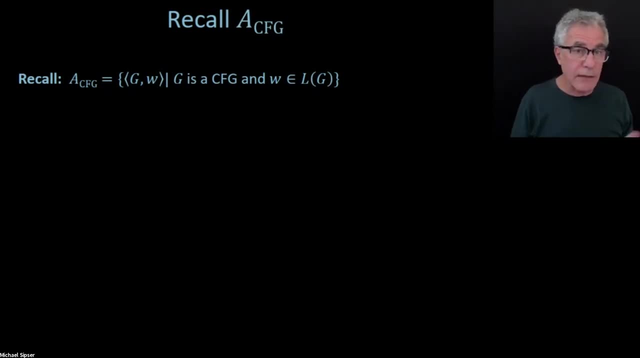 of the most important polynomial time algorithms. In a sense. it's kind of, you can make a certain argument that this is sort of, in a sense, the most fundamental polynomial time algorithm- Some people might argue with me on that- And that's a process called dynamic programming. 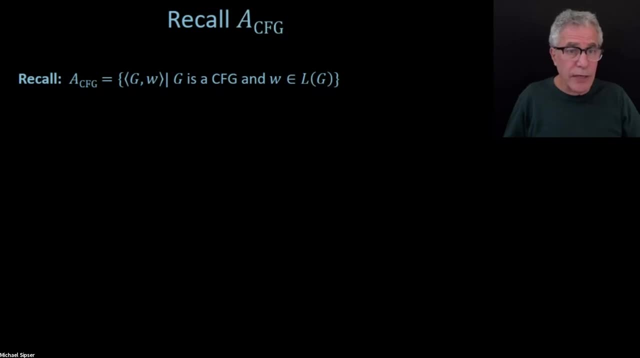 OK, which I'm sure some of you have seen already in your algorithms classes and some of you may not have, But since you have a homework problem on it, I want to spend a little time describing it to you, And that's useful for solving this ACFG problem, which you may remember. 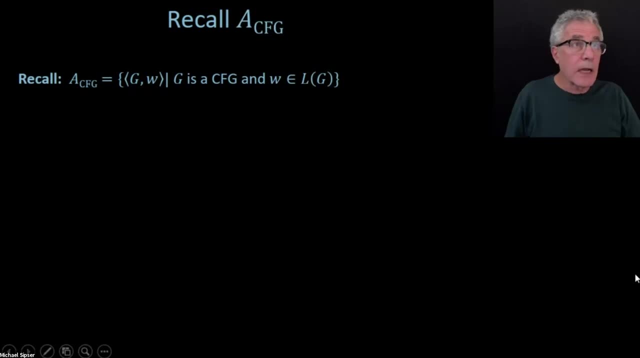 from the first half of the course involving testing if a grammar generates a string. So you remember this ACFG problem. You're given a grammar context-free grammar and a string And I want to know, is it in the language of the grammar? So that's going to. 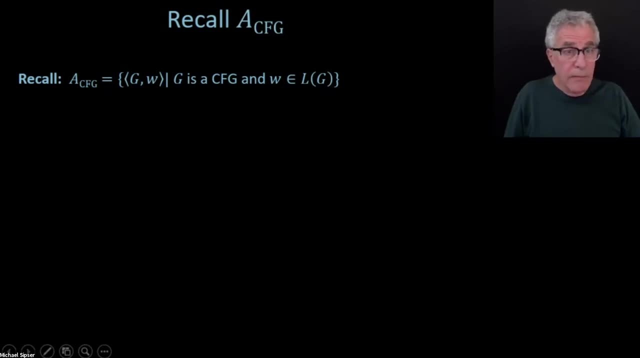 turn out to be solvable in polynomial time, but only with a kind of a clever algorithm. Remember, it's decidable. We decided it by converting, by making sure that you are converting the grammar in Chomsky-Chamberlain Chomsky normal form. Then all the derivations have a certain length. You just try all the. 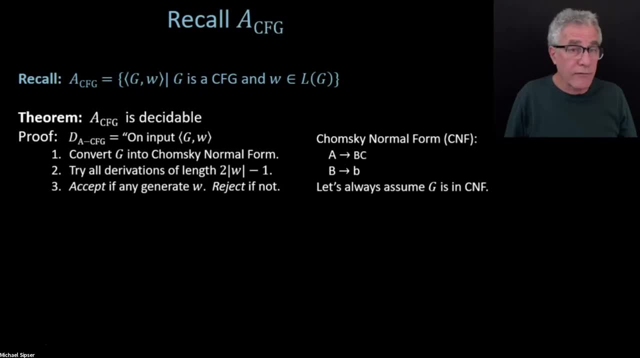 possible derivations of that length and you accept if any of those derivations generate W. You may remember that from the first half of the course That immediately gives an NP-type algorithm for this language, Because basically you non-deterministically, instead of trying them all sequentially, all of these derivations. 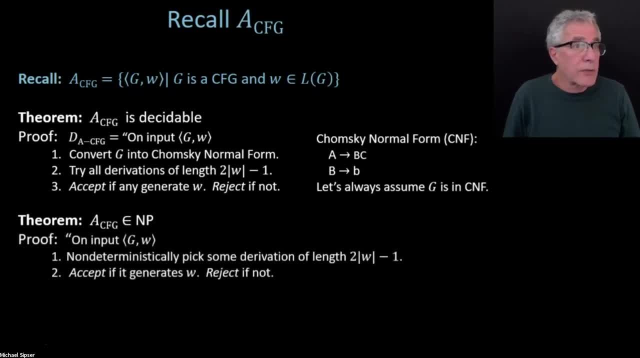 you try them in parallel, non-deterministically. So non-deterministically, you pick some derivation of that length and you accept if it generates the input. This classically fits our model of NP. You can think of it as guessing the derivation and checking that it works- or in parallel. 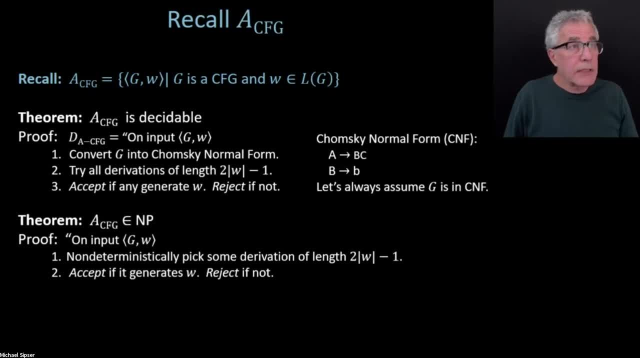 writing down all possible derivations, derivations. But this AC of G problem is classically an NP problem, probably in NP, And if you just imagine that, so what's going to be the certificate? If you found an input that's in the language that's. 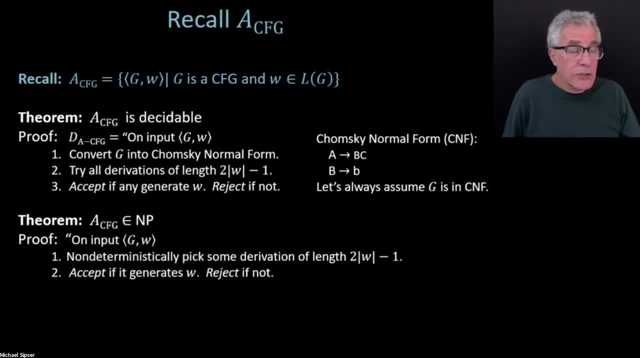 generated by the grammar. the certificate is a derivation. So if you look at it that way, you might think: well, that's the best you can do. This is going to be an NP problem in NP and there's not going to be a way of avoiding. 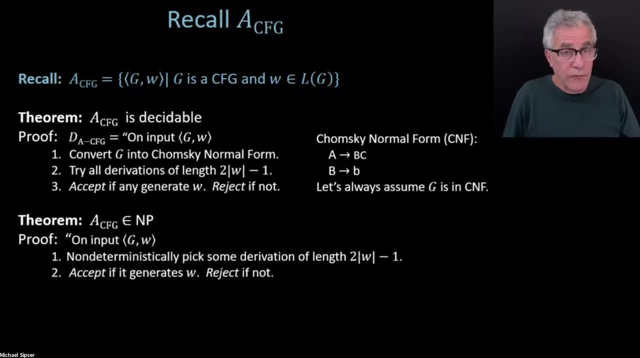 searching for the derivation. But that's not true. There is a way of avoiding searching for the derivation. You can build up the derivation using dynamic programming, And so that's what I wanted to describe for you how that works, also partly because it's a homework. 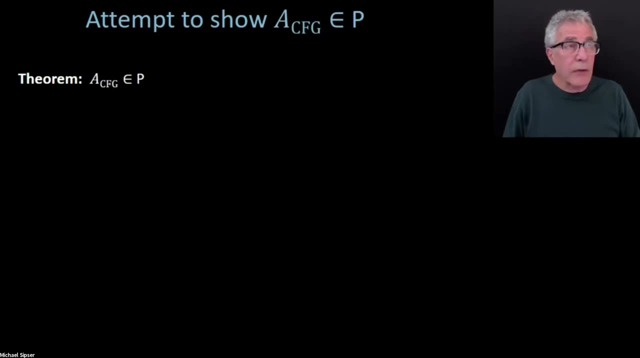 problem, And I think dynamic programming is a very important algorithm. So before we describe what dynamic programming is, which is very simple, by the way- let's try to work up to it by making an attempt to solve this problem just using ordinary recursion. 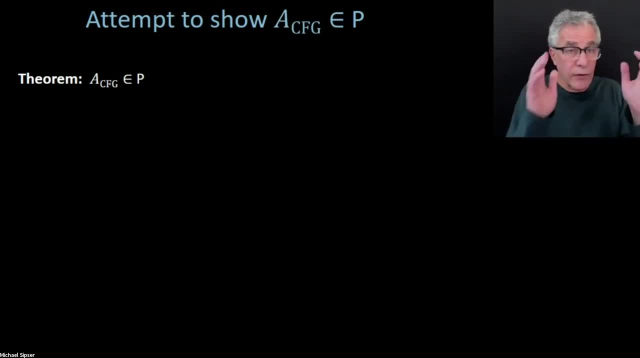 So how would we solve the AC of G problem? So you're given a grammar, You're given an input. Let's assume the grammar is in Chomsky normalization. It's in Chomsky normal form, so that's going to be useful. 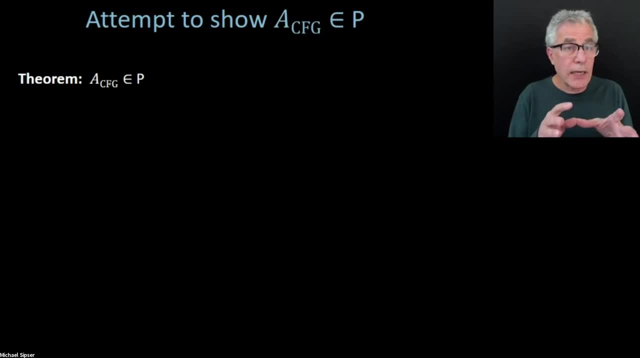 So it's a Chomsky normal form grammar And we want to see how to test if you can generate w, And it's going to be recursive algorithm. Recursive algorithm is going to actually solve something slightly more general. I'm going to give you the grammar. 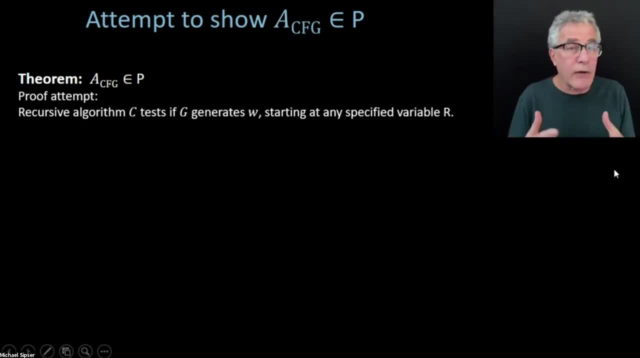 I'm going to give you the string And I'm also going to allow you to start at some other variable. so I'm going to give you some variable r And I know I want to know: can I generate w starting at r? So that's my slightly more general problem. 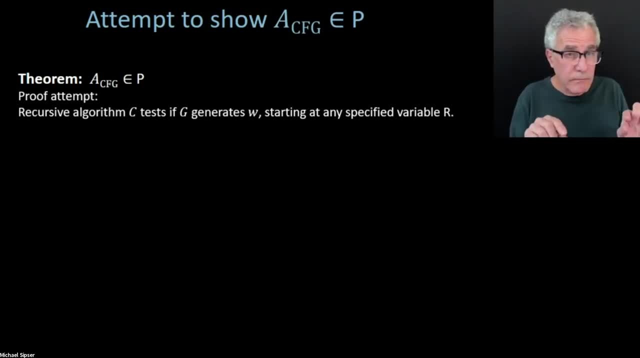 which is going to be useful in the recursion. So the input now to this algorithm is the grammar, the input and the starting variable. And now how is the algorithm going to work? It's going to try to test. can I get to? 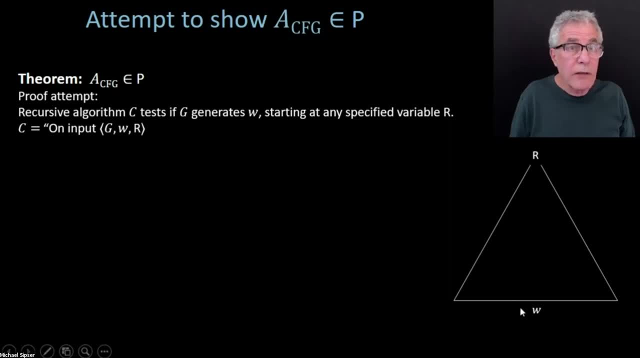 is there some derivation, pictured here as the parse tree, for w starting at r? That's what the algorithm is trying to answer. Can I get w from r? The way it's going to do that is it's going to try to divide w into the two strings. 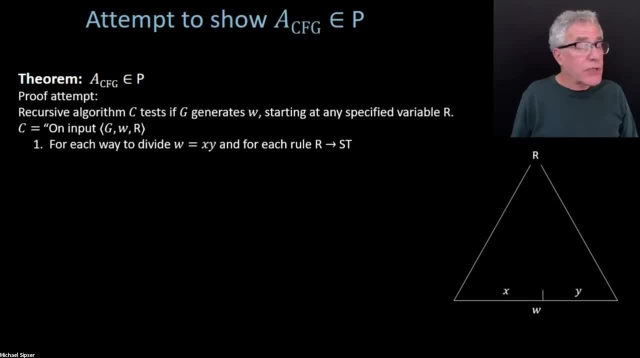 in all possible ways, Which sounds like it might be exponential, but it isn't. There's only a polynomial, polynomial number of ways to divide the string into two substrings. just a border n, just depending on the way you make that cut. 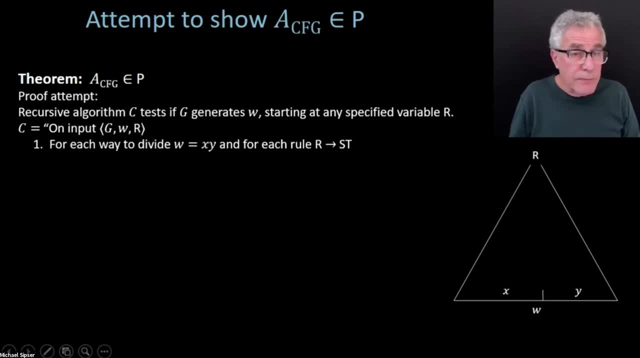 So there's some, so that's not too bad. There's a polynomial, there's only n ways of making that division And also I'm going to try every possible rule that comes from R that generates two variables. So these are what's allowed in Chomsky normal form. 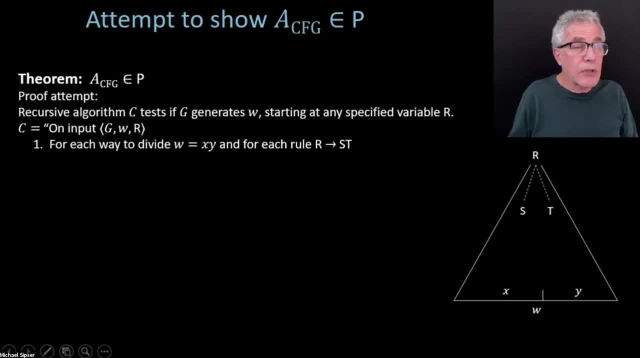 R goes to ST. So I'm going to, for each possible way of cutting w into x and xy and for each possible rule, R goes to ST. I'm going to see recursively: can I get from S to x and from T to y. 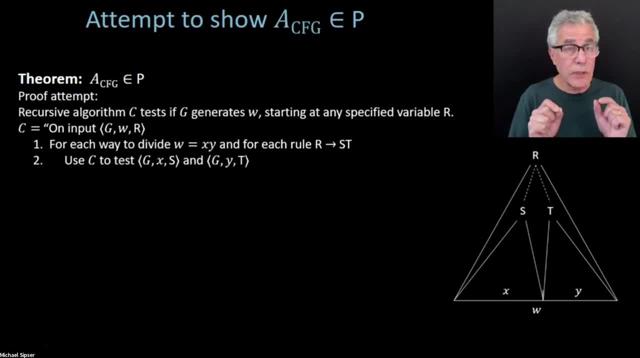 So I'm going to use my recursion now. Now that I have smaller strings instead of w, I can apply recursion and try to answer it that way, And this algorithm will work. So if I found a way to cut w into xy and I found a rule, 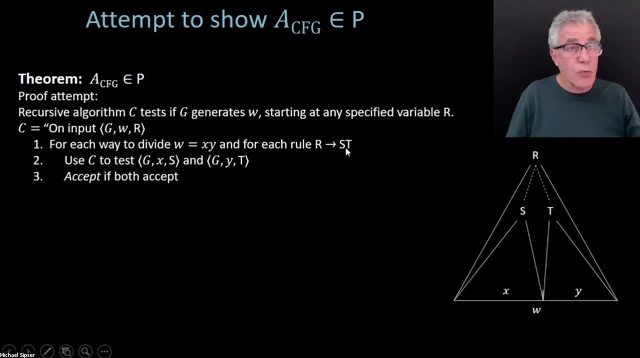 R goes to ST such that S generates x and T generates y, then I'm good. I know I can generate w from R, OK. And if there's no way of cutting w up to satisfy that, or, you know, if I can't find any way to divide w into xy and a rule, 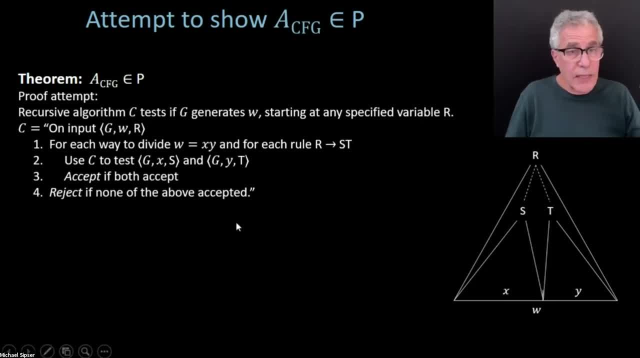 R goes to ST, which makes this work. if all possible ways fail, then you can't get from R to w. OK, And then you can decide the original ACFG problem now by starting from the start variable. instead of just any old R, You plug in the start variable for R. 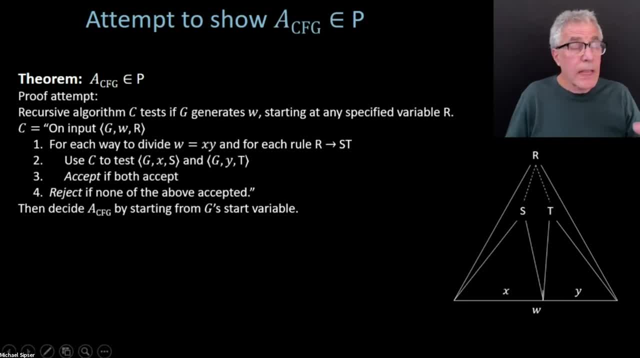 OK. so this algorithm works OK And it can be used to solve ACFG. But the question is: is it polynomial? And it's not, Because every time you're doing the recursion, you're essentially adding another factor of n. 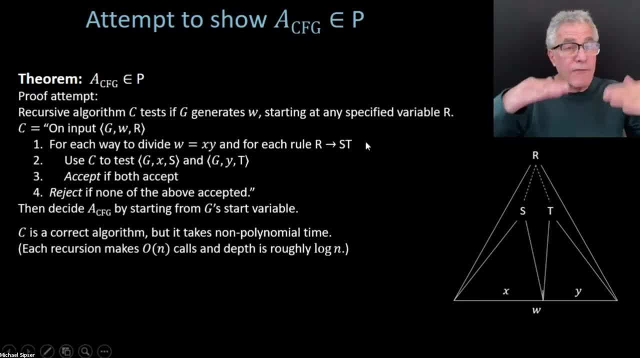 Because here, as we pointed out, this is a factor of n, But that's happening every time you're doing a recursive level And you can imagine- you know I'm just doing a very crude analysis here- depending upon how you divide w up. 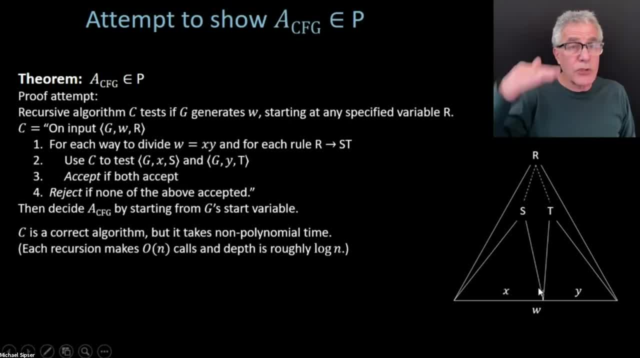 But roughly speaking, it's going to get divided in half each time. So there's going to be log n levels, And so that means you're going to be multiplying n by itself, log n times, or give you an n to the log n algorithm. 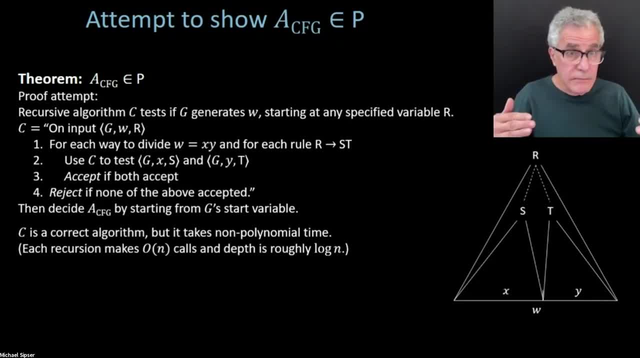 That's not polynomial, Because polynomial is n to the constant. for some fixed constant, n to the log, n is not going to be polynomial. So this is not a polynomial algorithm. So instead, you're going to. You're going to have to do something, just a little bit. 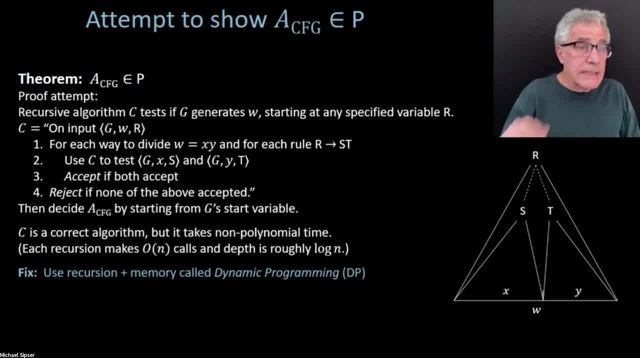 more clever. It's going to be the same basic idea, but just relying on one little observation, And the little observation is that when this non-polynomial implementation that I just described is actually pretty dumb Because it's doing a lot of recomputation of things, 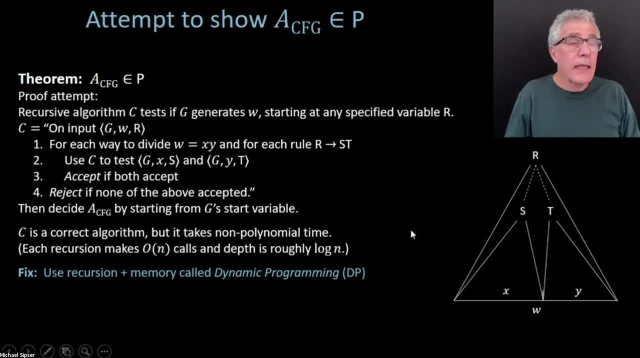 that it's already solved. Why is that? Because if you look at the number of possible different subproblems here, once I fix, once I give you g and I give you w, how many different subproblems g, s and t are there. 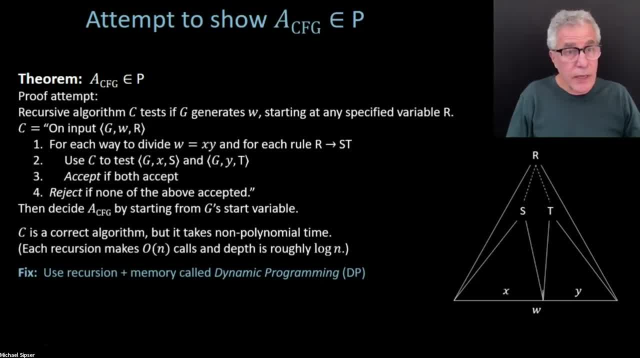 Well, the number of sub, the number of strings here, all of those strings are going to be substrings of w. There's only roughly n squared substrings of w. I'm always going to be generating in a subproblem here some substring of w from some starting variable. 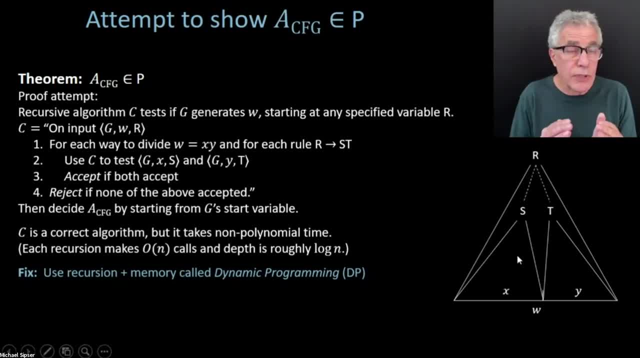 in the grammar. So, because there aren't that many different substrings and not that many different starting variables, the number, the total number of possible problems that this algorithm is going to be called on to solve, is going to be, in total, a polynomial number of different substrings. 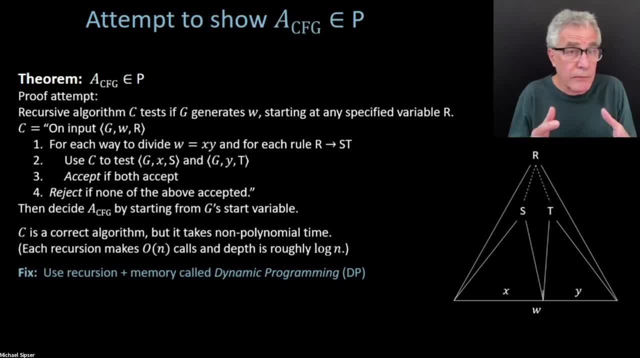 There aren't very many of them. There's only something like w and n squared. So if the algorithm is running for exponentially long time, it's solving the same subproblem over and over again. That's dumb. Why don't you just remember when you solve the subproblem? 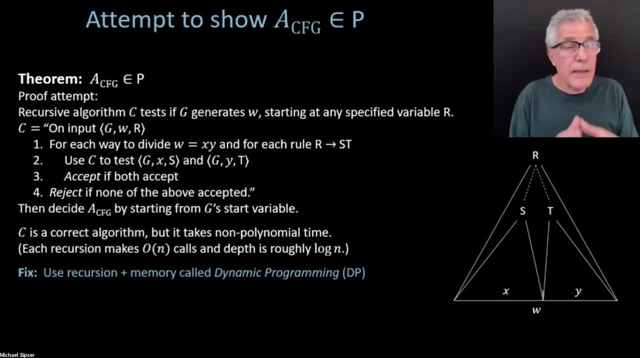 so you don't solve it again. Doing that enhanced recursion, where you remember the problems you've already solved, is called dynamic programming. I don't know why it has such a confusing name like that. Actually it's called by several different things. 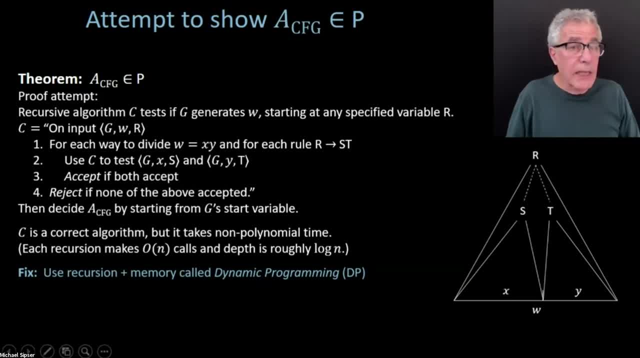 But anyway, that's known as dynamic programming. It's recursion plus the memory. And here is just repeating myself. There are not very many different substrings, So every time you're going to be in your recursion somewhere, you're going to be working with a substring. 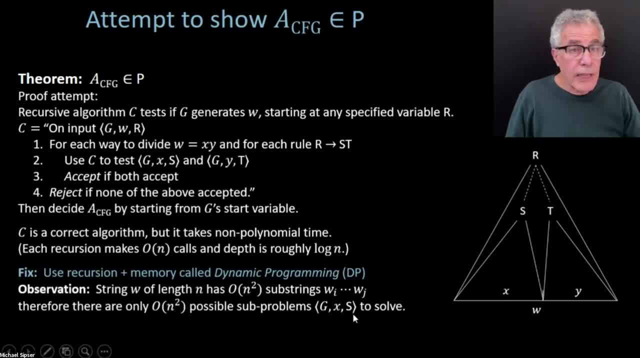 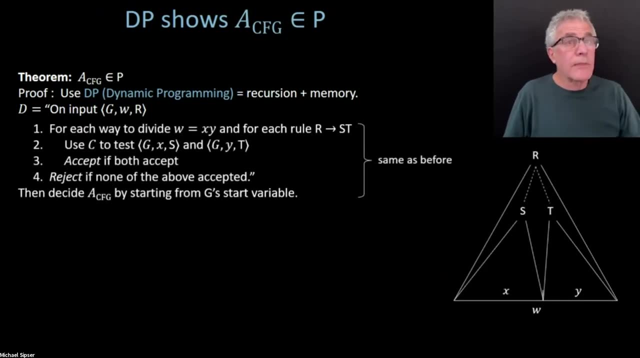 So there's not that many different subproblems that you can possibly solve And just remember when you solve the subproblem and not solve it again. So let me just show you that algorithm again here, with a little modification. So first of all let me give you this is the same algorithm. 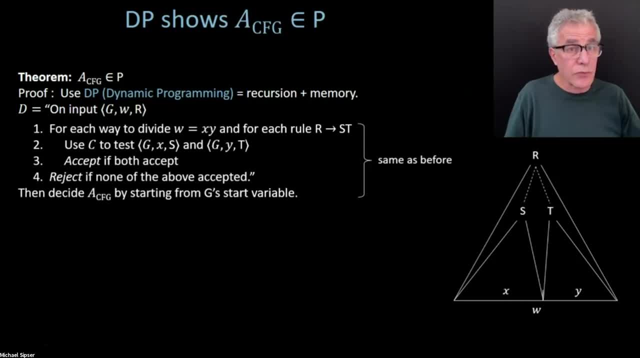 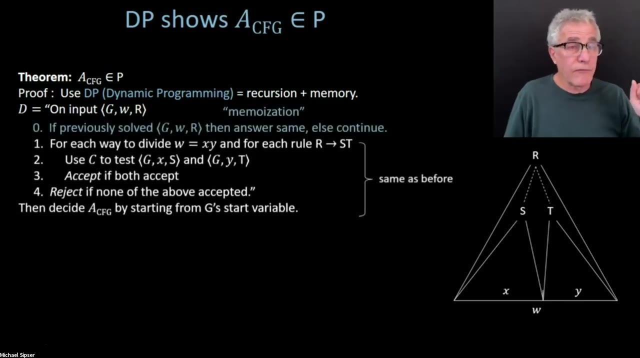 from the previous slide. I'm just repeating it here, without all the other stuff, so we can just look at it directly, Dividing it into x and y for each possible rule, And then recurse. Now I'm going to add a little step 0 beforehand which says: 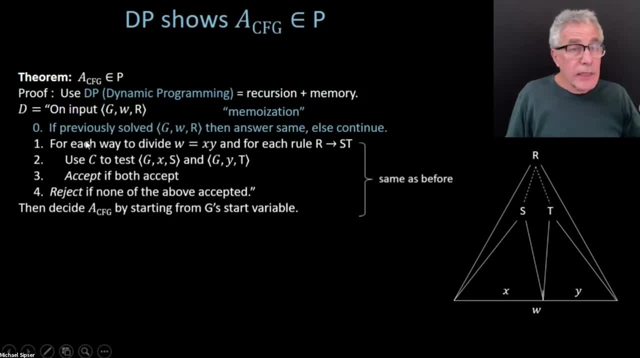 if I have g, w and r, let me just check first whether I've already solved that one before. So I have to keep track of the ones I've already solved. That's not too bad, because there's only n squared order, n squared possible different ones. 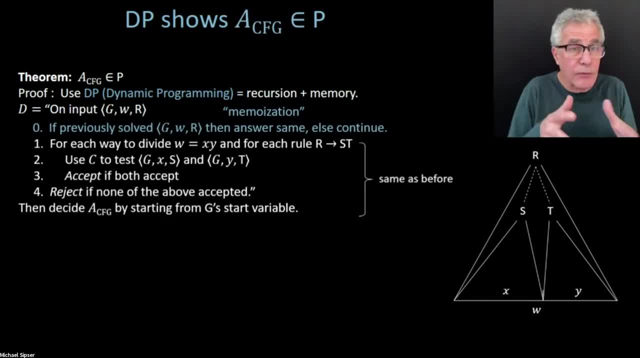 that I could be called on to solve. So I'm just going to have a little table where I'm going to remember those And then every time I get a new one, I get one to solve, I'll check. is it on that table? 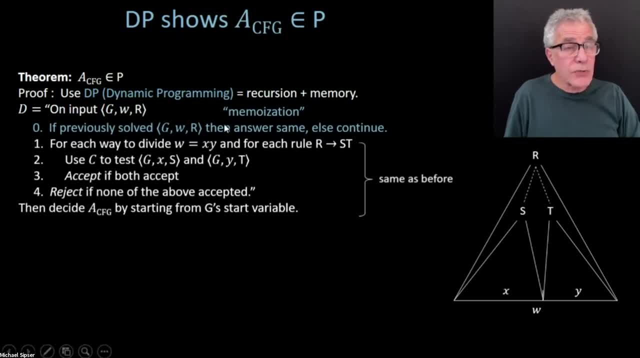 And what's the answer? So I won't have to rerun those. So now the total: I'm going to be basically pruning that tree so that it has only a polynomial number of leaves, And so the total size of that tree now is going to be polynomial. 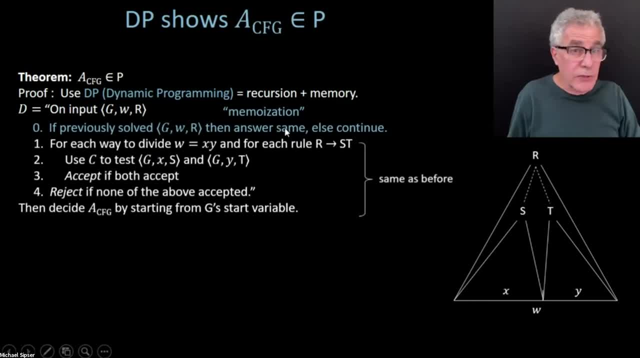 And so that's going to yield a polynomial running time. This, by the way- I only learned this myself. I'm sure you guys all know this who have taken this in the algorithms course- has a special name called memoization, not memorization. 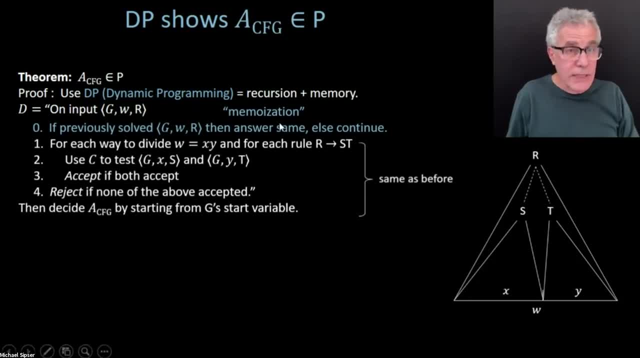 So that came from the same root, I think. But memoization, which is somehow remembering the results of a computation so you don't have to repeat it. So the total number of calls is going to be, at most, n squared to this algorithm, because you're never. 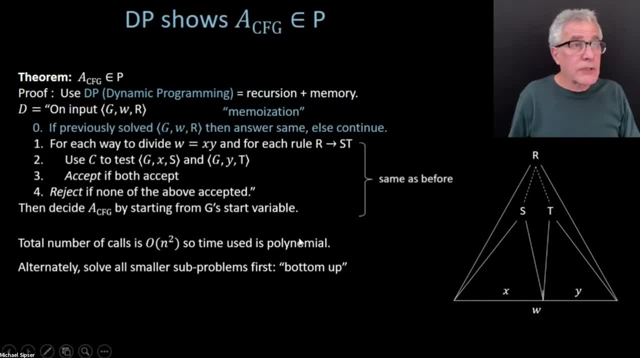 going to be redoing work that you've done already And when you actually have to go through it, the running time, so the total amount of time that you're going to need, is going to be polynomial altogether. So let's hear, I don't remember what my check-in is on this. 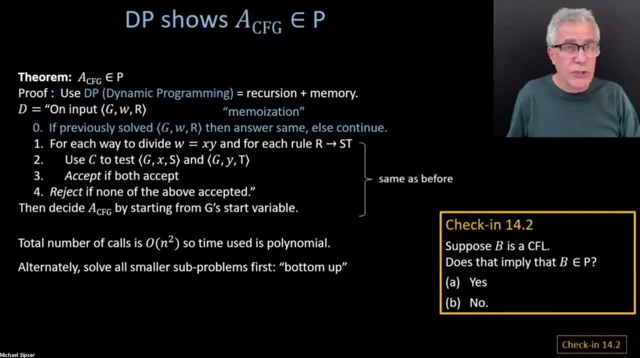 Oh yeah. So I mean this is somehow related And feel free to ask questions too while you're thinking about, you know this check-in. But the check-in says: here we've solved the ACFG problem in polynomial time. 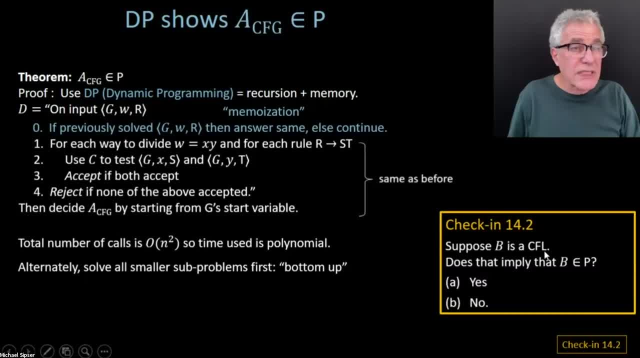 Does that tell us that every context-free language itself is also solvable in polynomial time? So just mull that over and please give me an answer to it. I hope you do better on this check-in than you did on the last one. 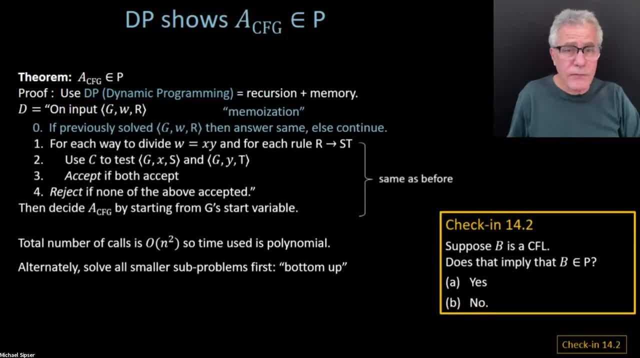 But anyway, why don't you go ahead and think about that And I can take some questions in the meantime? Somebody is asking here- actually I'm getting several questions on this- Why isn't it order n cubed or something greater than order n squared? because of the variables? 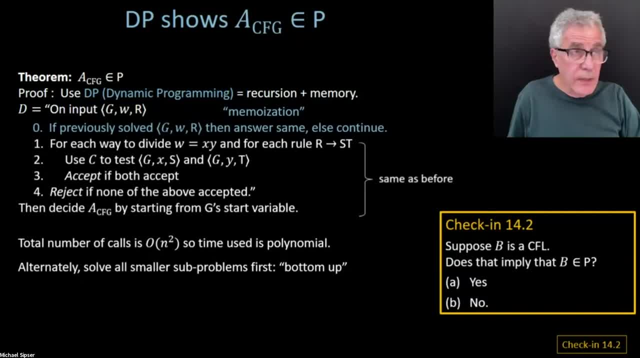 The variables are not. don't depend on n. You know when you're given. Well, actually that's not true. No, You are right, because the grammar is part of the input, So you might have as many as n different variables. 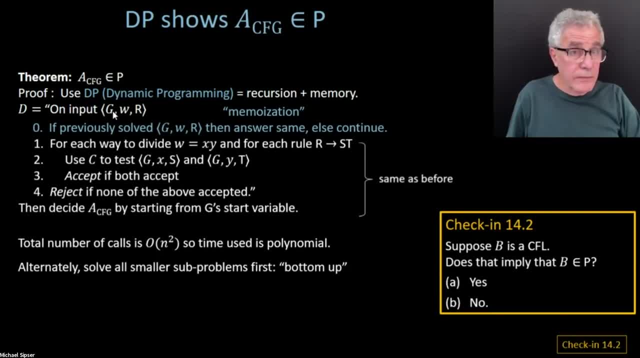 in the given grammar. So you are right, There is potentially, you know, the grammar might be half the size of the input and the input to the grammar w might be half the size of the input. So I didn't think about that, but you're correct. 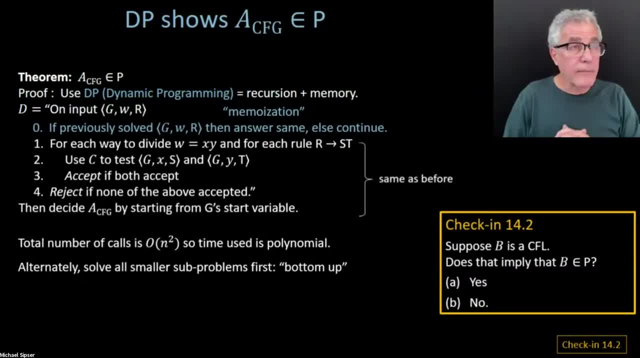 There are potentially different numbers of variables in different grammars, So you have to add an extra factor, which would be at most the size of the input, because that's as many variables as you could possibly have. So it really should be, I think. order n cubed. 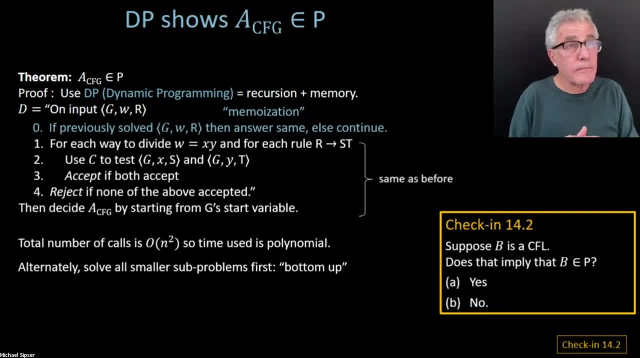 to take that into account as well, plus all of the work that needs to happen in terms of the number of variables that you have. So that's going to happen. in terms of dividing things up On a one-tape Turing machine, there's. 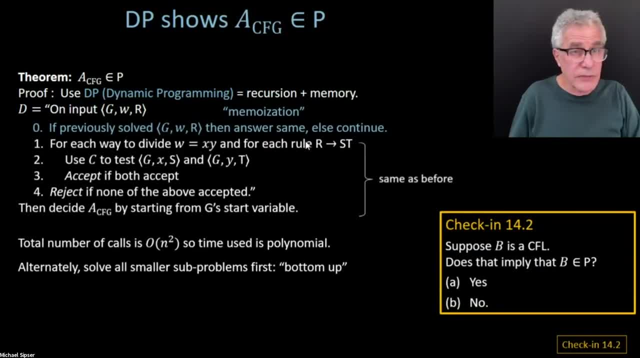 going to be some extra work just to carry out some of these individual steps, because with a single tape things are sometimes a little awkward. I think the total running time is going to end up being something like n to the fourth or n to the fifth on a one-tape Turing machine. 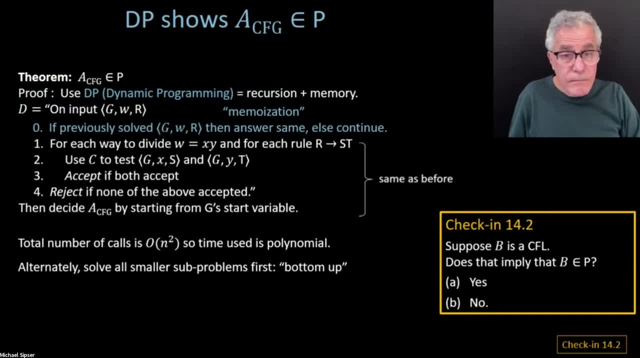 But that's a good point. So somebody is saying: how can we run n squared strings in finite time? I'm not saying why finite time. We have polynomial time. Every stage of this algorithm is allowed to run for polynomially many steps. 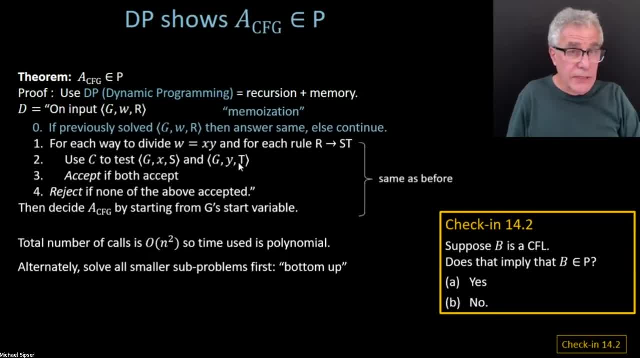 As long as it's clearly polynomial, we can just write that down as a single stage. Part two should say: oh, there's a typo here, So use d. Thank you, That is a typo, I'm afraid, if I change it on my original slide here. 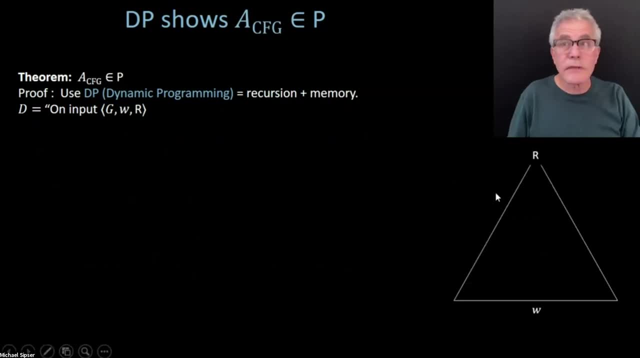 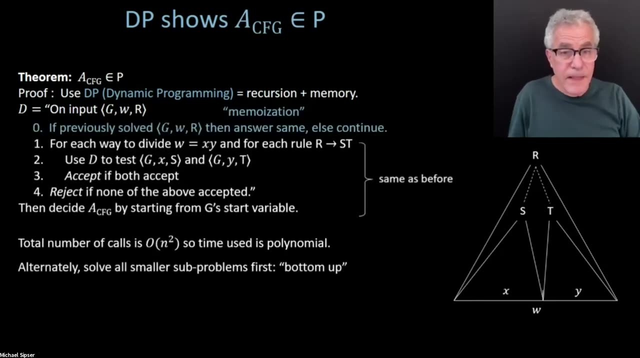 things will break in some horrible way. Let's just see. Did I completely wreck my slide? No, that's good. Yeah, thank you, Good point. Oops, OK, how's our check-in doing? OK, I think you're just about all done. 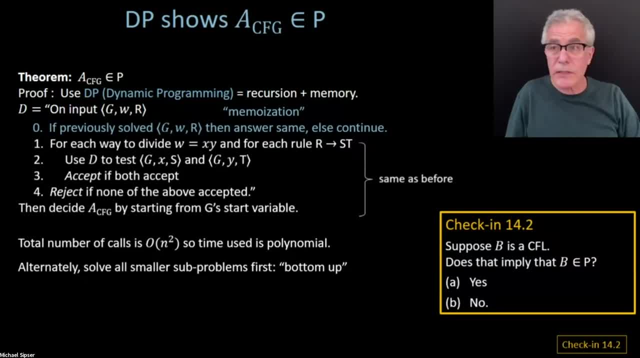 Oh, I still spent a lot of time on this End polling, As you may remember from the first half of the course. so the answer is A. indeed, Remember that we showed ACFG is decidable and therefore each context-free language itself is decidable. 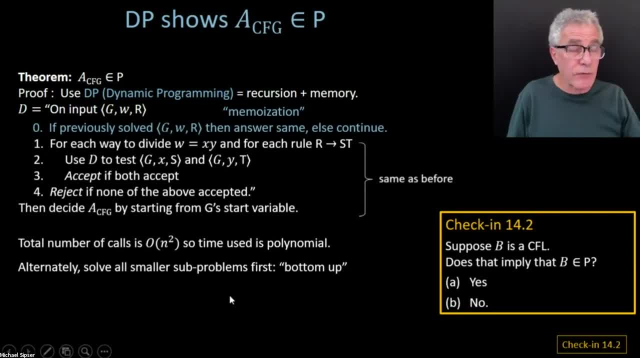 just because you can then plug in a specific grammar into the ACFG. The very same reasoning works here. So if you have a context-free language, it has a grammar. you can plug that grammar into the ACFG problem and then that's polynomial time. 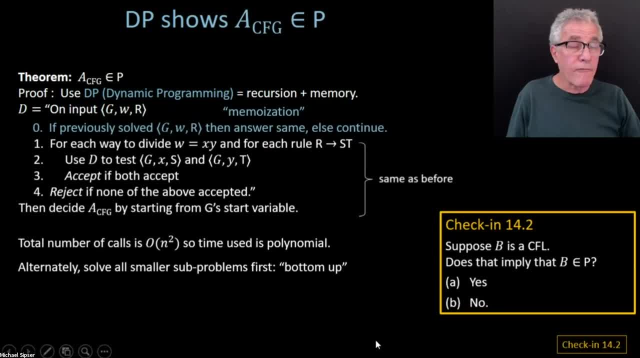 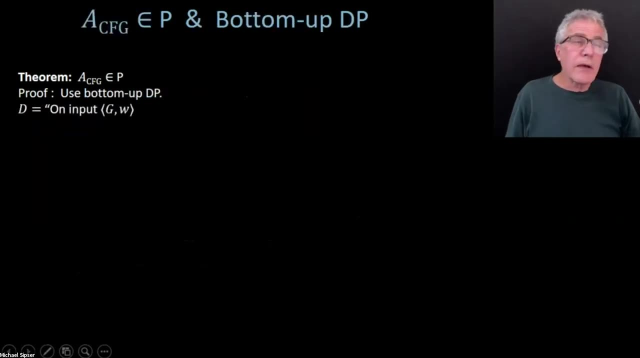 You're going to get a polynomial time algorithm for that language. So good to review that. It's the same thing from the same argument we used before. OK, Also, I don't want to spend a lot of time on this. There's another way of looking at dynamic programming. 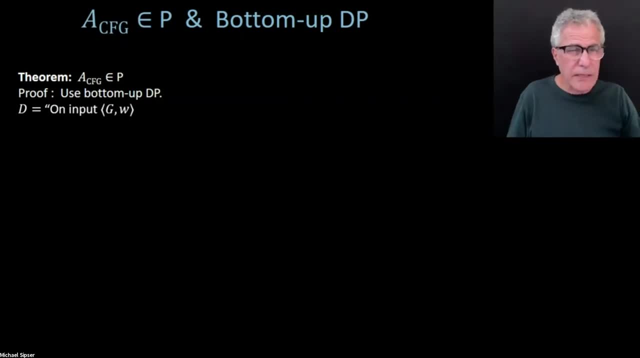 We'll talk about this again, maybe in a lecture, probably next lecture, just because I know you have a homework problem on it And if you've seen dynamic programming before, this is going to be easy. If you haven't seen it before, it's going to be, I think. 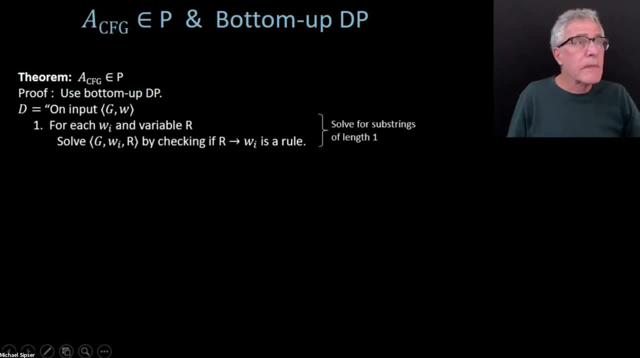 probably a little challenging. But another way of looking at dynamic programming is the so-called bottom-up version of dynamic programming, And what that would mean is you solve all of the subproblems first, before you solve all the smaller subproblems, before you solve the larger subproblems. 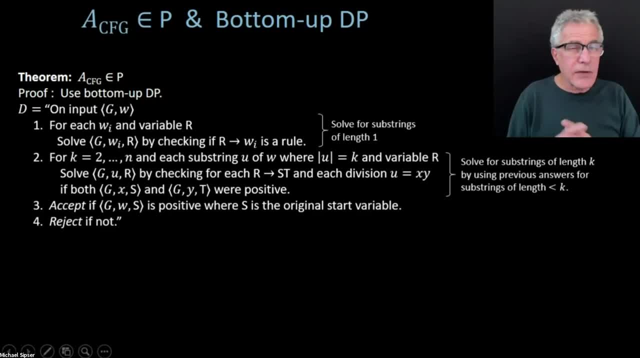 Let me just you know- it's here on the slide. I'm not sure I want to talk it through, But basically you solve the subproblems here where the strings are going to start with strings of length 1. And then from that you build up to subproblems. 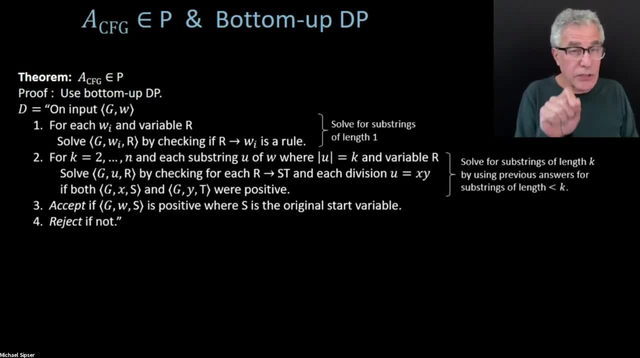 where the substrings are of length 2, and then 3, and so on, And each of those only relies on the smaller previously solved subproblems. So you can kind of in a systematic way solve all the larger and larger subproblems for larger 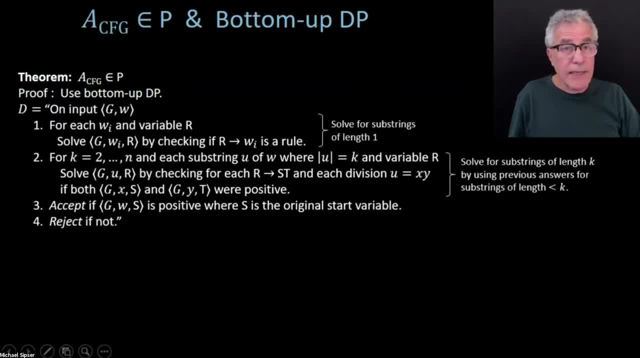 and larger substrings And that gives a kind of a different perspective on dynamic programming And it's kind of fantastic For different problems. sometimes it's better to think about either this sort of top-down recursion based process or the sort of the bottom-up process. 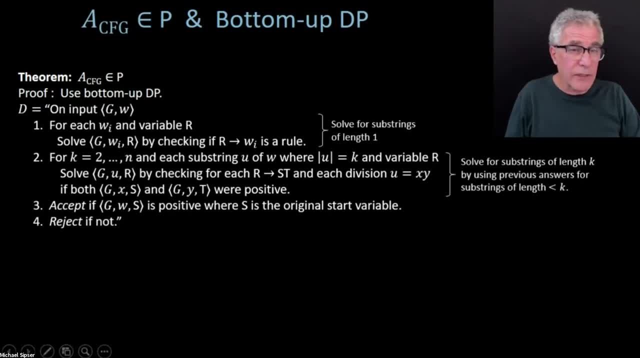 that I'm describing here. They're really completely equivalent, But you know, the version that's described for this particular algorithm, which appears in the textbook, is actually the bottom-up algorithm, So you shouldn't be confused if you see something there which looks somewhat different. 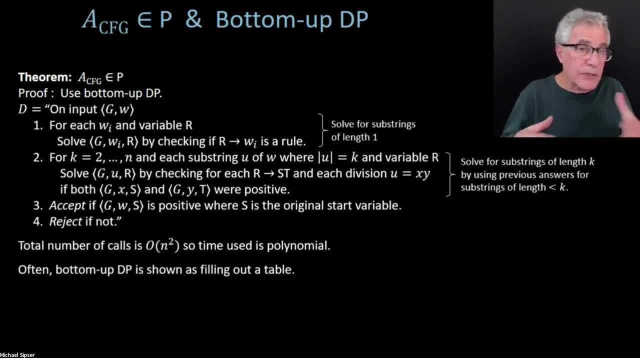 And that's often you see, you basically solve all possible subproblems, basically filling out a table. Let me not say anything more about that here, since we're running a little short on time, But there are really two perspectives on dynamic programming. 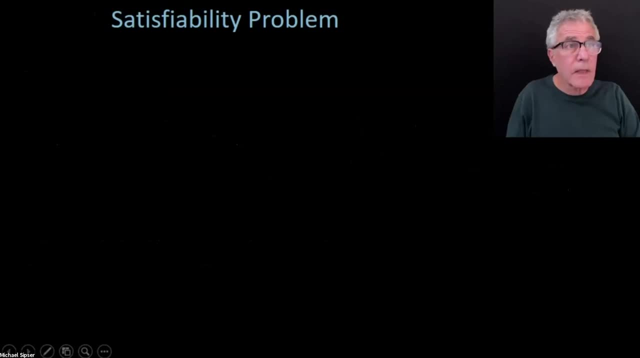 OK. so, moving on from there, let's shift gears, Leave context-free languages and dynamic programming behind and start moving toward understanding P and NP, And for that we will introduce a new problem called the satisfiability problem, And that's one we're going to spend a lot of time on. 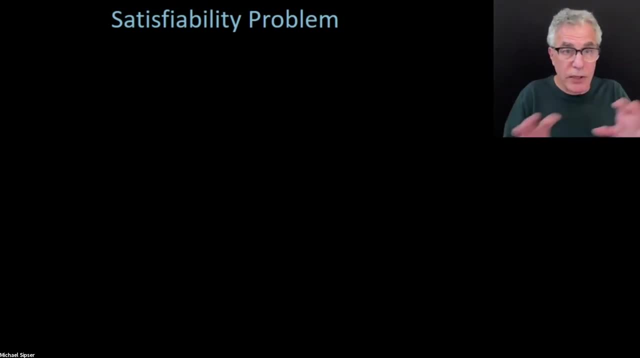 So important to, if you tuned out a little bit during the dynamic programming discussion time to get back on board. So the satisfiability problem is going to be a computational problem that we're going to be working on And it has to do with Boolean formula. 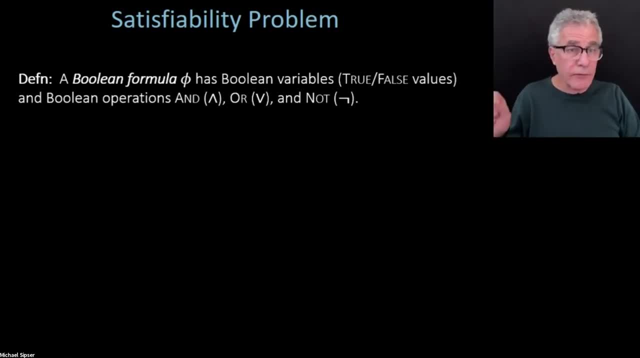 So these are expressions like arithmetical formula, like x plus y times z, But instead of using numerical ones, we're going to be using Boolean variables that take on Boolean values: true, false, or sometimes represented by 1 and 0.. 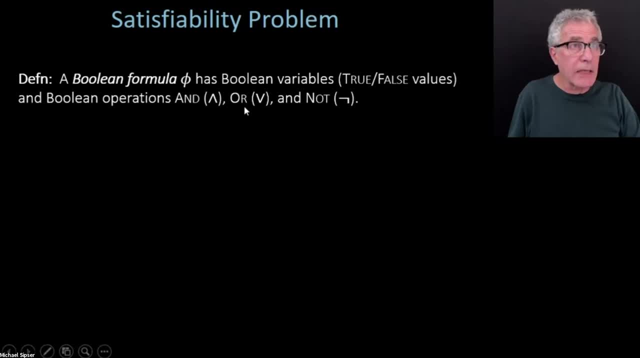 And the operators that we're going to be using are going to be the AND, OR and negation operations: AND OR and NOT OK. And we're going to say such a Boolean formula, we're going to call it satisfiable. 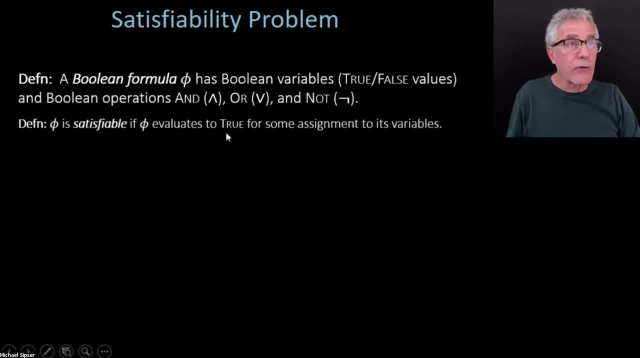 I'll give you an example in a second. If that formula evaluates to true, if you assign- make some assignment of values to its variables. So just like arithmetical formula will have some value if you plug in values for the variables. 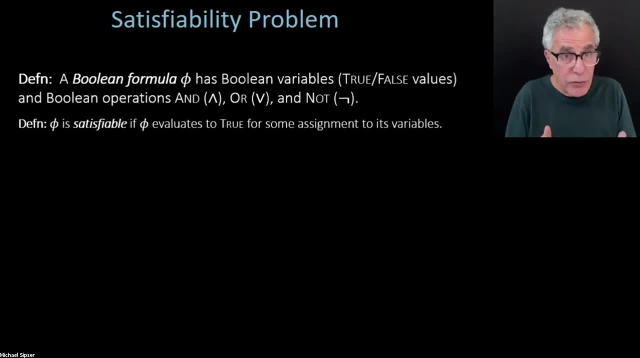 Boolean formula is going to have some value if you plug in Boolean values for its variables. And I want to know: is there some way to plug in values which makes the whole thing evaluate to true? The formula itself is going to evaluate to some either true or false. 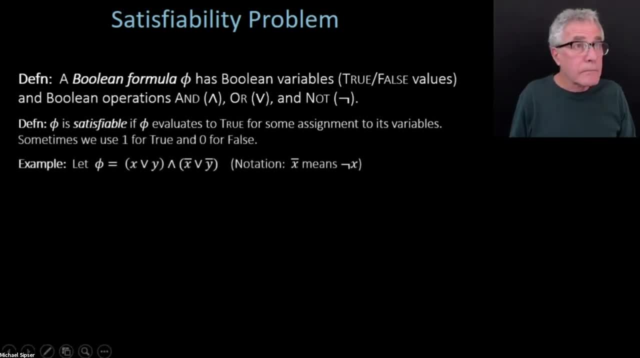 And I want it to evaluate to true. So here is our example. Let's take the formula phi, which is x or y and x complement or not, x or not y. So the notation x with a bar over it, x complement, is just x bar, not x. 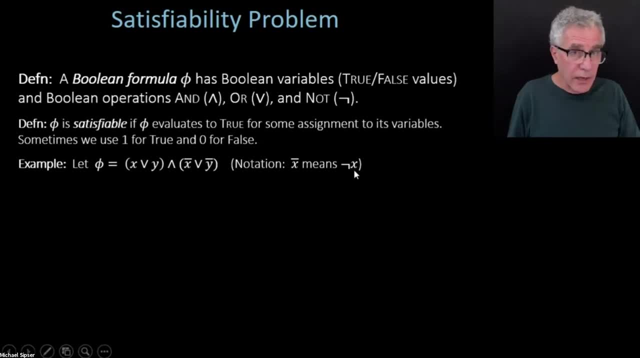 It's just the way. if you're familiar with the other notation for the not operation, which just inverts ones and zeros, we would write it. we're going to write it with a bar instead of the negation symbol. So I'm assuming that you've all seen Boolean algebra. 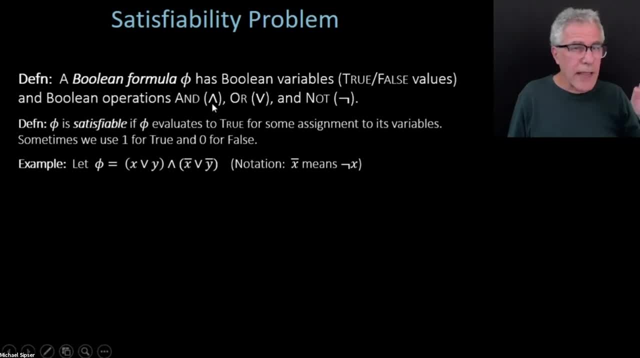 Boolean arithmetic before, where the AND operation is only true if both inputs are true. So these are going to be binary AND operations and binary OR operations. OR is going to be true if either input is true and not as true if its single input is false. 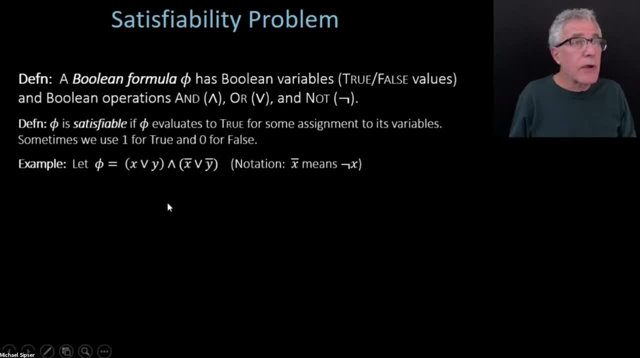 So it just flips the answer. OK. So here I want to know for this Boolean formula here: is it satisfiable? Is there some way to assign values to the variables to make this formula evaluate to true? So for example, let's just try things. 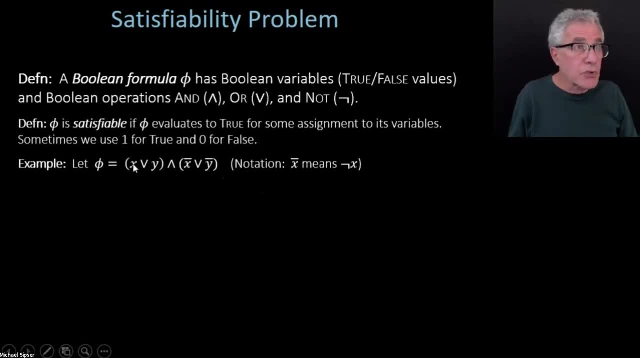 Let's make x and y both true. So x is true and y is true. So x or y? well, that's good, that's true, But now we have to do an AND, so we need both sides to be true. 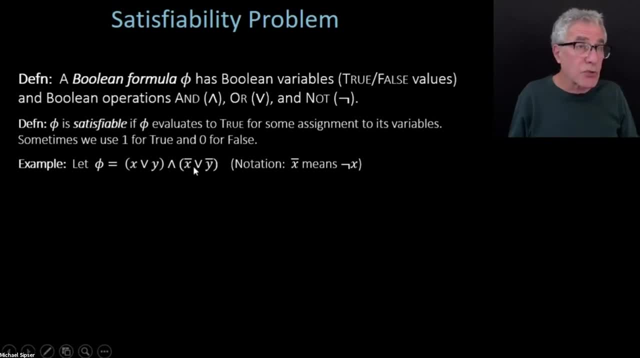 So now we have x complement. Well, we said x is true, so x complement is false, y complement is false, False or false is false. So now we have a true and false That's going to be false. We did not find a satisfying assignment. 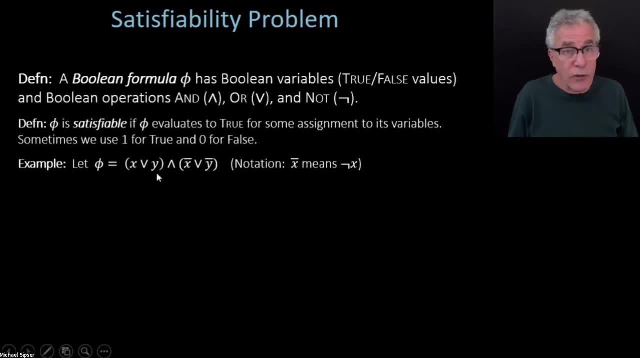 But maybe there's another one, And in fact there is. If you make x true and y false, then both of these parts will evaluate to true and then you'll have true and true. So we found a satisfying assignment to this formula. 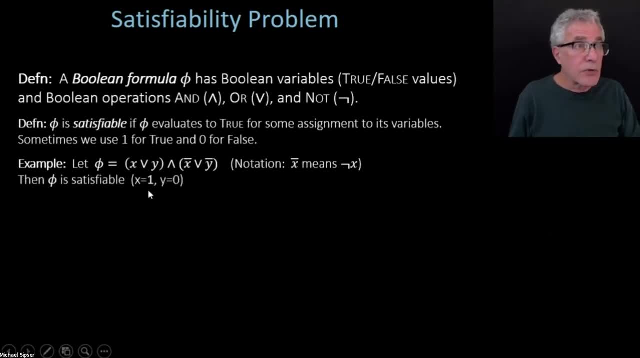 It is in fact satisfiable. So if you say x is 1 and y is 0, yes, this is satisfiable. Now the problem of testing for a Boolean formula, if it is satisfiable, is going to be the SAT language. 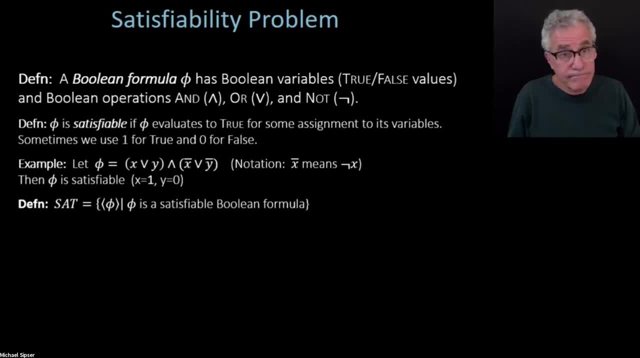 It's a collection of satisfiable Boolean formula And testing whether you're in SAT or not is going to be an important computational problem. And there was an amazing theorem which really got this whole subject going. It was discovered independently by Steve Cook in North America. 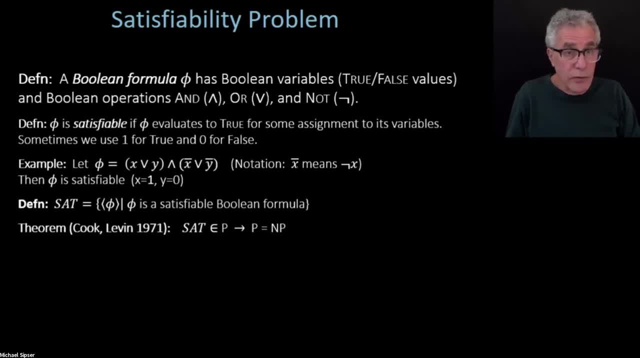 and Leonard Levin in the former Soviet Union almost exactly at the same time, which made a connection between this one problem and all of the problems in NP. So by solving this one satisfiability problem in polynomial time, it allows you to solve all of the problems. 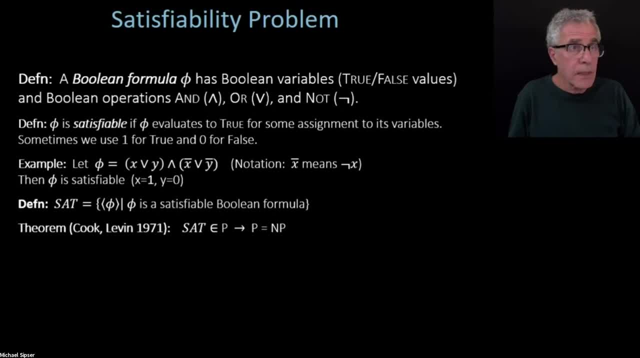 in NP in polynomial time. So if you could solve this problem SAT in NP, then Hamiltonian path is also solvable in P. It's kind of you know, you step back and think about that. it's kind of amazing. 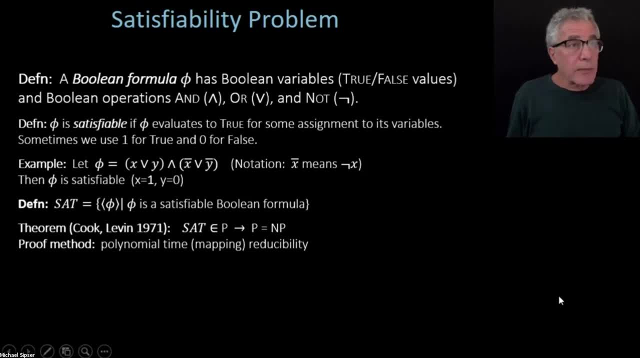 And the method that we're going to introduce is called polynomial time reducibility, And let's do a quick check-in on this. This should be an easy one. Why don't you just think about? is SAT, the SAT problem that we just described there? 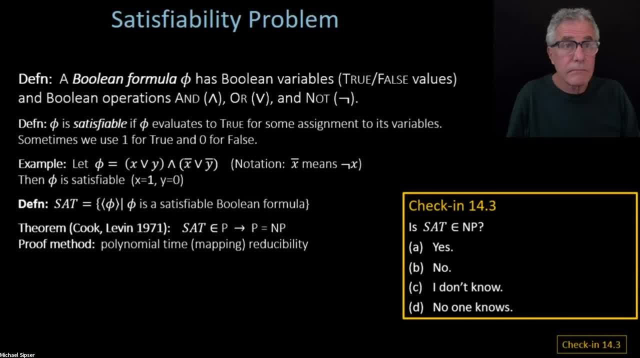 is that in NP, Three seconds, You all there. OK, Ending polling. Yeah, So hopefully you're getting the intuition for NP that these are the problems. To be in NP means that when you're a member of the language, there's a short proof or a short certificate of membership. 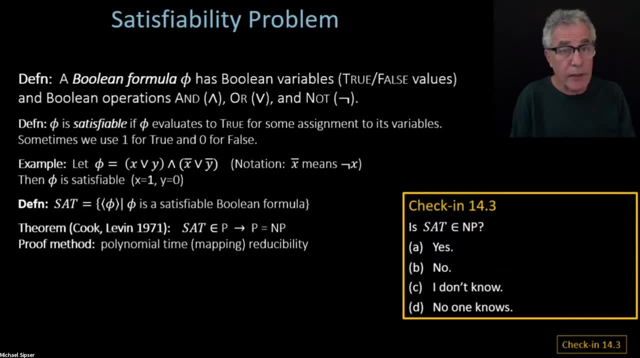 In this case, the short certificate that the formula is satisfiable is the assignment which makes it true, also called the satisfying assignment. So, yes, this is an NP language, a language that's in NP, So there are a lot of things that we don't know in this subject. 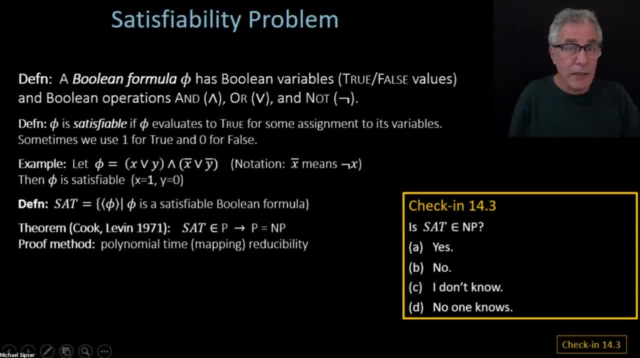 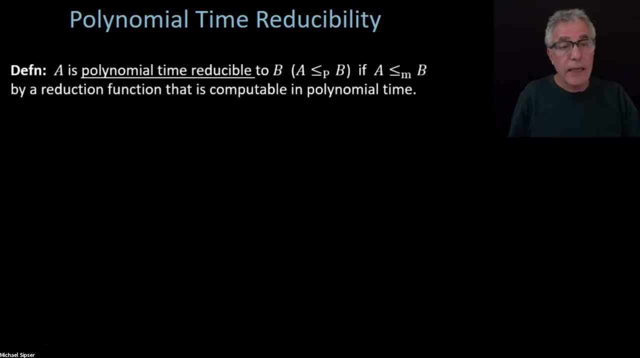 but this isn't one of them. We do know that SAT is in NP, So let's talk about our method for showing this remarkable fact that if you can solve SAT in polynomial time, then all of NP is solvable in polynomial time, And it uses this notion of polynomial time reducibility. 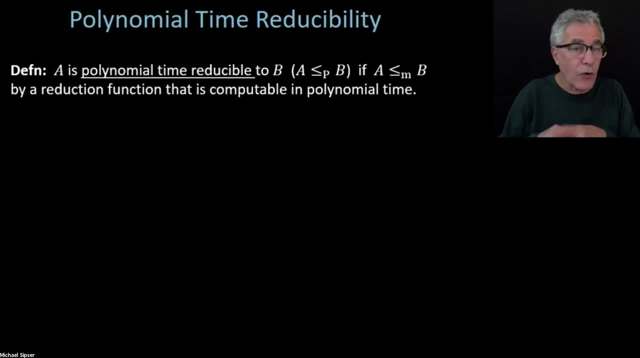 which is just like mapping reducibility that I hope you've all grown to know and love in the first half of the course. But now the reduction has to operate in polynomial time. So it's the same picture that we had before, mapping A to B, transforming A questions to B questions. 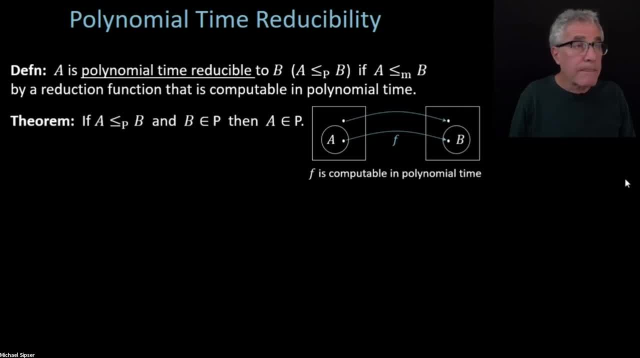 but now the transformation has to operate quickly And we get that if A is polynomial time reducible to B and B is polynomial time, then A is also polynomial time. Same pattern as before: If A is reducible to B and B is easy, then A is easy. 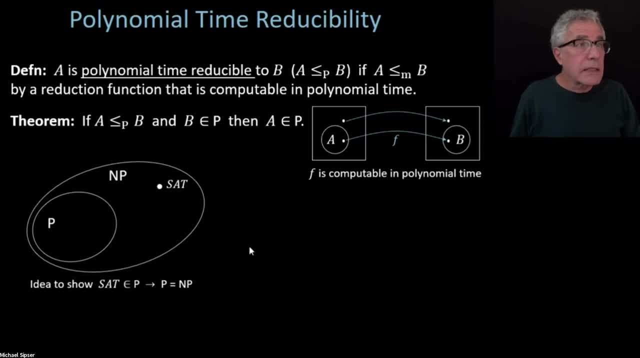 And here is kind of the essence of the idea, or at least the outline in a sense, the idea of this Cook and Levin theorem, that if satisfiability is in P then everything in NP can be done in P. which is because we will show that all problems in NP 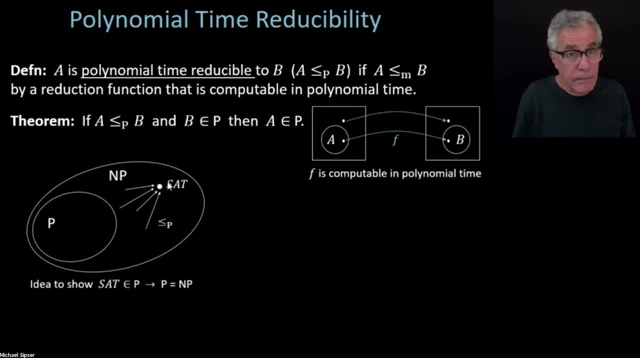 are polynomial time reducible to SAT. That's the amazing fact. So, therefore, if you can bring SAT down into P by using this reduction, it brings everything else along with it, because everything is reducible to SAT. So we just have to show how to do that. 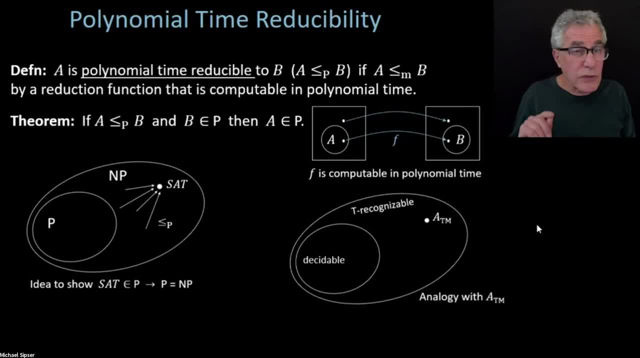 And there is an analogy that we had in the first half of the course in one of our homework problems, if you may remember, We showed that ATM has the very special property that all Turing recognizable languages are mapping reducible to it. I think that was problem 2 on 2A. 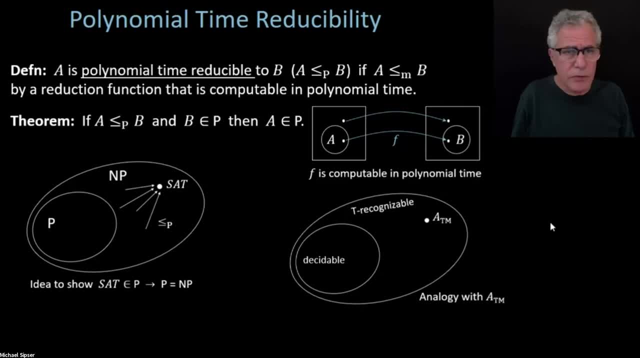 either in this problem set 3 or problem set 2. I think problem set 3. That every Turing recognizable language is polynomial time reducible to ATM, And so very similar picture And there's a lot of analogies here that you can draw. 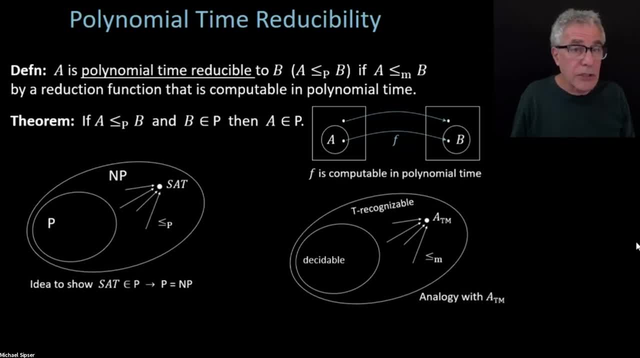 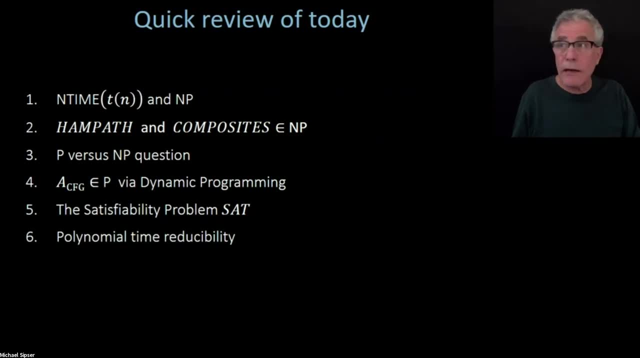 between the computability section and the complexity section. Anyway, with that I know we're just about out of time, so let's do a quick review of what we've done here And I will stick around for questions for a while. Is there a? 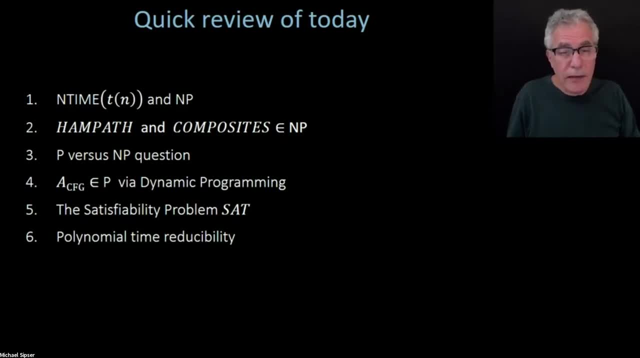 OK, that's a good question. Is there kind of a you know sort of a regular reduction analogy version to mapping reducibility? You know, we had the general reduction for the computability section and we had the mapping reduction for the computability section. 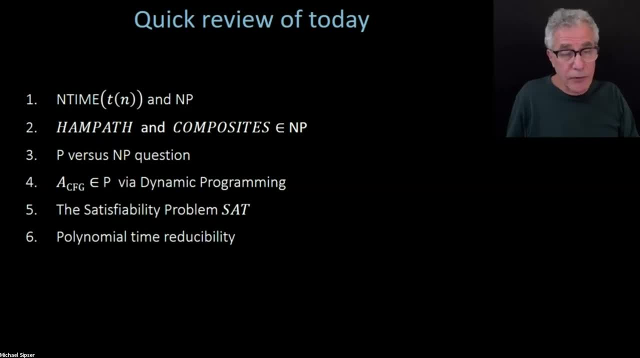 Here we're only going to be focusing now on the mapping reduction. So polynomial time reduction is, by assumption, going to be a mapping reduction. Yes, there is a general polynomial time reduction notion as well, If you you know, this is not required. 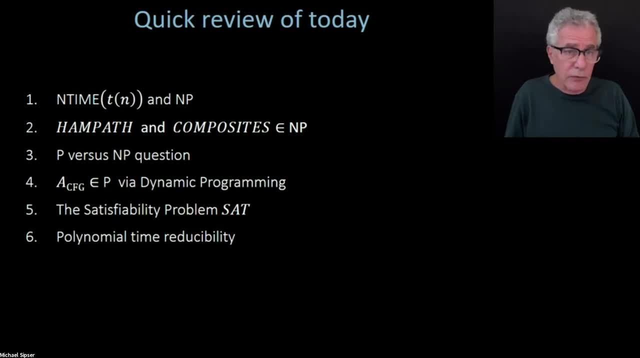 but if you are curious about the general reduction and how to precisely formulate that, it actually appears in chapter six under Turing reducibility. That's the general notion of reducibility spelled out in a formal way And there's polynomial time Turing reducibility as well. 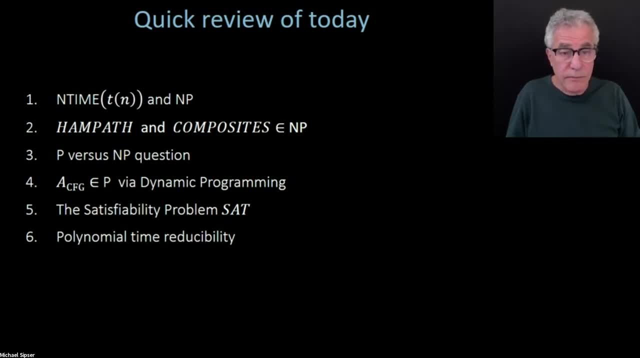 We're not going to talk about it in this course. Other questions: Does NP correspond exactly to verification in polynomial time? Well, we have to. for me to answer that as a precise question, we have to have a precise definition of verification. 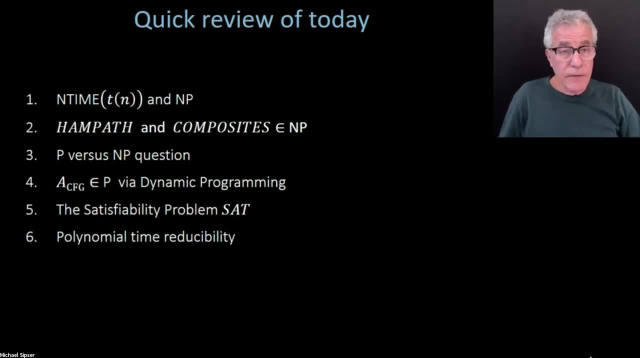 But with the right definition, the answer is yes. So you can define a verifier as a polynomial time algorithm that gives a certificate, that takes a certificate and an input to the language and will, you know, accept if that certificate is a valid certificate. 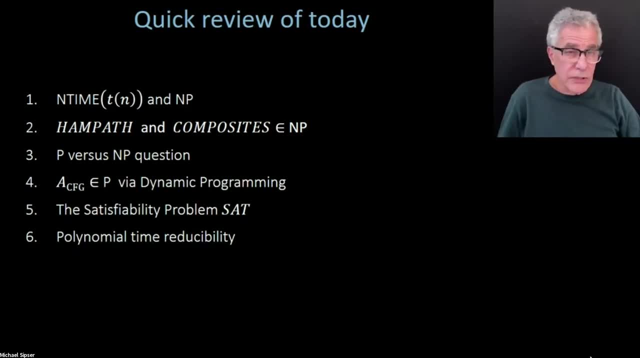 for that input. This is actually discussed in chapter I think nine of the text, But you now I'm forgetting already what's where in the book. But yeah, you can think of it. you can think of NP in terms of verification. 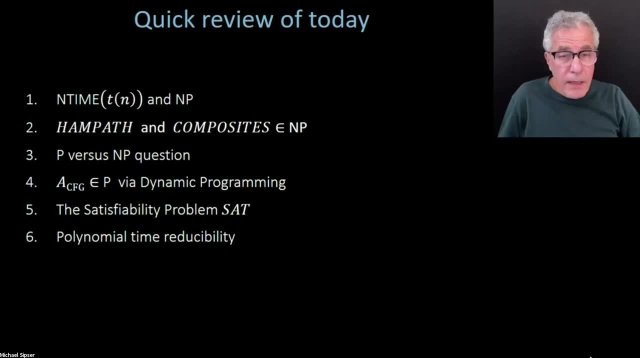 as a definition? Is proving P equal NP the same as proving that a polynomial? you know, actually I can even make the. if you want, you can post public comments too, as well. I should have done that in other cases. Is proving P equal NP the same as proving? 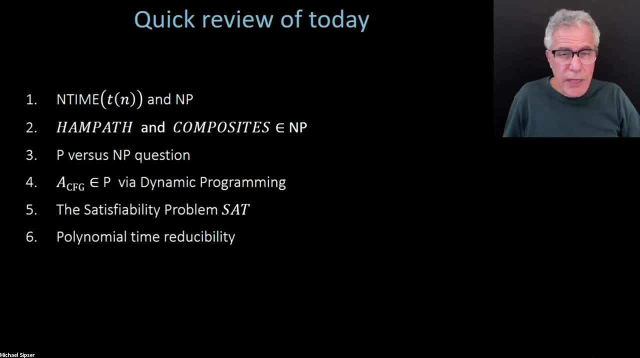 that a polynomial time non-deterministic. Turing machine N has a polynomial time deterministic. Yeah, So it doesn't mean that. suppose we prove that P equals NP, which is the minority view- I would say quite the small minority view- that 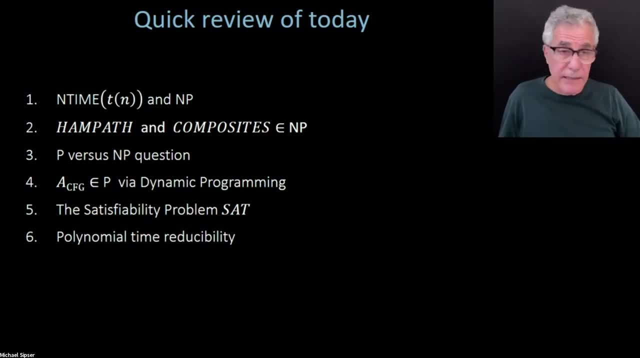 there are some people who believe that that is entirely possible and might even be the case, But that's a very small small group. But yeah, if you prove P equal NP, that's the same as saying that every non-deterministic polynomial time Turing machine.